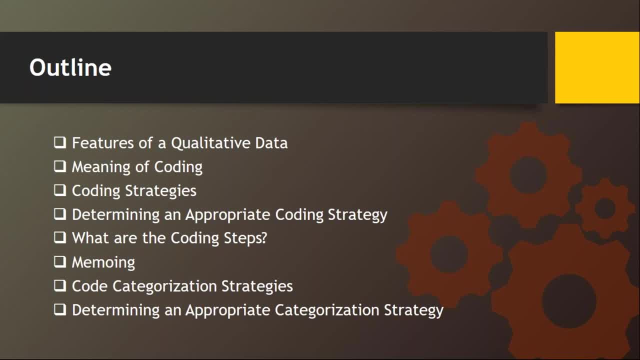 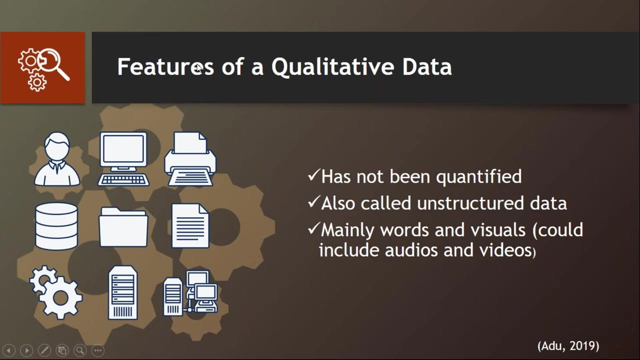 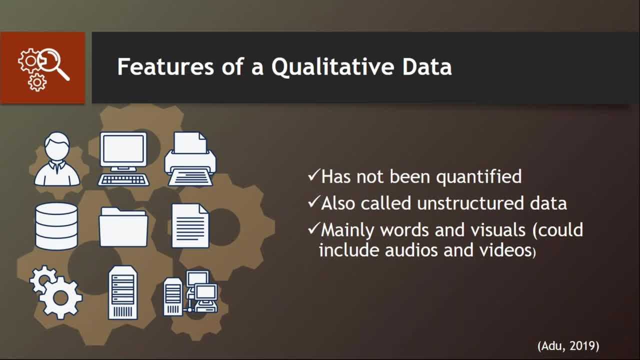 So to be more, to simplify the process, any data that is quantified is a qualitative data right, And sometimes people call it unstructured data because it doesn't follow specific formats. you know mostly words, sometimes visuals, or it can be audio and also video, So all these kind of information will help you to determine what 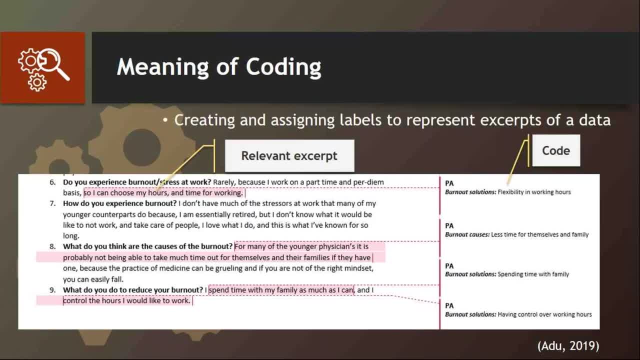 qualitative. qualitative data is all about Right. And so what is coding? Think about coding as summarizing right. You spoke to a lot of participants and they gave you many information that you wish you want to share it into your audience. But audience they don't have time to listen to everything that a participant tells you, So 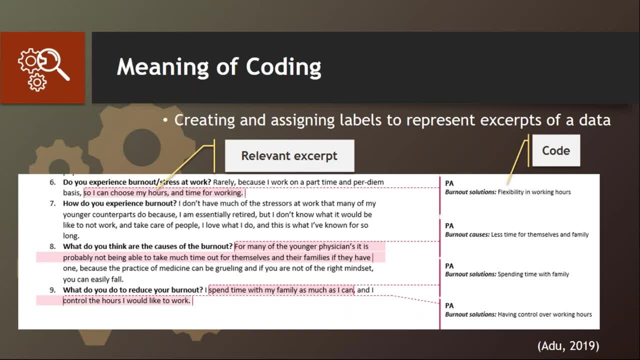 So what are you going to do? You have to summarize the information and give it to them, But you cannot just do ordinary summary, because you want them to trust the information that you got from them. And then what are you going to do? You have to do coding. So coding is all about assigning phrases to relevant information in the data, And those phrases will help you to address your research question. At the same time, the phrases are representing the 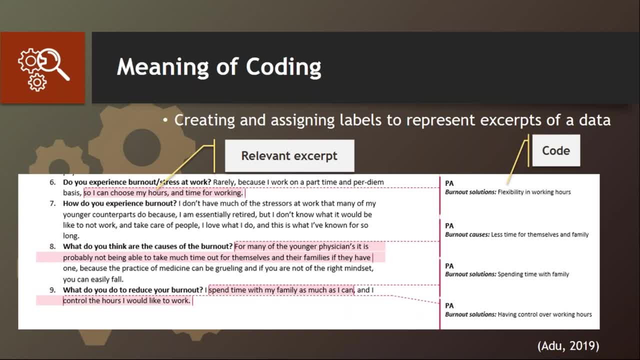 significant information in the data. So that's all about coding And it's all about data reduction. you are reducing the data, but you are not losing the meaning of the behind the data that participant gave to you. So you always have to be. it should be a systematic process, right Step by step process, so that your audience or your readers will believe what you found in your data. So they are. 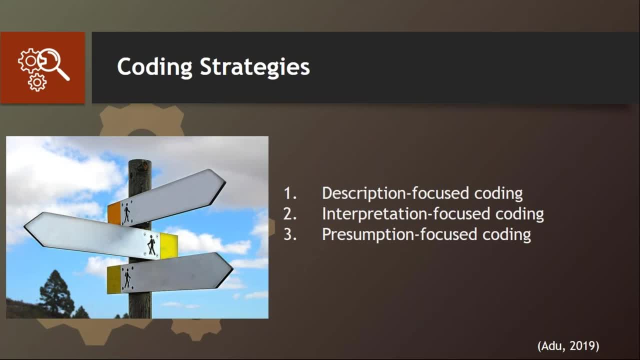 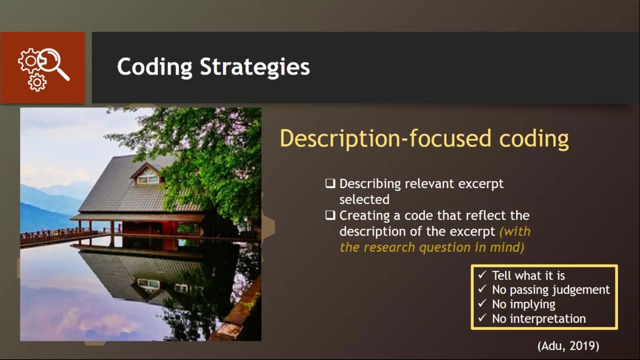 many strategies that you could use, But for my book I identify three main strategies that you can use to code your data. So we have description focused coding, interpretation focused coding and presumption focused coding. As the name implies, description focused coding is all about describing relevant information in the data right And after describing you. 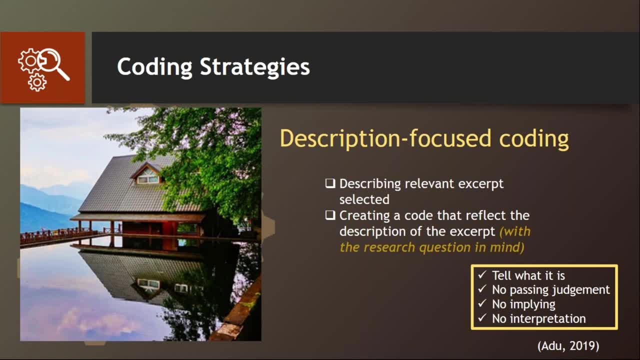 develop a phrase called a code to represent the description. And then so what you're doing? you are just telling what you see, or telling what participant is telling you. right, You are not making any judgment, you are not making any interpretation or not implying anything. You are just a vessel that participant information will be passing through you And then you give that information to your audience. No interpretation, you are just. 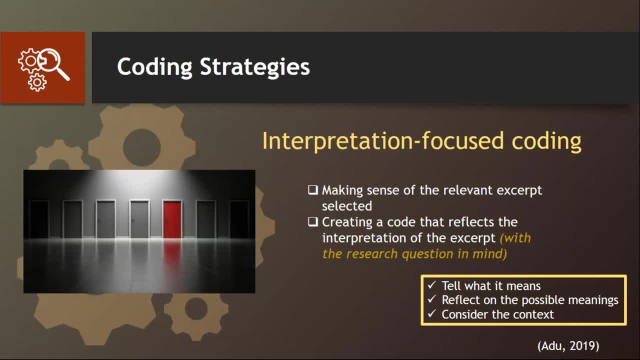 describing what they told you. For interpretation, focused coding, you are making sense of the relevant information. So, after you have identified significant information in the data, based on the research question, you ask yourself: what does this information mean? Right, And then, based on your, on your understanding of the meaning of the information, you create a phrase to represent that understanding, and a phrase should be able to address: 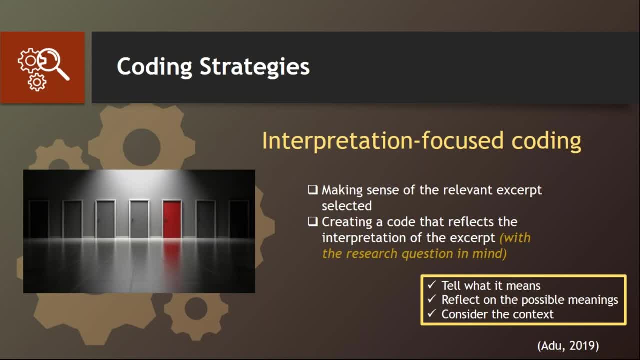 your research question that you have. So you always have to have your research question in mind as you are making sense of the data. So you are telling what it means, You reflect on the possible meanings, considering the context. who gave you that information? What is the situation? 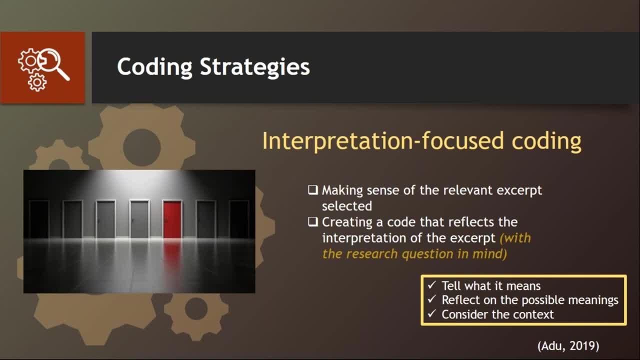 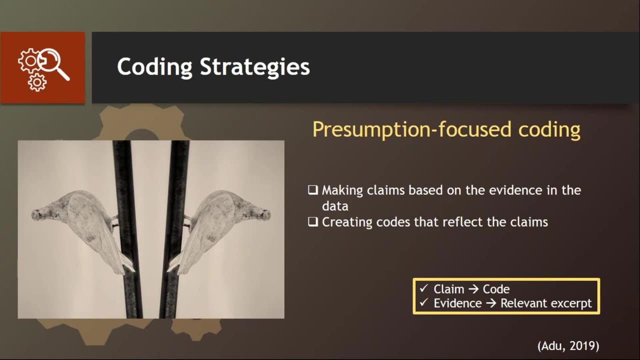 they find themselves in? Can their background information help you to understand what they are saying? So that's how it's all about the interpretation focus coding, And in my book I give you a lot of examples of how it will look like. The last one is presumption focus coding. 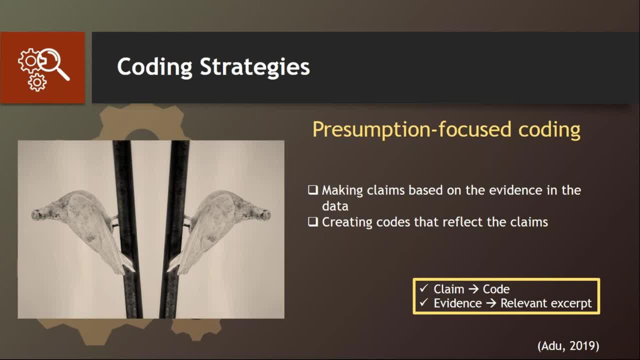 You are making presumption, you are making conclusions, So you see participant data as evidence and then, based on those evidence that you find in the data, you make conclusions, you make claims. So the claims will be phrases that will be used to represent the evidence that you see in the data. 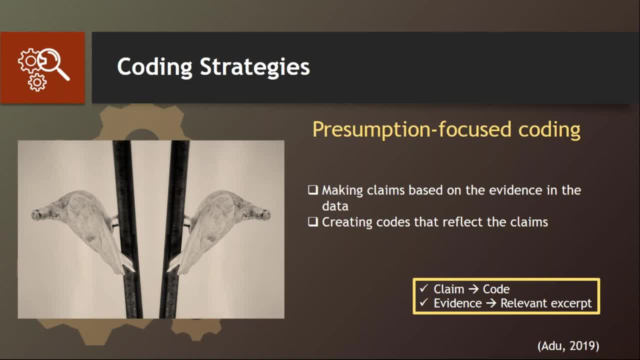 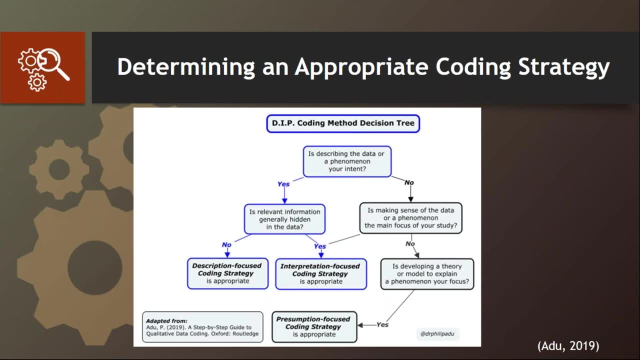 right. so that's also about the third strategy that you can use. So how do you decide the specific strategy that you have to use? So I have this diagram that will help you and to do that. But before we go to this diagram, let me give you an example. I don't know. 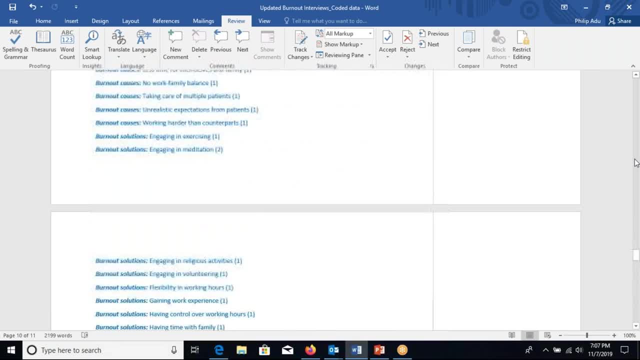 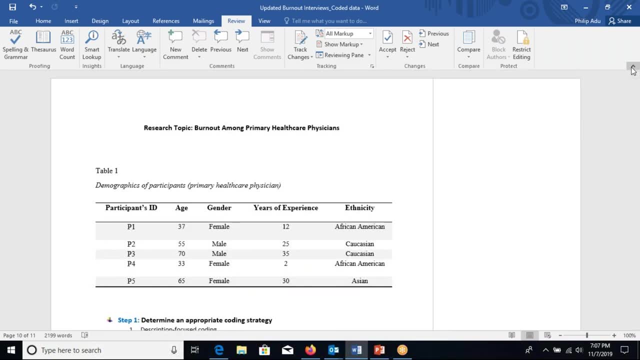 whether you have a copy of this document. um, i remember i sent it to dr morris, so okay. so let's um look through this and see whether i would be able to understand how to use their strategies. right, so let's assume that you have collected data from um five participants who are doctors. 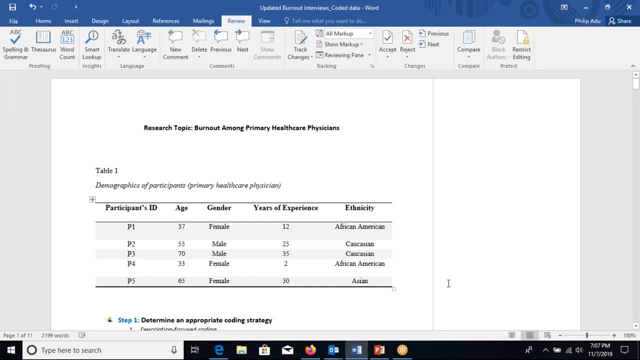 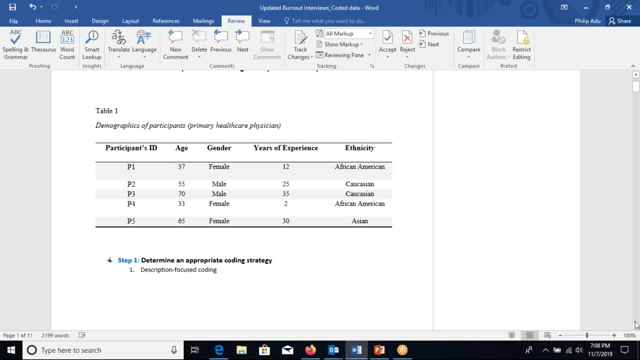 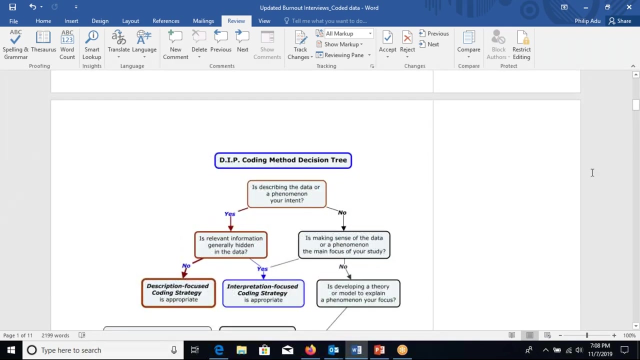 um, and these are their demographic information. so you have their age, their gender, their work, um year of experience and also the ethnicity right and then. so the first step that you have to do when you have your data is to decide what coding strategy should i use, and um, you always have to. 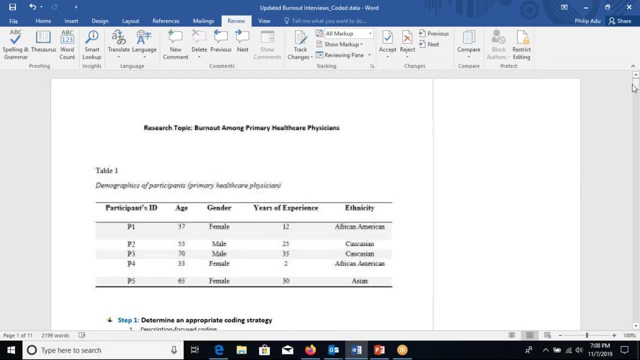 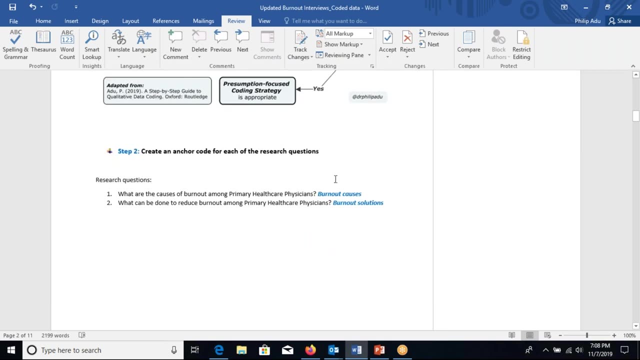 think about: okay, what am i looking for in the data? right? so your, the purpose of your study is to find out, uh, more information about burnout among um primary health care physicians, right? and then you look at your research questions, right? so um, looking at this research question. they are very straightforward. 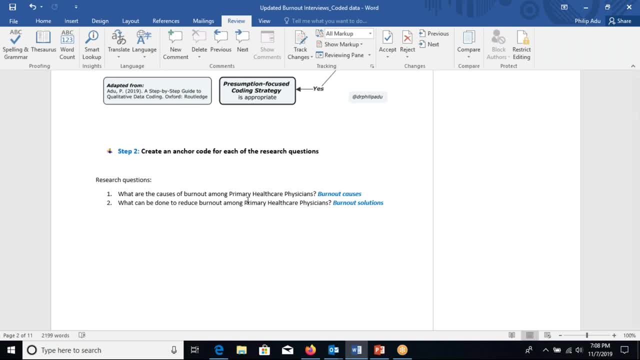 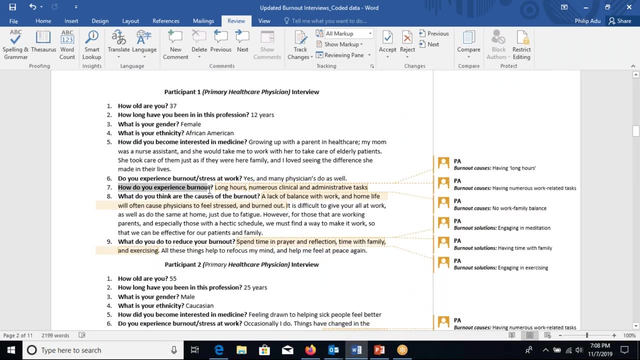 what are the causes of burnout among this population right and what should be done to reduce those burnouts. so it's so much direct information that you can get it from your data, especially if you ask during the intervention. you ask them directly about the experience about burnout and they provided that information to you. 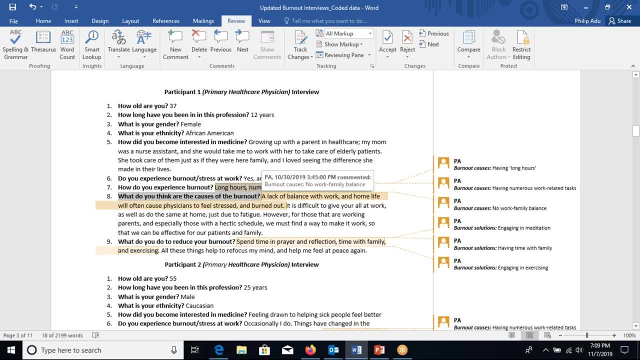 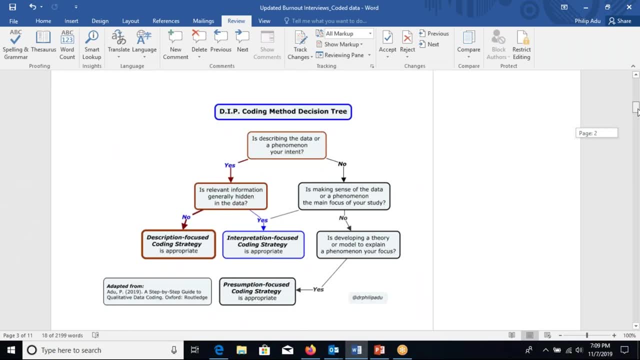 so the information is so direct, you can just go through the data and identify those significant information. because of that descriptive, description focus coding will be the best, because your data um, um. the purpose of the study is to describe what is going on in terms of the burnout, the causes and the solutions. right. 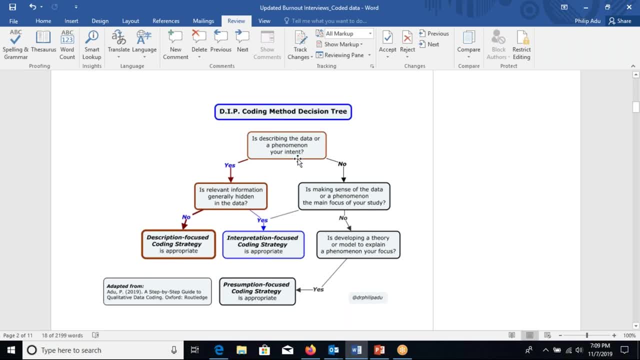 and you ask them directly. so you got the information directly from them. you don't have to imply or interpret the information, they just gave it to you. you just have to summarize and present it to your audience and, when you look at your data, to the information that you are looking for. 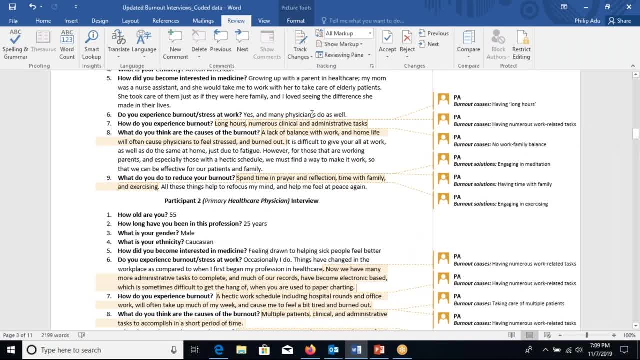 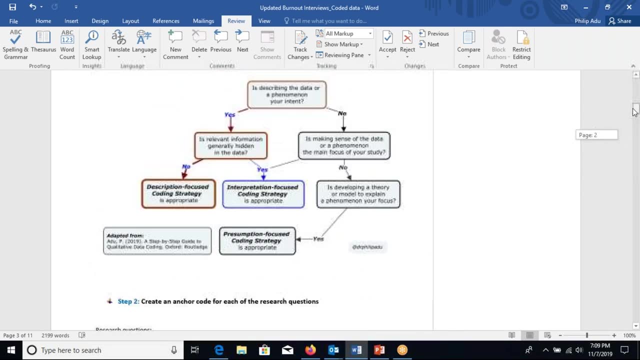 is not hidden, it's in plain sight because you ask them a direct question about the experience of burnout. they provided you that information so you don't have to make sense of it before you can do the coding. so that's why descriptive- uh description- focus coding will be the best right. 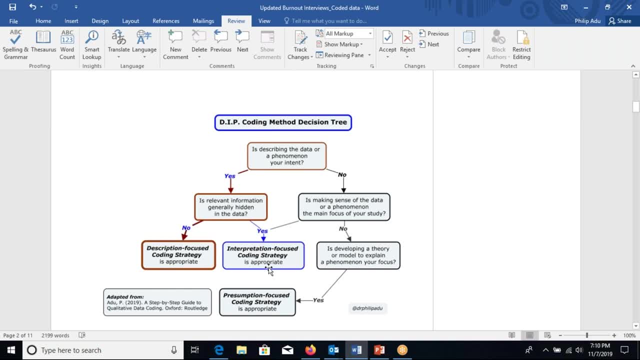 it doesn't mean that if you choose the interpretation- uh, adaptation, focus, coding is not good- but when you are choosing the best one, then descriptive, because, um, the research question is quite direct and the information you can get it directly from what you participants say. so so that's why, first, so, the first thing that, um, i want to say is to think about when you're choosing a. 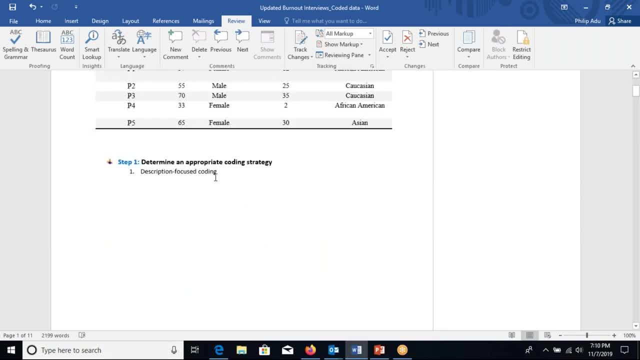 step that you have to do is to choose the determined appropriate coding strategy and for the, in this case, description focus coding will be the best, because you just want to describe what they are telling you. and the second step in the coding process is you have to label your research question right. so 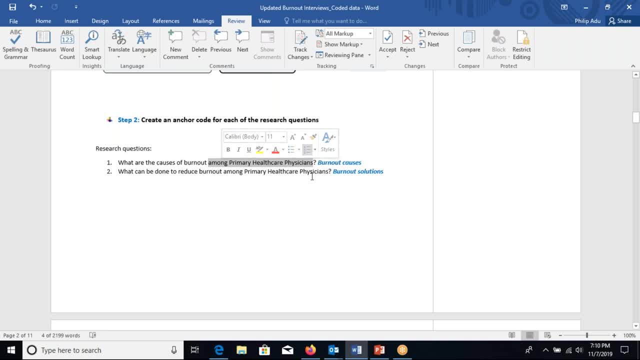 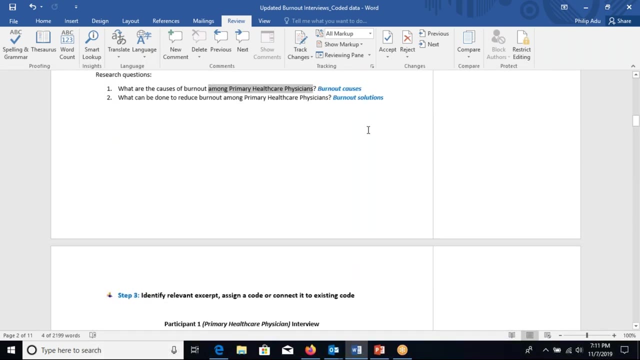 you can see that I've labeled that my first research question label is burnout courses and the second one burnout solutions. right, the reason why you have to label is that you want to develop code under each of the research questions so that, at the end of the day, you'll be able to develop things that 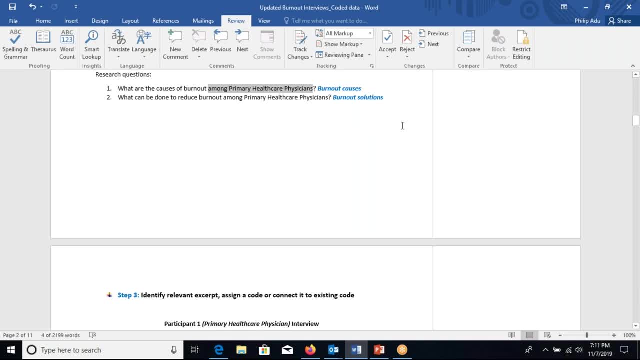 are addressing each of the research questions you don't want to. so labeling your research question helps with the organization of your code, right. that's why you have to label it right, and the label is called anchor code- anchor code- and it's a term that you can use to label your research question, right. so 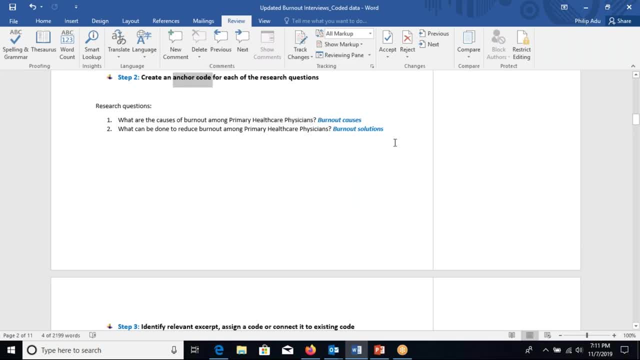 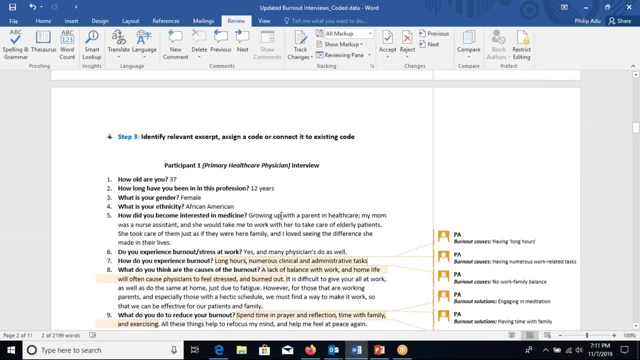 it's a term that is used in my book, right? so you label the research question. what would be the next step? the next step is to go to your participant responses and identify assets or relevant information and then assign code to them. you create code to represent those information, so, as you. 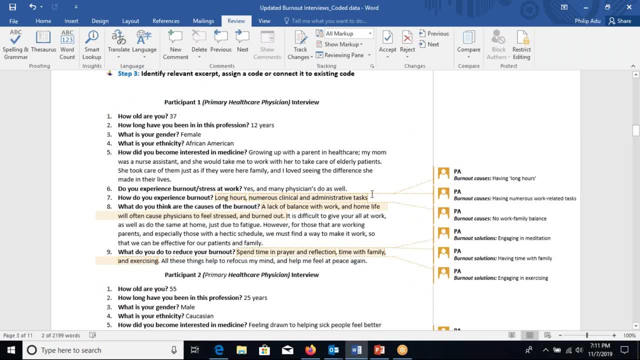 can see here this. this process is called manual coding. right, it's because you are manually go, you are not using a software. if you are using a software, there's a different process. but if you want to use Microsoft Word to do that, when you identify significant information, you- just you know, select. 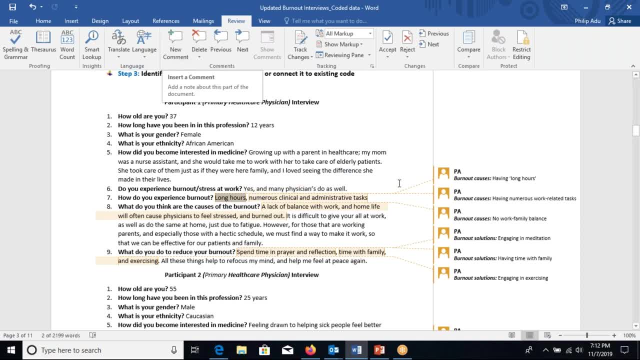 that right. and then you click on comment and then you type: first you first type the anchor code, the label that you gave to the research question. so this significant information will be addressing the first research question. that's why I indicated burnout causes and then column, and then you type the code that you you want to use to represent that. 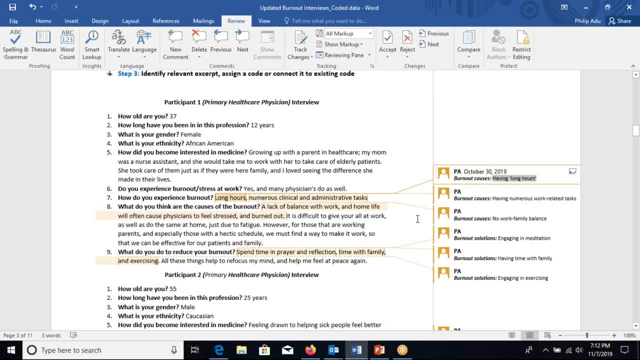 information, right, so you can see here that sometimes you can quote participant as a code, right, the most important is, the code shouldn't be more than five words, you don't? you don't want to be too long, right? it's between two to five words are very good. 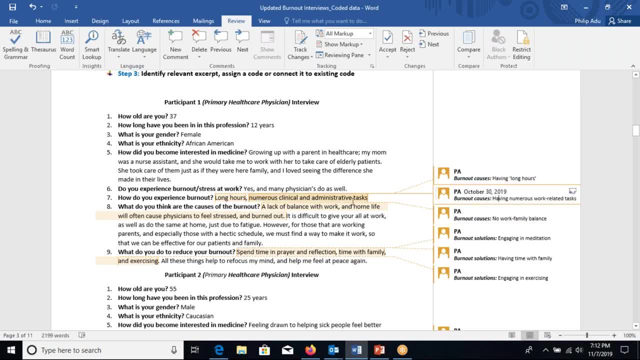 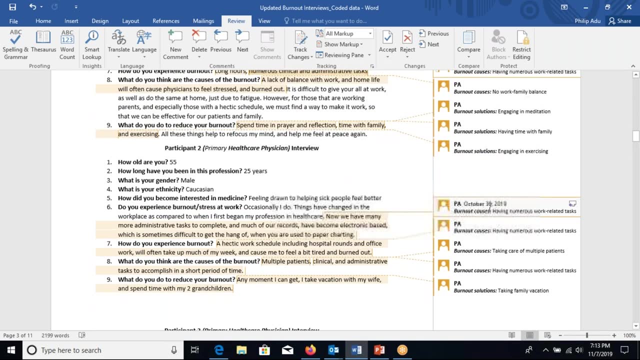 so I went through. you know, when you identify significant information, you develop a code. so sometimes what will happen is that as you are doing the coding, you realize that you have identified significant information that you can use to connect to previously developed code. right, let's say one. 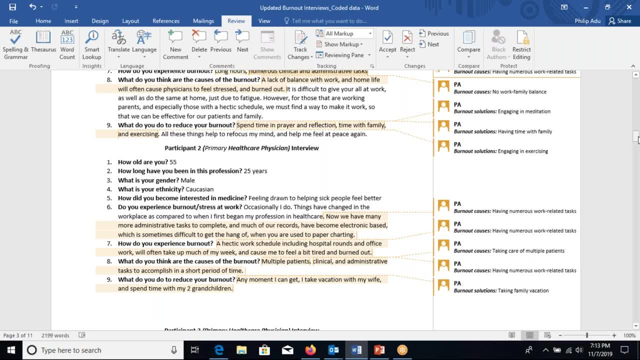 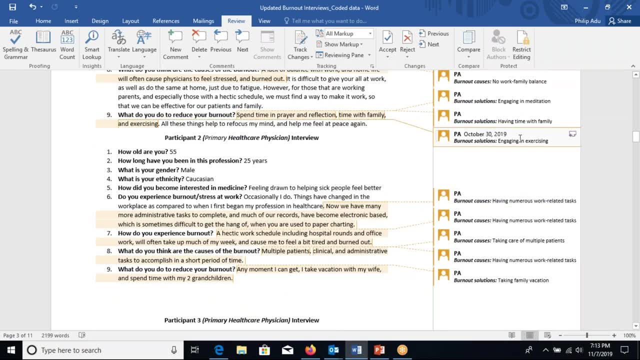 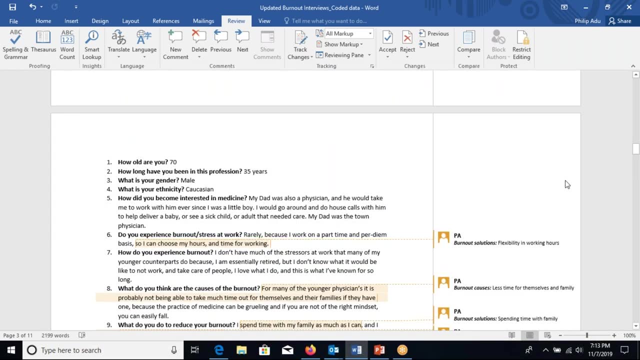 example is. I want to give one example here. so let's say you have develop a called here right engaging in meditation- right. and then another partis Designer talking subtitle, making mixed statement about no engaging in medic medication, assess solution to address India burnout- right. so you use the same code right down in. 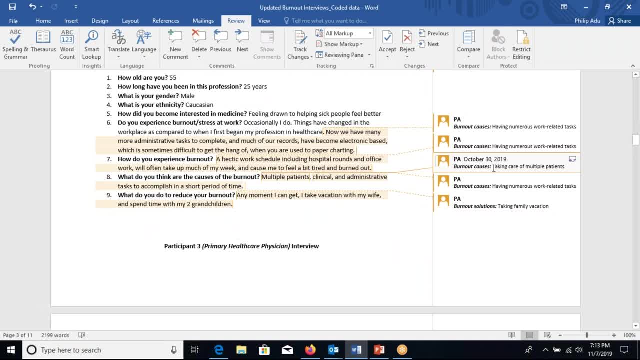 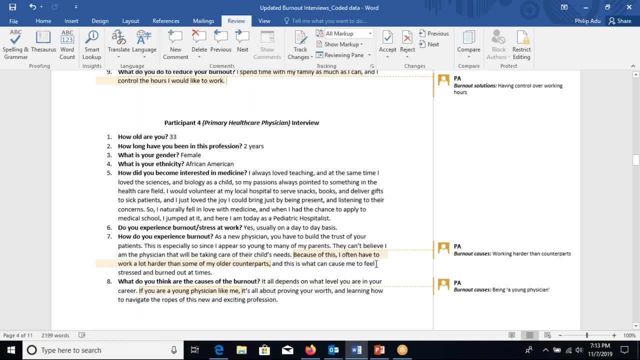 here and that's why I'm on the trouble list- really small, by the way, and if you code that you have already developed to connect to any information that talks about meditation, right? So this means that whenever you identify significant information, you have to ask yourself: is there any existing code that you can use to connect to the significant? 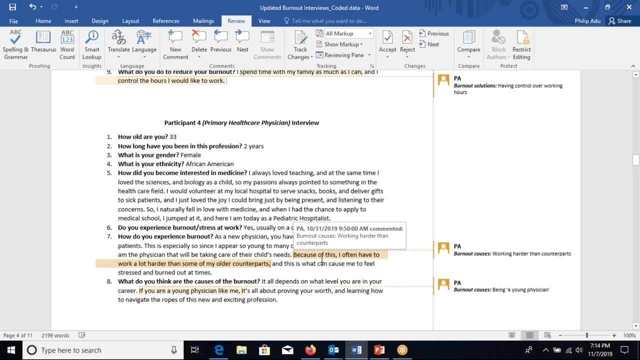 information. If there is no existing, then you can develop a new code, right? So think about. it is this way: You have containers, right? the codes are just containers, and then you go to participant responses and identify significant information and drop it into those containers. 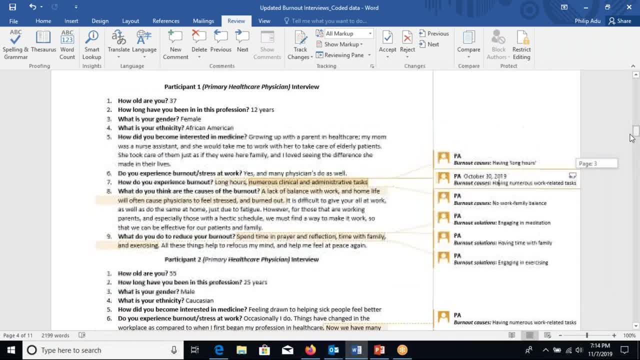 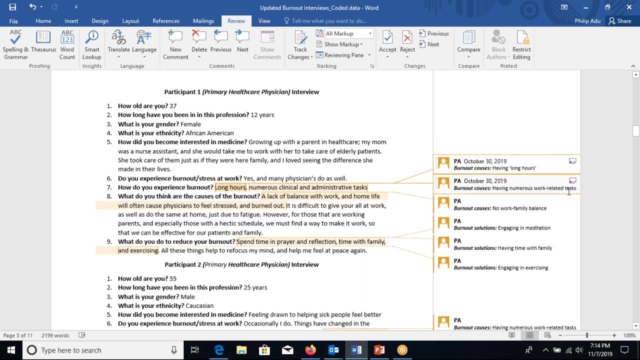 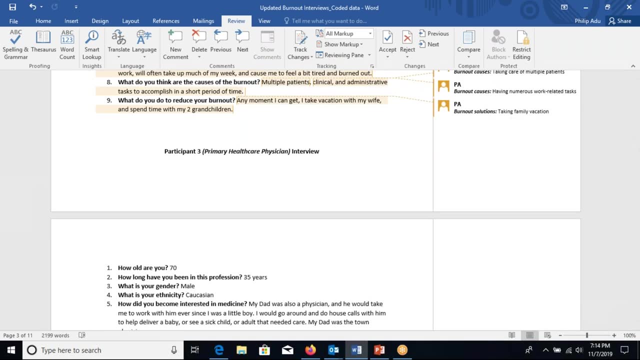 right. so at the beginning you create new containers, right. So I have a container for having long hours. I have container for having numerous work requests, Creating vessel related tax. I have a container for engaging in meditation, right. so as you are going through the participant responses, right, you may identify. 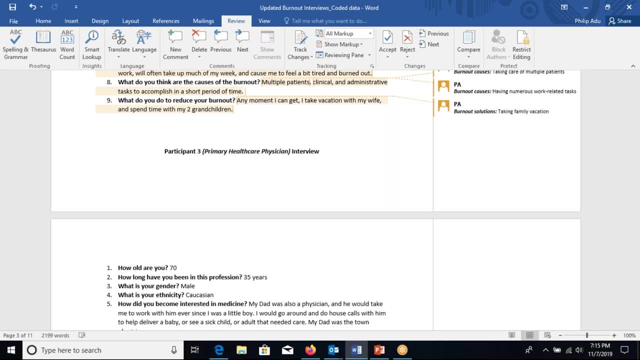 information, that when you identify significant information, you have to go back and look at your previously developed containers and see whether you'll be able to drop those significant information into that if they are related. if you cannot drop it, if it's not related, you create a new container. 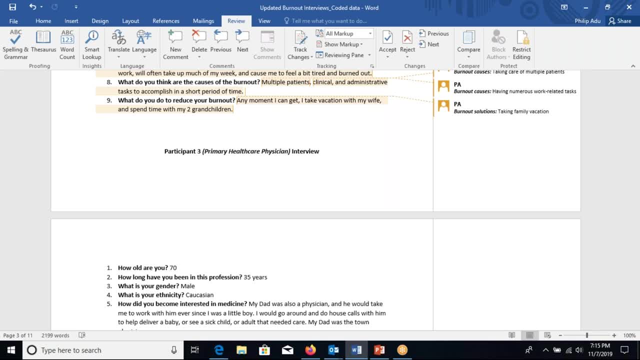 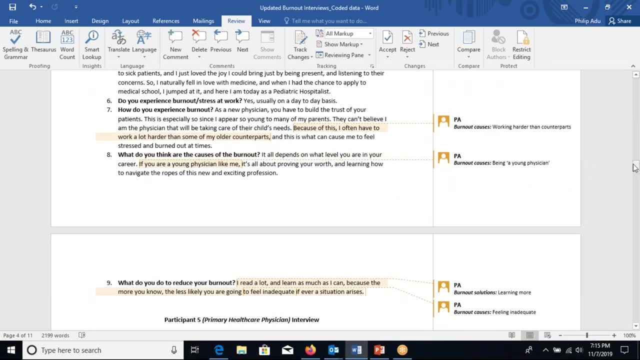 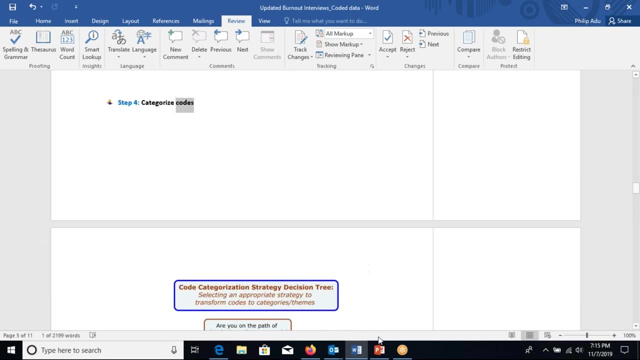 am I making sense right? so this is how the coding process is. so you code, you identify significant information and do that, and then you move to the next stage where you have to categorize the code, and we are going to talk about that. but this is just a brief information about a process. so, as I said, 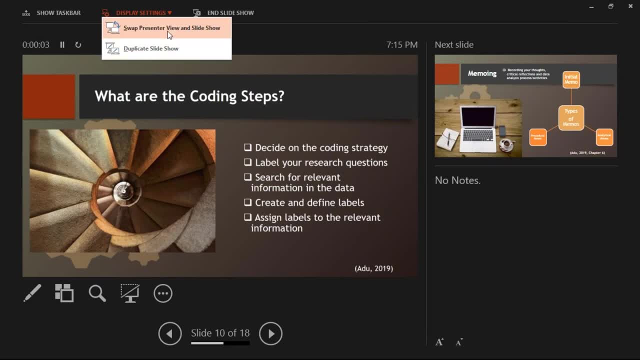 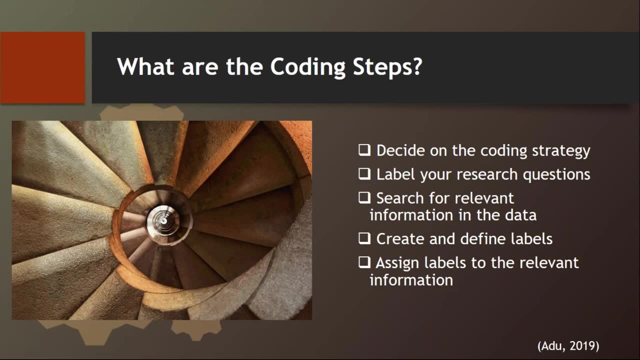 as you can see here, I have a container and I'm going to go back and look at my container. so, as you can see here, you have to first decide the coding strategy right, and then you label your research question and then you go through your data right and identifies relevant information that will help you. 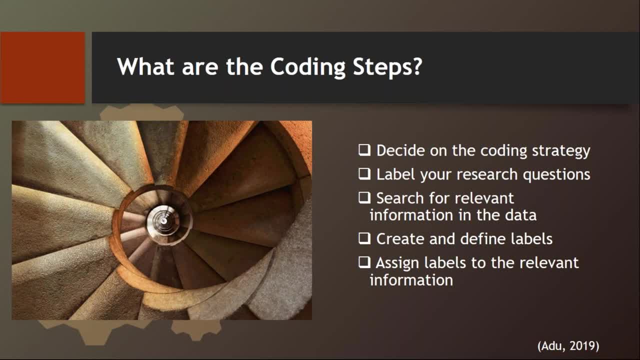 to address the research question and then assign code to them or put them into various containers, right, and then you have to make sure that you have the right to define what you are defining. so this means that when you create a container or a label, you have to define it. so this means that each of the code 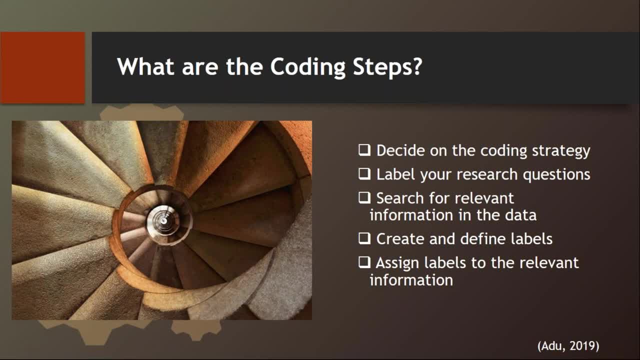 that you develop, you have to define. why do you have to define? so that when you go back and look at it and access of what does meditation mean in the context of what participant told you, you'll be able to know the definition of meditation right, based on the data that you have, so that you'll be able to 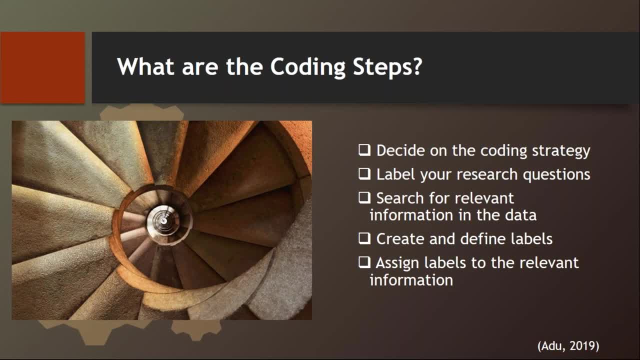 especially when you are doing categorizing- when they are categorizing your or codes, you'll be able to know the meaning of each of the code or what's the code stand for. So it's very important to define them, And I also talk a lot about defining the codes. 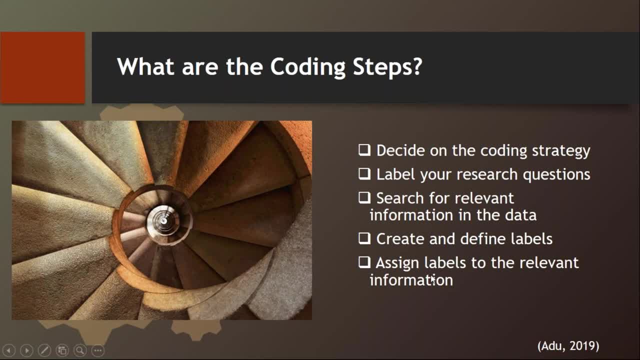 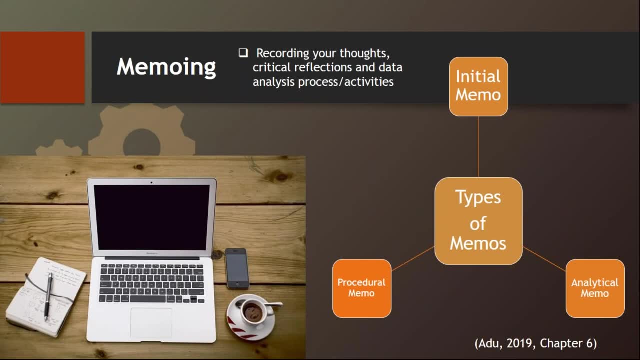 or the labels in my book, Then. so the next step that you have to think about is, as you are developing codes, there will be rich information that will come into mind, Because you don't have time to reflect on great ideas that comes to mind. what do you have to do? 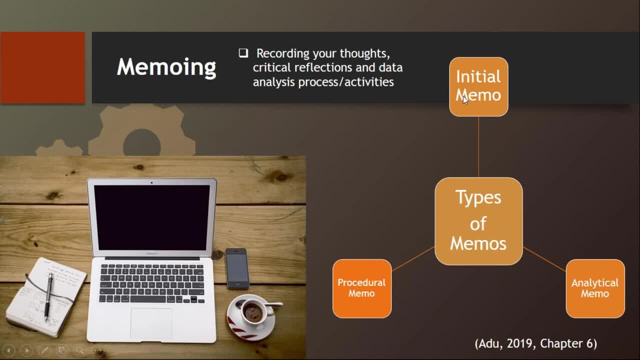 You have to write them down. That is called initial memoing right. So you are recording your thoughts as you are coding your data right. And then, when you finish coding or when you stop in the middle of the coding, you can go back and reflect on your talk. 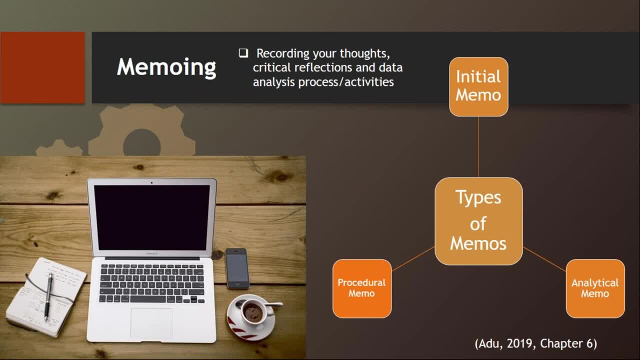 and maybe digest that and maybe create more information or think about it and critically think about it and also write more reflection. That is what will be analytical coding. So you are analyzing your initial thoughts, right, You are during the coding process. you might not be able to pay attention. 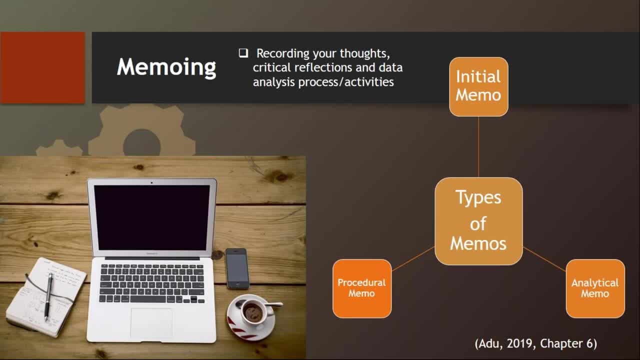 to rich information that comes into mind. That's why you have to record it And then, when you finish coding, you can go back and reflect and add more information to that. And when you are adding more information and analyzing what you have, it's called analytical coding or memoing right. 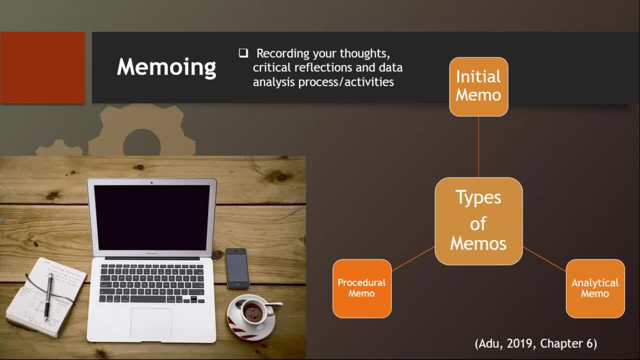 Reflection of what you have already written. right And procedural coding is all about no memoing. It's all about memory. It's all about recording the step-by-step process. The reason why you have to record it is sometimes when you are presenting your findings. 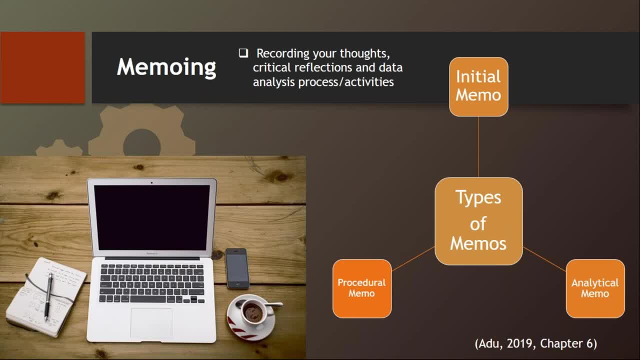 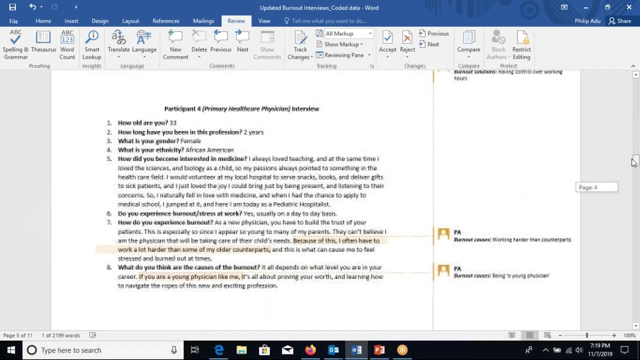 people want to know the process and you have to document the process so that they'll believe what you found. So this is where you record what you are doing, the step-by-step. So the same thing that I did here by telling you the steps that I took to develop. 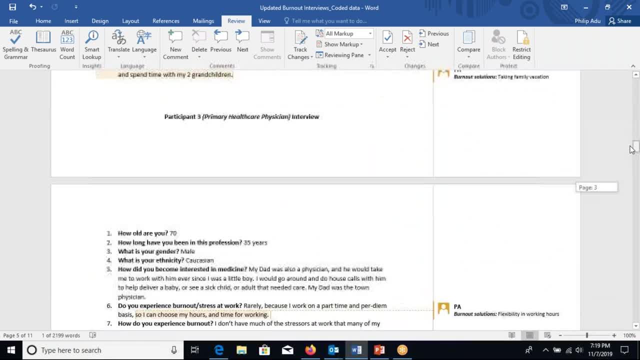 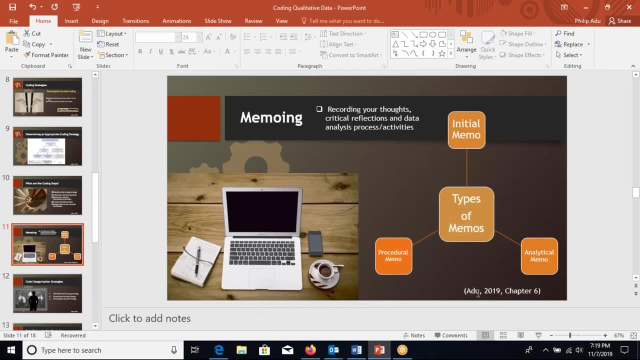 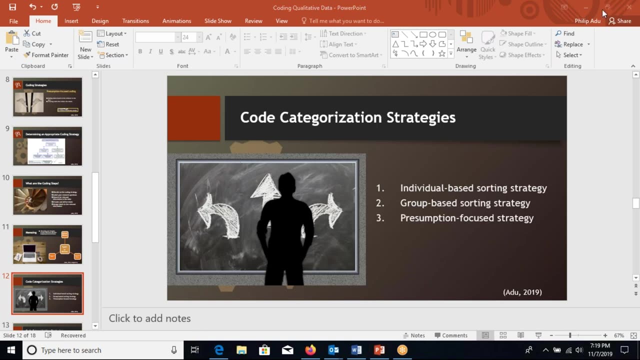 codes. you can, you know, list the steps now so that you'll be able to share it with them, with your audience. So that's how you're going to do it. Any question? Is there any place that I have to explain further? 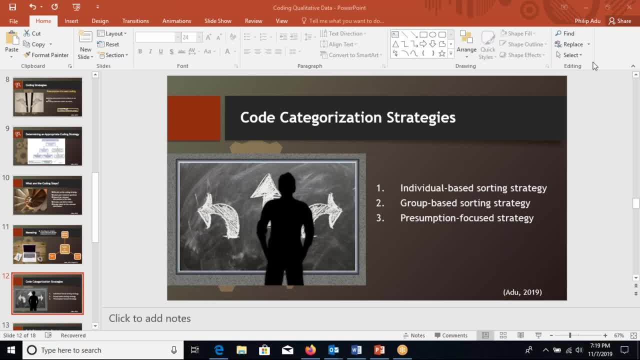 for you to understand. I think it's pretty simple, but that might be because I understand it. I do have some questions, Dr Adu, but I want to wait until when's the appropriate time, Like I often have conversations with students. 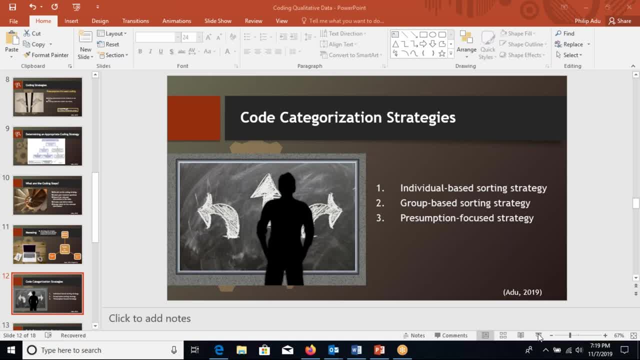 in this process about the difference between descriptive and interpretive coding and when is right, And so all the things that you're describing are just part of the process, but I get students sometimes who are, almost wanna say, stuck in descriptive coding when they really need to move into a more interpretive space. 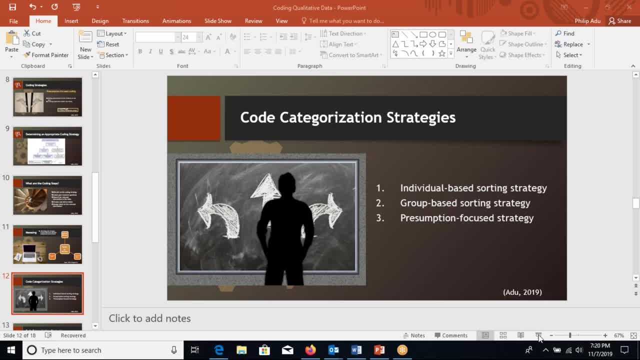 based on what their research questions are, or even their design. Can you talk about that? Yeah, so I always show them a table. I don't have it here. I posted to all my LinkedIn And that table is also in the book. 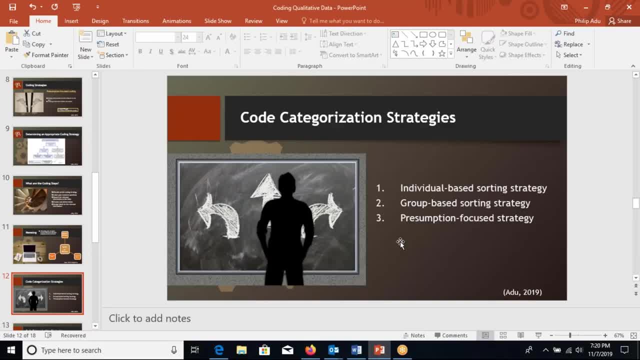 I gave information about if you are using this. If you are using phenomenological approach, what kind of coding strategies do you have to use? If you are using graded theory, what kind of coding strategy that you have to use? If you are using interpretative phenomenological analysis, what coding strategy that you have? 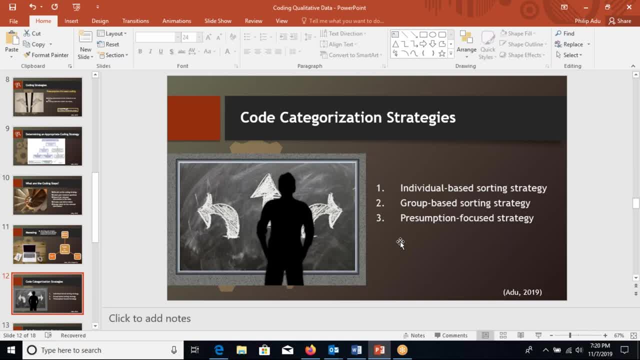 to use It's all about. it's sometimes difficult to determine, but I try to differentiate between them. So, in terms of the levels, right, the first level of coding is descriptive, and normally you use descriptive coding when you are doing a narrative study, because narrative study 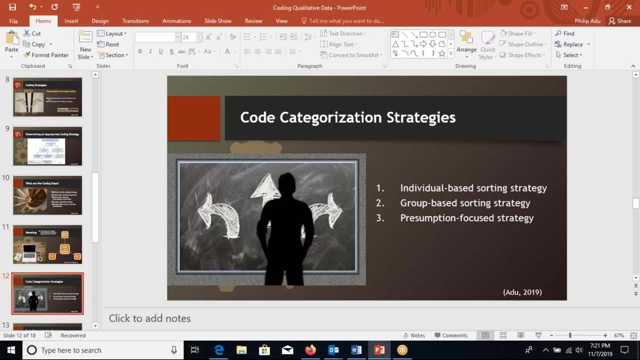 is all about describing participant stories right. Sometimes, when you are doing a phenomenological study where you want to describe participant experience without bringing in your own intelligence, If you are using descriptive representation, then descriptive description focused coding will be the best right. 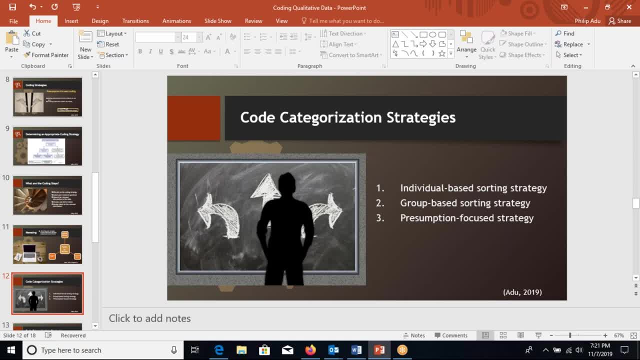 Sometimes, although the research question is more of descriptive, but maybe the data, when you look at the data, when you review the data, you realize that answers to the questions are hidden. You have to make sense of the data before you can address the research. 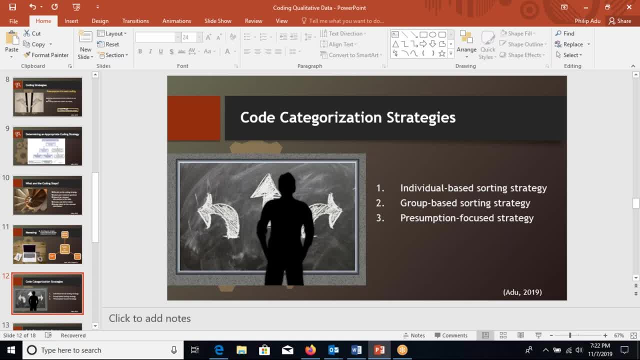 Right such question, then the interpretation focused coding will be the best. You have to make sense. You have to ask yourself: what does the participant information mean? right, And then, based on that, you can develop code. So sometimes it depends on the nature of the data that you have. 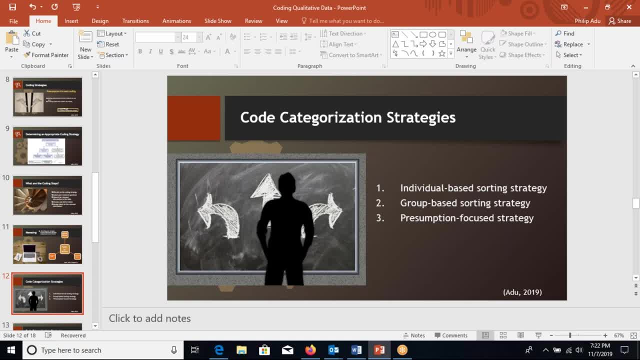 It also depends on the purpose of the study. If your purpose of the study is more of descriptive in nature- you are describing the participant experience, you are describing that event- then descriptive is the best. But if the data that you have is the information that you need is hidden, especially when you 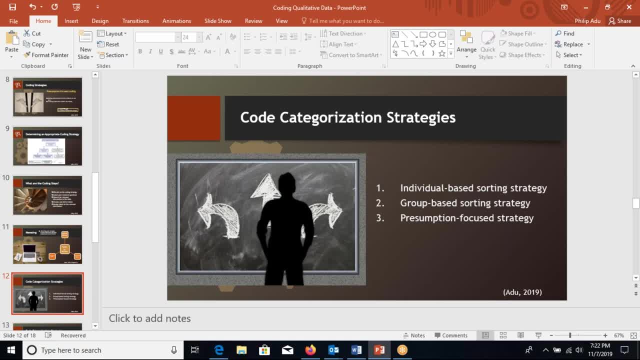 are dealing with documents, right? Maybe you collect a document and the documents were not generated to directly address your research question. It was maybe generated years ago, right? And you are using your research question, So you have to make sense of the data. 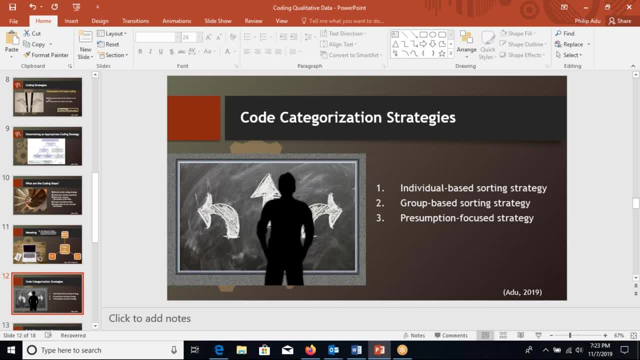 So in this case, interpretation focused coding will be the best. Presumption focused coding normally is used when you want to develop a theory, right. You want to develop an explanation to represent an issue, or you want to explain a concept or a phenomenon- right. 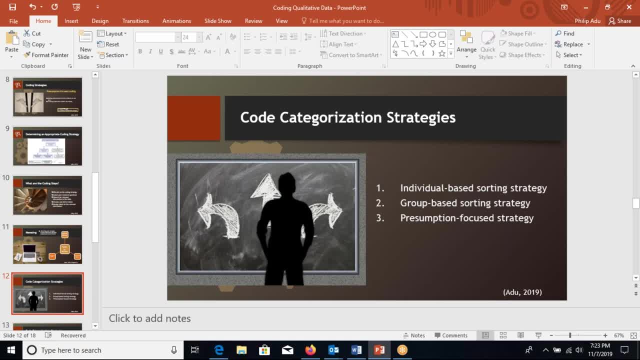 And most of the time, those who are using a grounded theory are using the presumption focused coding. Thank you very much, You're welcome. So the next one that you have to think: after you have coded your data, you realize that you have a lot of codes. 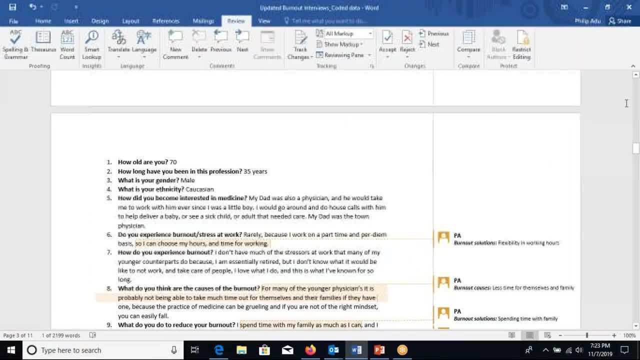 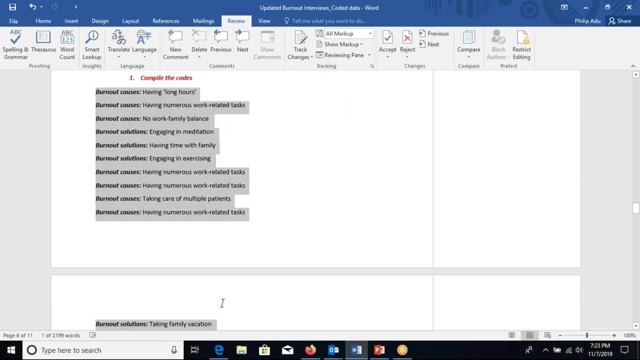 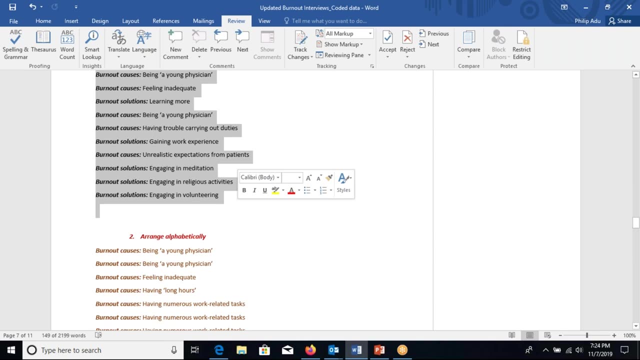 And, as you can see from this example, I have, so I have a lot. So these are the codes I've created. It's a lot. This is as you can see here. I cannot present all this information to my audience, right. 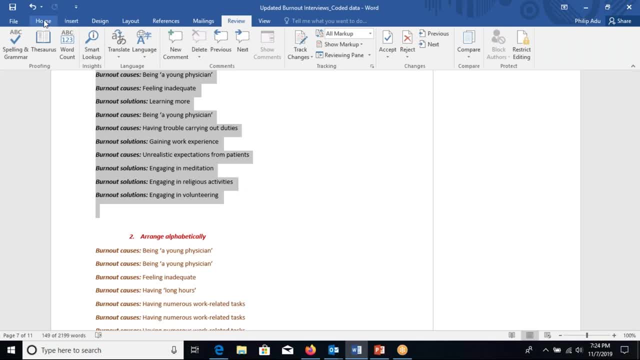 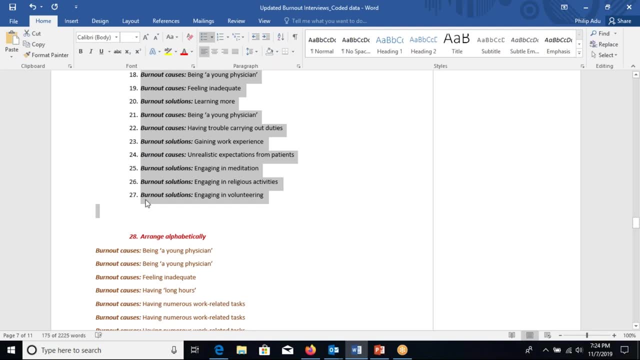 Because I have to talk about each of them and let me see the numbers here. So there are 27 things that I have to talk to my audience and they don't have time to listen to everything. So you have to move to the next step, where you have to categorize what you have developed. 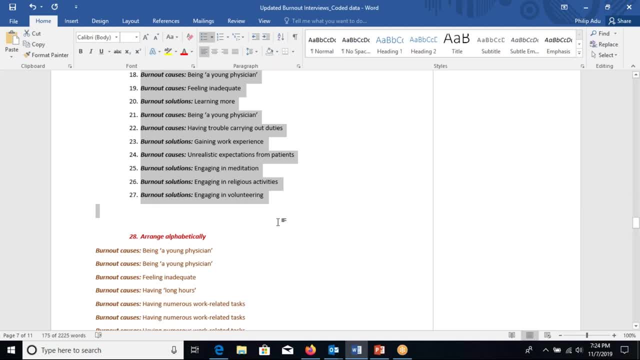 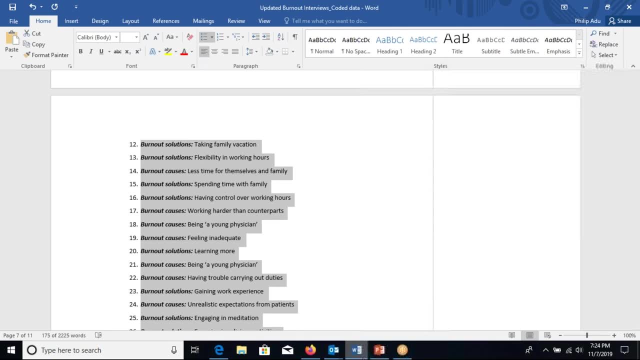 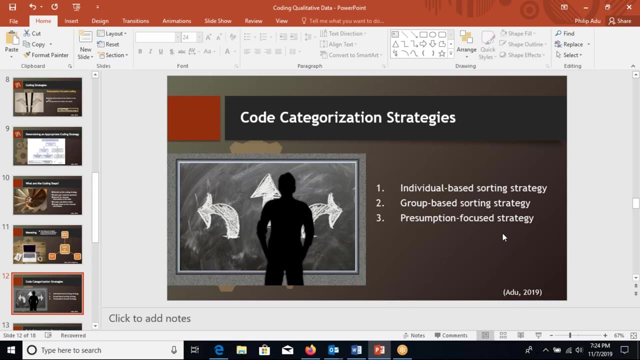 Right, And that's why you have to- you know, you have to determine the categorization strategy that you can use right, And we have three main types. We have individual-based sorting strategy, group-based sorting strategy and presumption focused strategy. 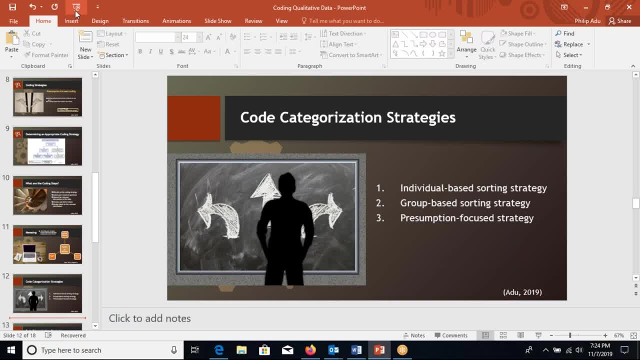 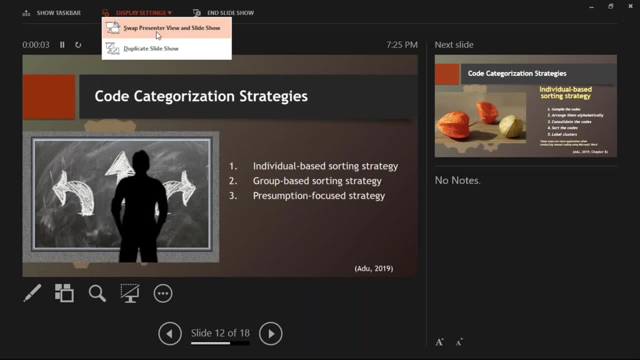 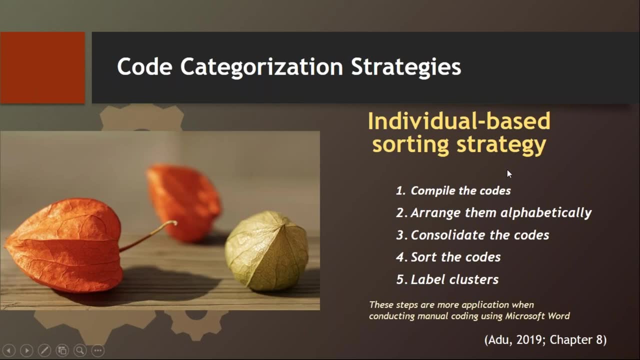 And I explain. let me pull this one up again. Okay, So the individual-based sorting strategy. Sorting is all about grouping them based on similarities, right So? and the essence of doing that is to come up with few themes to help you to address. 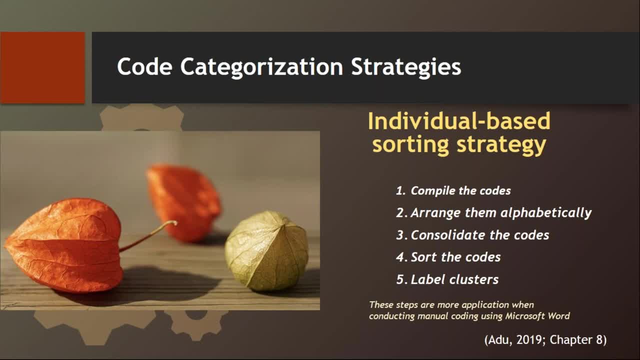 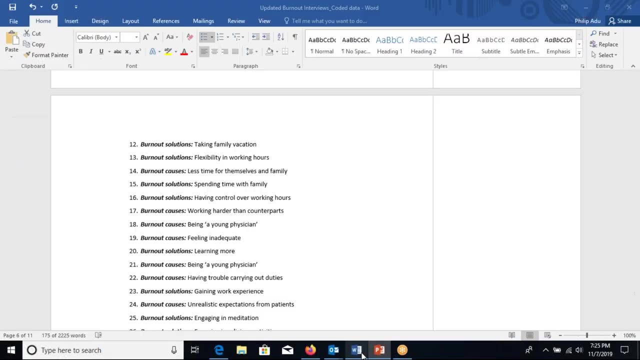 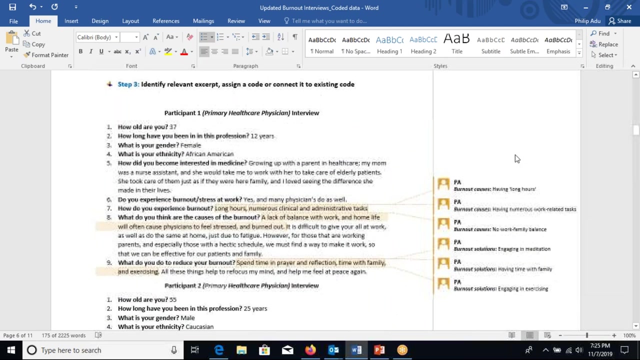 the research question, maybe six or five themes or four themes to address your research question that you have. Okay, So if you are doing a manual coding, right, this is how the sorting happens. So what I did here is, after coding all the data, I just select one of the and I select. 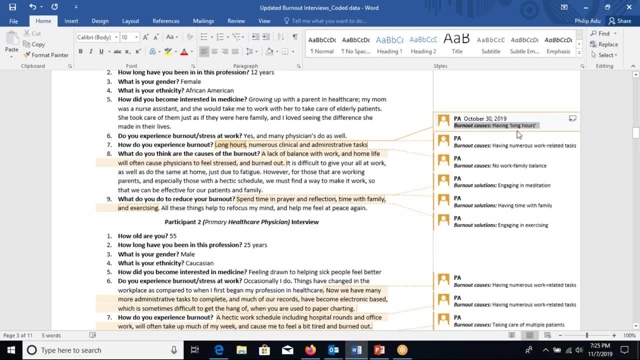 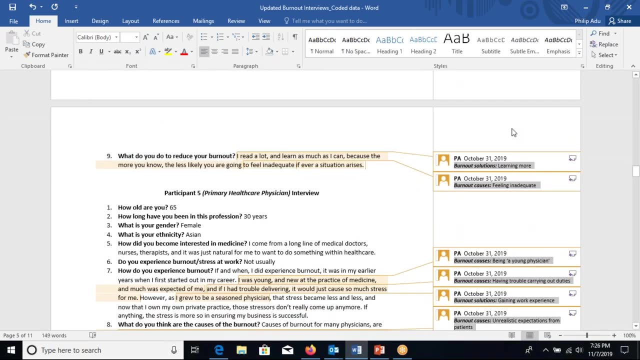 the first comment, the first code that I've created: select everything and click on the shift, Okay. And then I click on down arrow on the keyboard and then to select everything And then, after making sure that everything is selected, you right click on one of them. 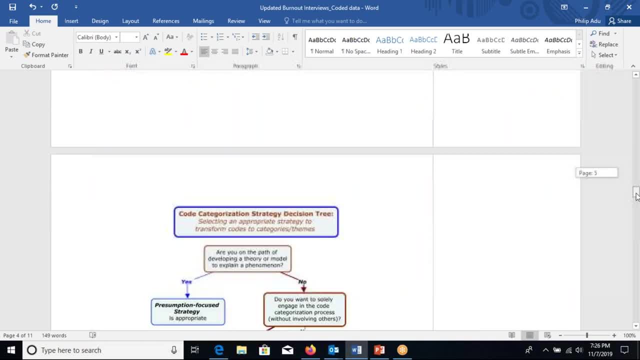 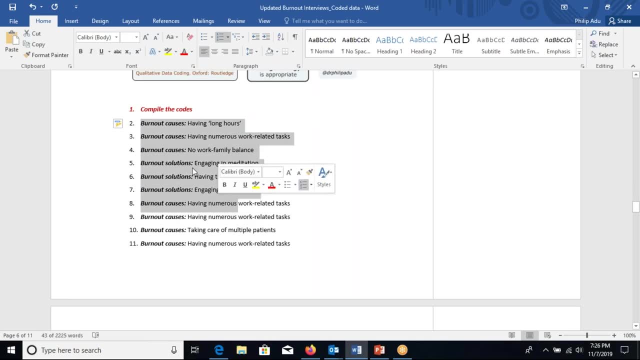 and copy And then you click on copy and then you paste it under here, under your document. So this is how I was able to get these all the codes. Okay, So this is how I was able to get these all the codes. 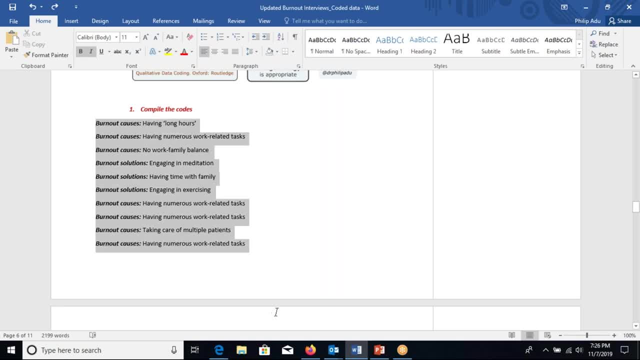 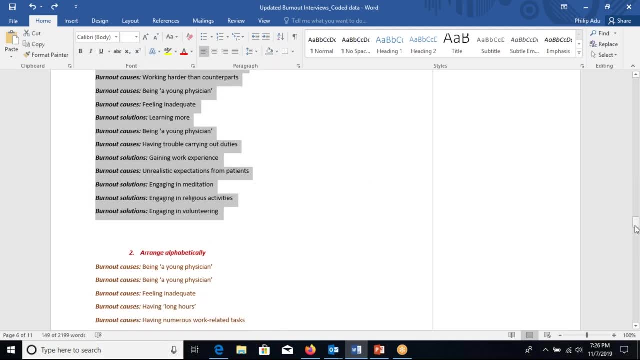 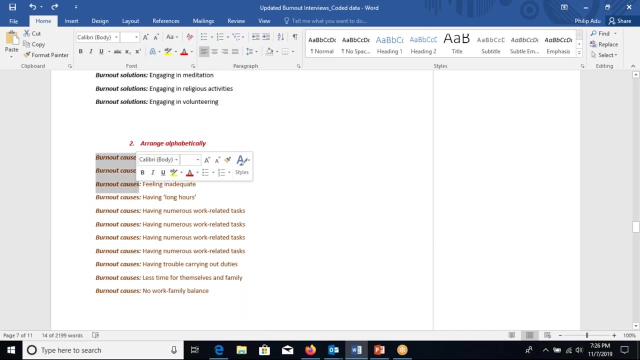 Okay, So this is how I was able to get these all the codes. Okay, So I clicked on the right button, right? So I copied and pasted them here. So after that, what do you have to do next? You have to arrange it alphabetically so that you'll be able to separate the first research. 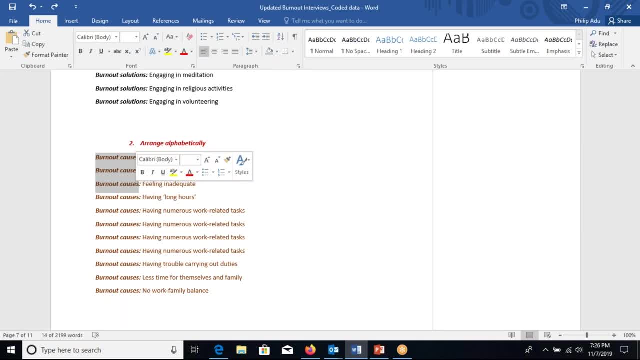 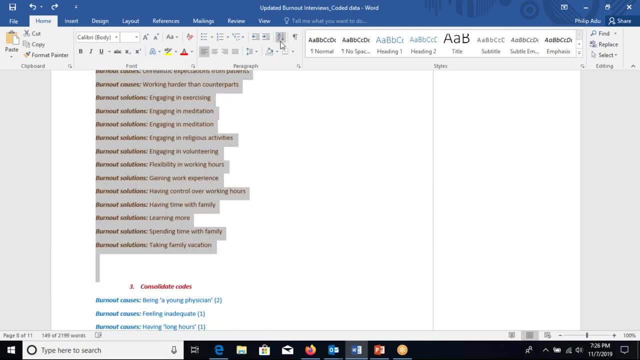 question. codes that are related to the first research question from the codes that are related to the second research question. Right, So I just selected it, and then I click on this icon A to Z, Okay, the sort- and then to arrange it alphabetically for me, And then the next step is consolidate. 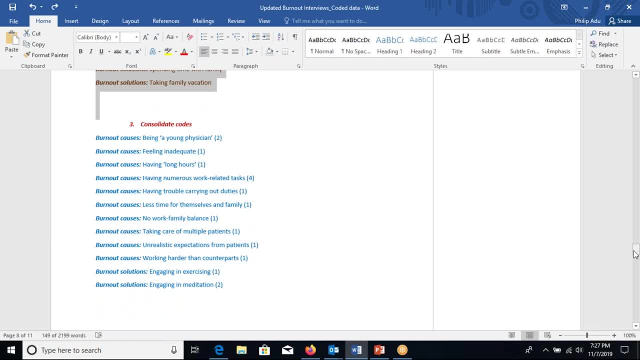 right the codes. How do you consolidate the code? I find it quite difficult to pronounce this one. So you know I mentioned that sometimes you will be able to have a code assigned to more than one significant information. So this code has been assigned to two. 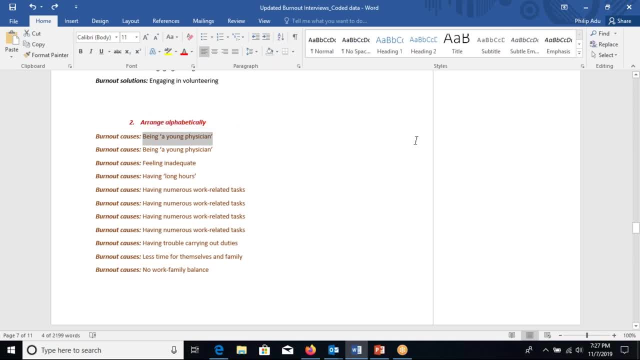 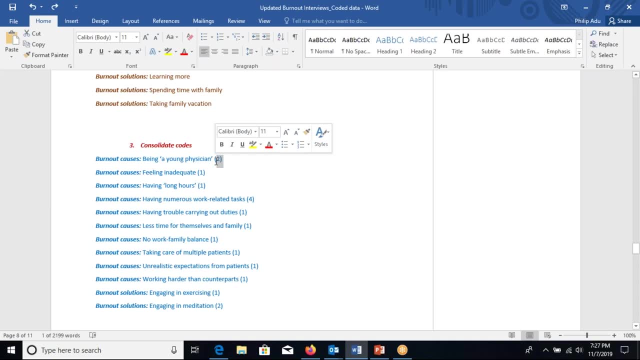 significant information, right? So when you want to put them together, you just delete one of them and then in parentheses you indicate two, because there are two significant information that were connected to this code, right? So two means that you have identified, you went through the data, you identified two relevant information and then 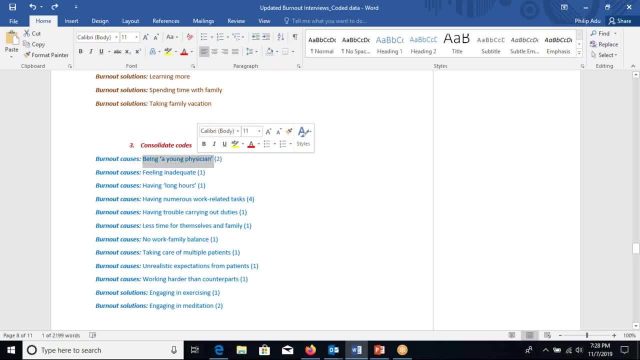 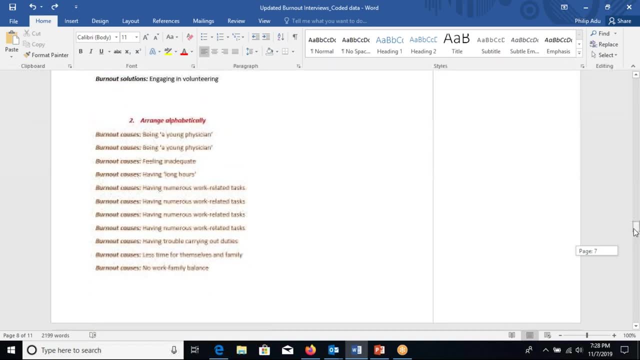 and put it in this basket or in this information, in this code, And then you do the same thing. So you go to, you can see that here we have only one code. that was one significant information that was connected to this code, right, because it's only one, filling in inadequate, So you just indicate one. 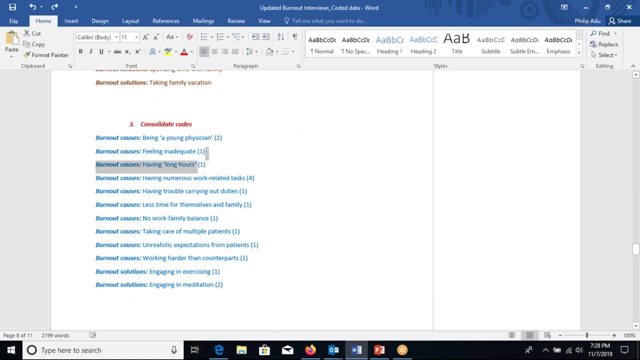 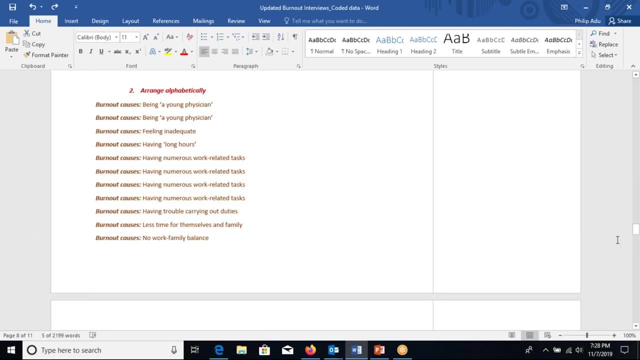 right and the same thing as for the second one. So you just go through and you can see that having numerous work-related tags. You can see here that having numerous work-related tags, there are four right, one, two, three, four, So this code were connected to four significant 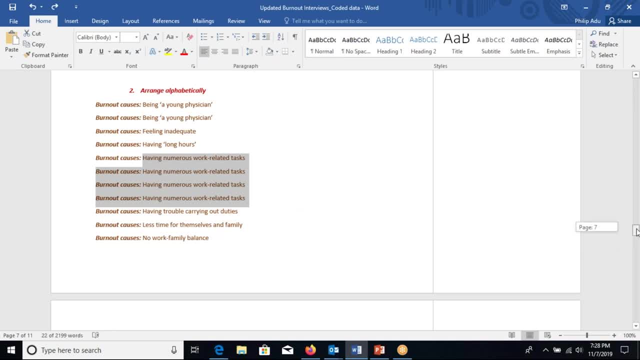 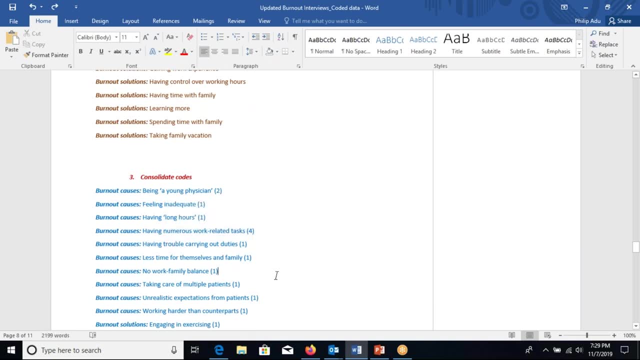 significant information. So we delete and then only maintain one, and then in parentheses you indicate four, right, So that will help you. So why are you doing all these things? It will give you information that, okay, we have not a perception per se. we have. 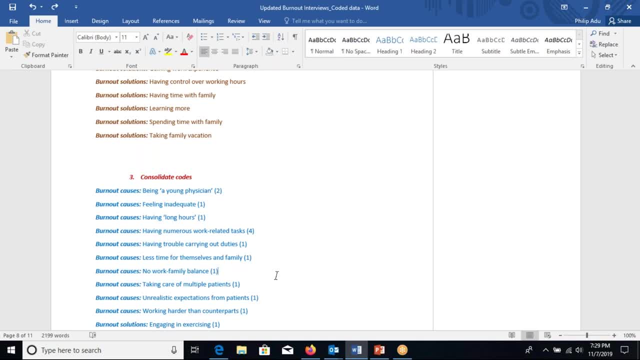 a thinking that the more participants talk about an issue, the more likely that issue is important. So if the participants are talking about this four times, this means that you know most of the causes of having numerous work-related tags is one of the main causes of right burnout. right. 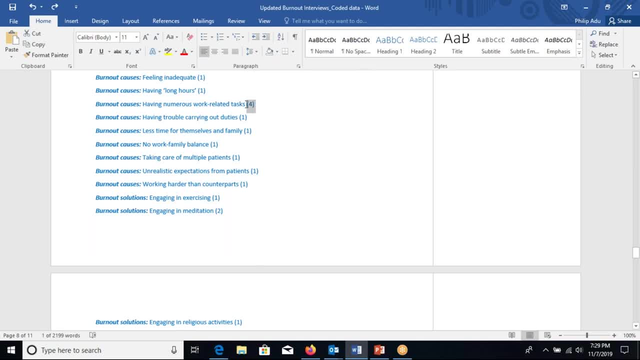 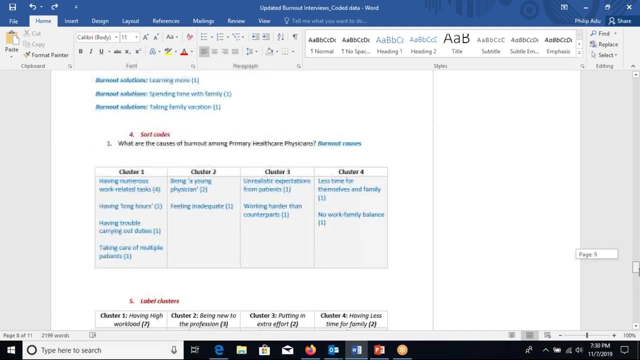 So the more the number or the more significant information, the likelihood that that information is limited, right, Right, I can see that information is very important, right so? so you can't compare everything. and the next step is the sorting individual. the reason one is individualized, sorted, is: 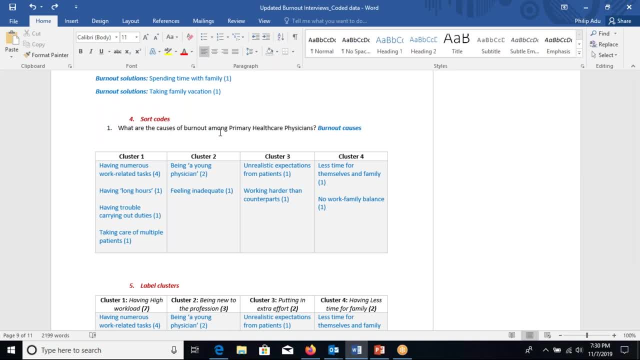 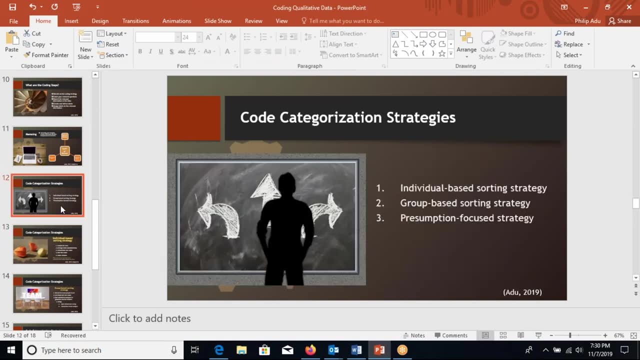 that you, as a researcher, you are doing it yourself. right, individual sorting, and we have the group one, and I will talk about a group one later. the second one, group with the group, means that you are involving people to help you to sort what you have. and then presumption- I'll also talk about it, but I just want you. 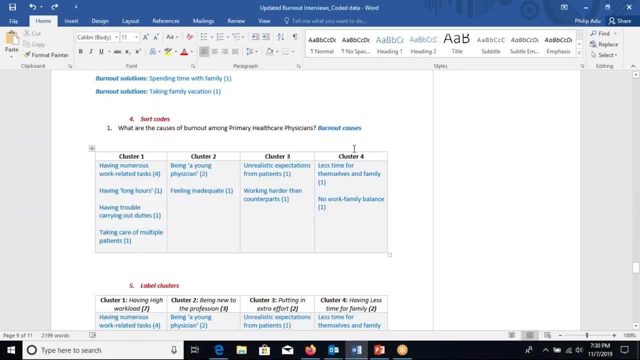 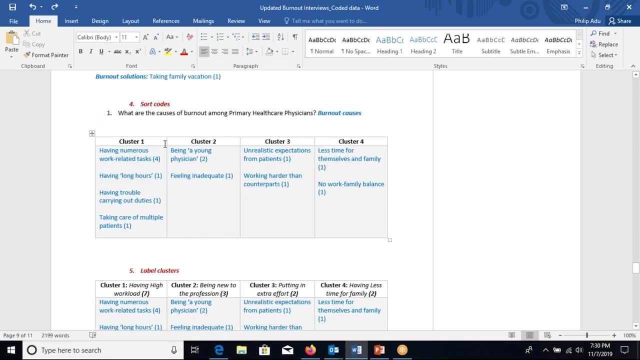 to understand the first one, which is the one that a lot of students use, because they do analysis themselves without involving anybody right? so the sorting is one thing that you have to do is you can have a table right with about four or five columns right and then 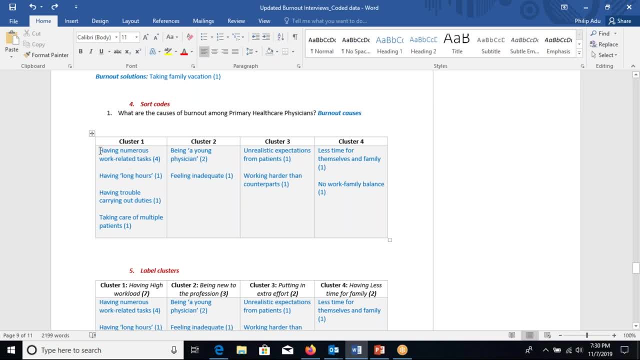 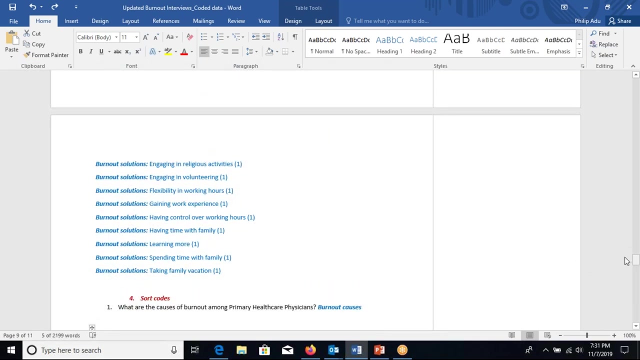 you first put the important code here. the important code is that the most important code is the one that have highest frequency or highest number of significant information collected. so you can see that you can put it first. you can put it here right in the first column, and then you go to the relevant. 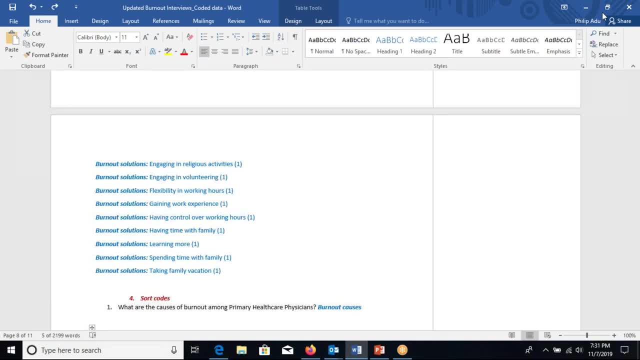 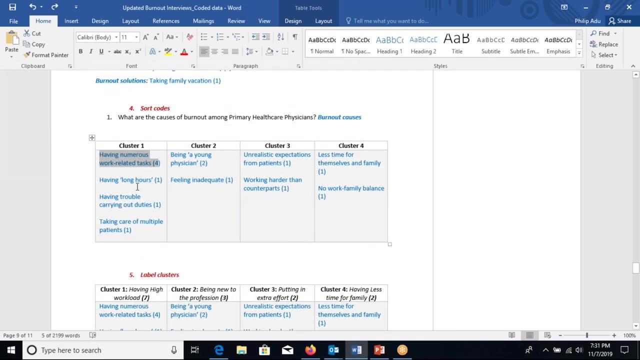 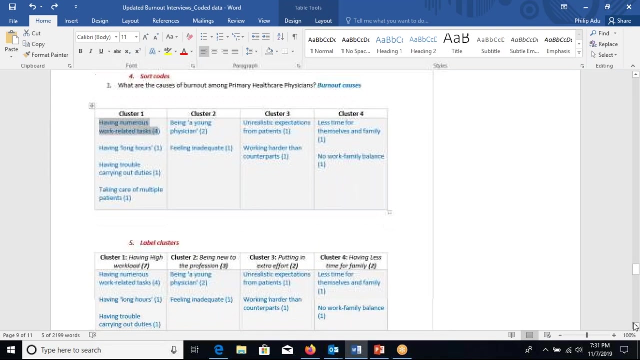 information. you go to the okay, so you go through and then see whether you can group them based on how they are related. so I was able to put them to the various classes and then, after putting them into classes, you have to label the cluster right. so, based on 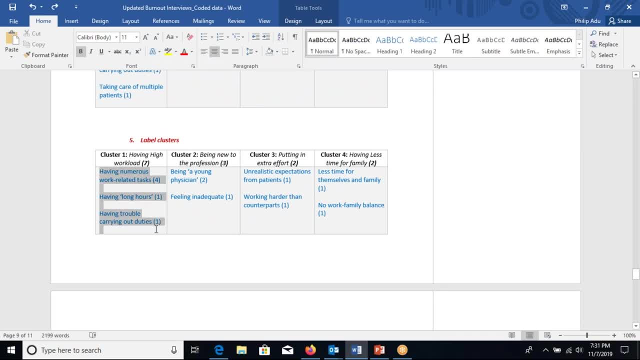 the content or they based on the content in the cluster. what label do you use and you want to give to it? and these labels will be the themes that will help you to address the research question. so for the research question one, I have four themes right, and then I did the same thing for the research question two. 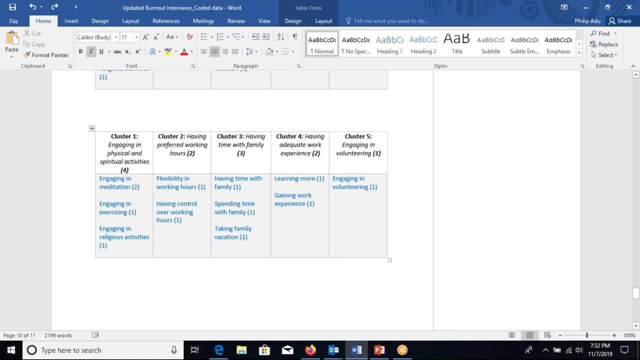 and I have five themes and you can see that I have four here. this means that I added everything, the significant information. one plus one plus two is four. one plus one, two. so this information will help you up, to help you to understand the most important theme. right, so I can see. 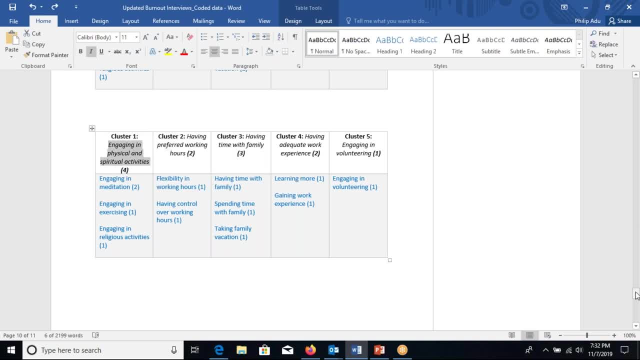 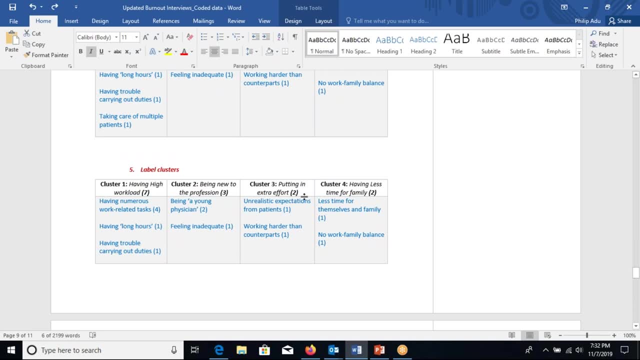 that this one is most important theme because of the number of significant information connected to it, and you can see that this one has seven, compared to the others have three, two and two. so this one is the most important cause of burnout, right? so this is how you can do it in terms of the sorting. so do you? 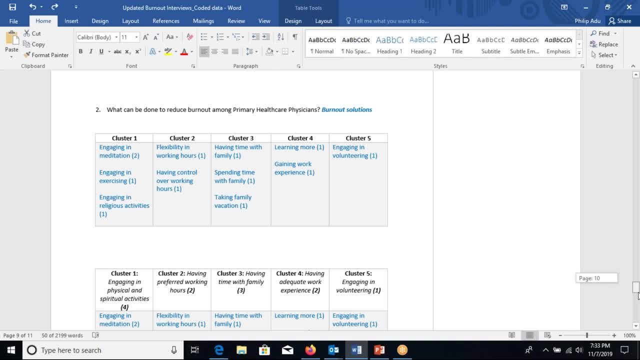 have any question for me, if you are not. Maria was asking about what are you using to do the codes I talking about like this software that I'm using right? oh, so in my book I have I talk about three software's. do we have something like software? we don't. 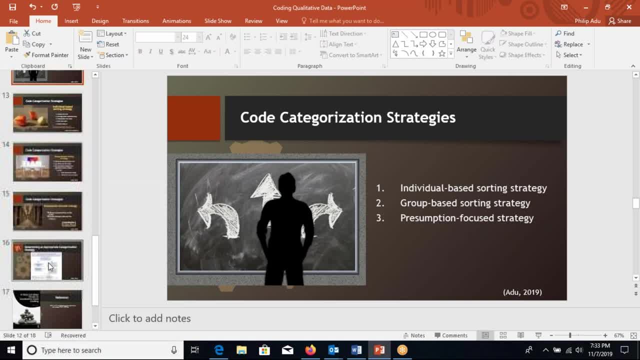 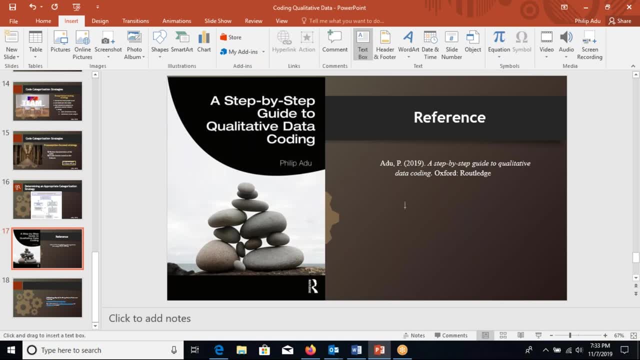 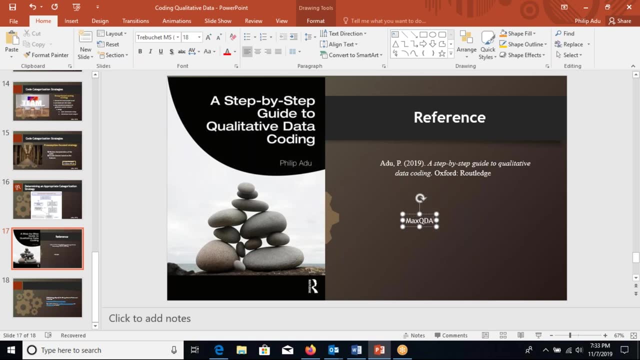 have okay, today software, so there, let me type them here. you know, doctor, do? they are using max Q D a in this course and so they'll start next week. yeah, next week this match will call them, but they've been practicing okay, so my book I didn't. 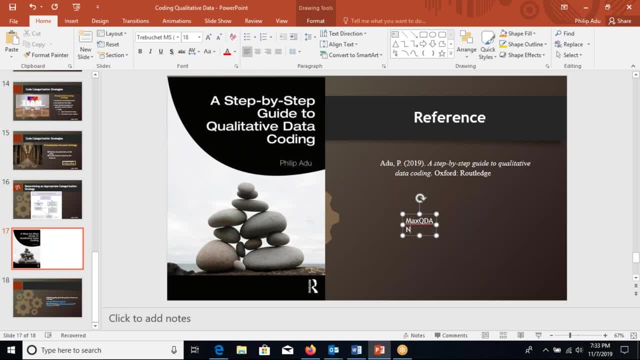 use max QDA, similar to in vivo, and then I also use the deuce. the deuce is as qualitative software online that you can use. I also use a free, free qualitative software called Q DA- my lie, so it's a free software that I could use. so these are. 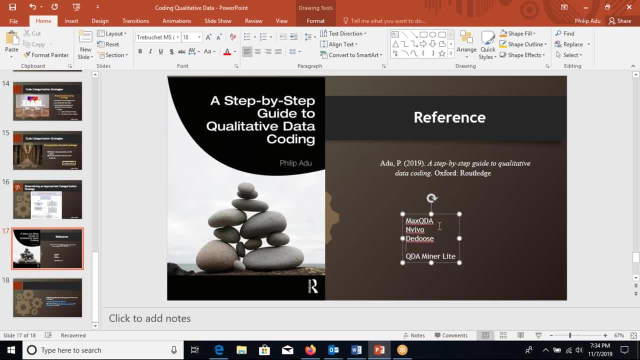 the three softwares that I use for my book, but I think also QDA. My QDA is also very good. it's easy to use, similar to in vivo. yeah, and also I, you, I also. you see you canION screen. we just give the instrument, the phone, then you can use these things trabalho. 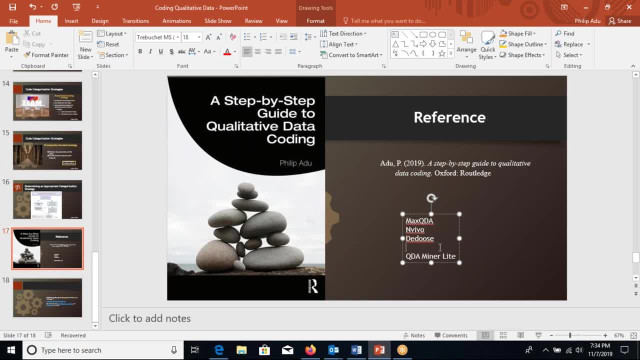 you see, here you can you create your files one minute. there is a link to the the use Microsoft Word for the manual coding for students who don't want to use any software and they want to do it manually, And so let me make a comment about that. 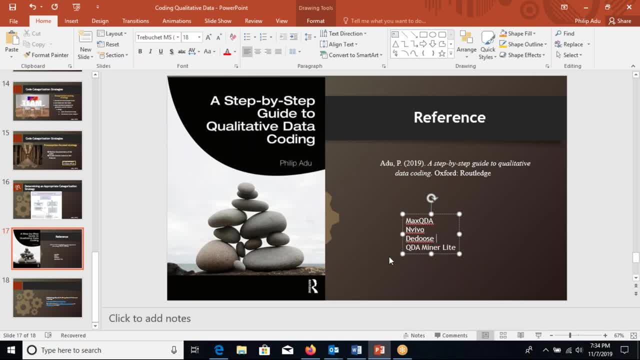 I think, yeah, multiple options on how you can approach it, And I think manual is still maybe somewhat misleading. right, Because you still are using some type of technology to pull some things together, But what you just want to do is still very much, it's not the drag and drop that you 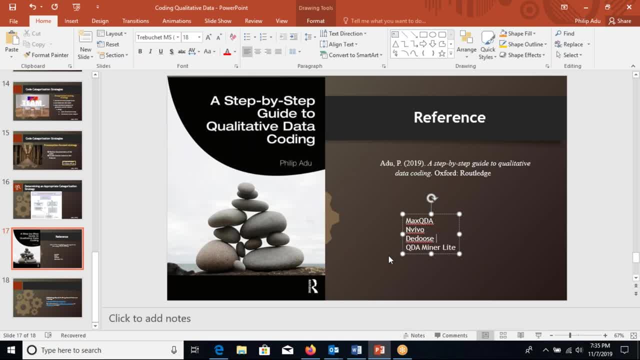 get with some of the software options, so Deduce and InVivo or MaxQDA, but it still allows you to do the things you're doing. I mean to code, assign meaning, numbers, categorize, but understand, I think for all. 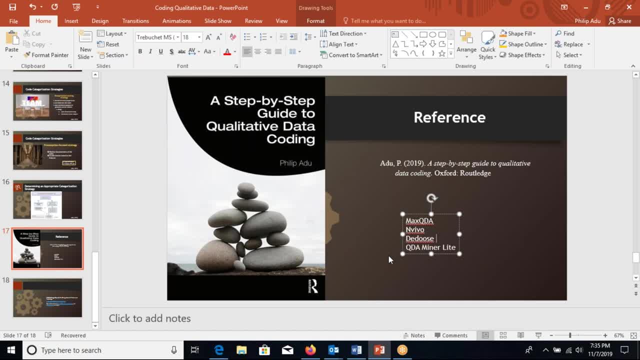 of you. the data set, The data set that Dr Adu is looking at- is pretty small and simple to manage. Some of you, if you're going to have 20 interviews or more and you might have an interview, that each of those interviews might turn into 16 to 20 pages of data. it becomes quite a bit. 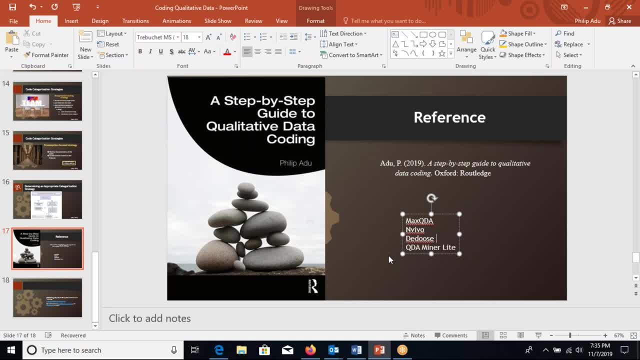 to manage manually. Mm-hmm, I completely agree. I even said in my book that if you are using manual coding, then you have to have a small amount of data. If you have a big amount of data, then you have to use manual coding. 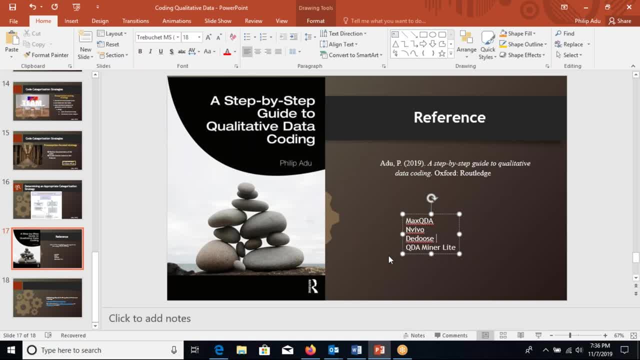 Then you have to use a software because it will also help you with the organization of the codes right. So in the software for manual coding, like using the Microsoft, where you have to count and sometimes you might make mistakes and doing the counting or telling the codes- 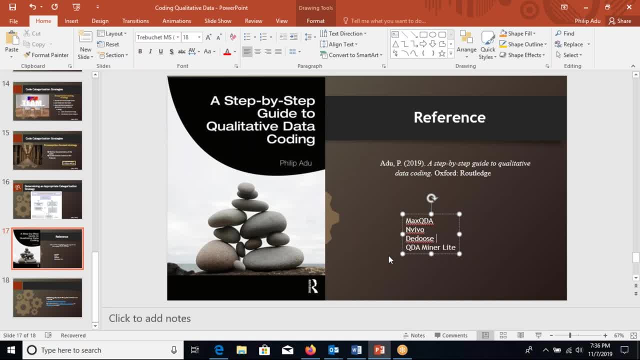 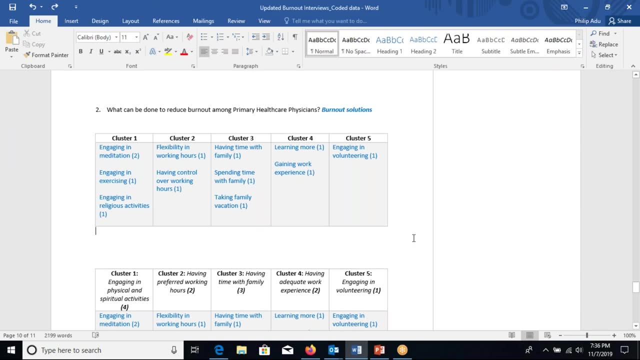 So it's always good to use software. Yeah, Yeah, and you are right concerning the manual coding. Yeah, Because for this one, sometimes I also I call, sometimes I call this electronic coding because, as you said, you are using technically, you are using technology to code right. 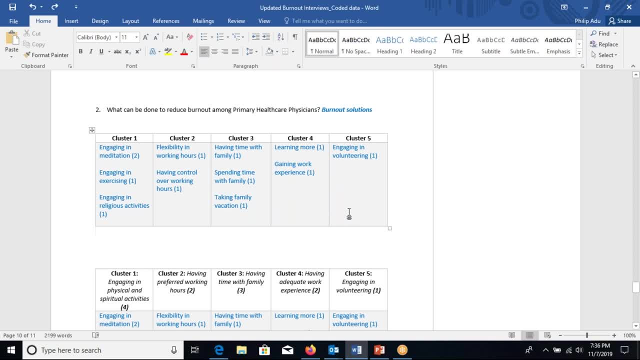 But most of the researchers categorize this process as manual, because you are counting them yourself, You are compiling them yourself and trying to put things together yourself instead of using the software. that the software can help you to tally the automatically tally the number of significant information connected to the code. yeah, 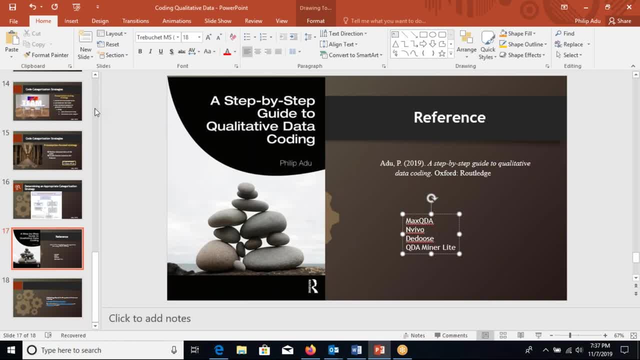 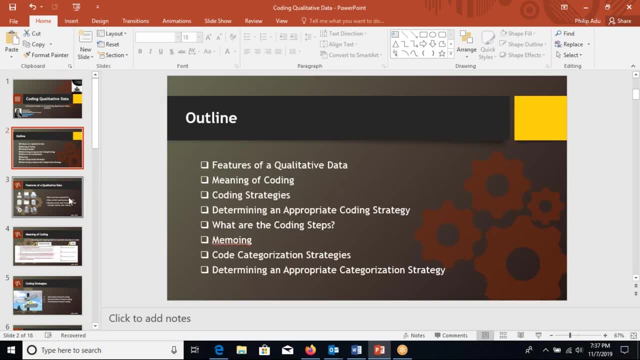 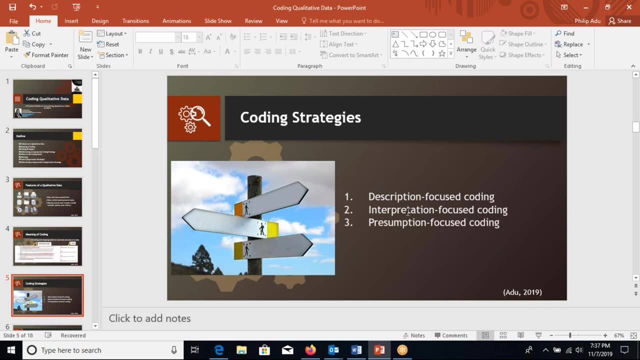 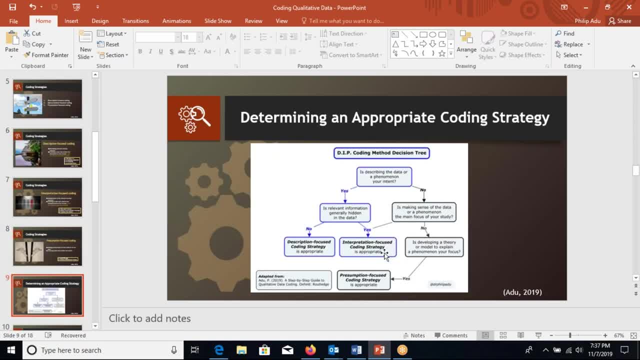 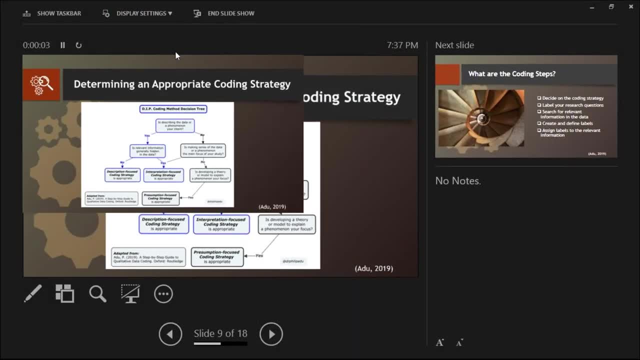 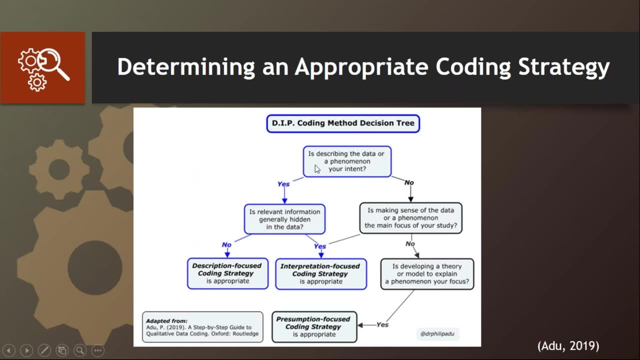 Let me see. I think this diagram will be able to help. Yeah, Okay, So Okay, Okay. that you have to ask yourself is: is describing the data or a phenomenon your intent, right? Is it the purpose of your study to describe a phenomenon or describe the data that you have? 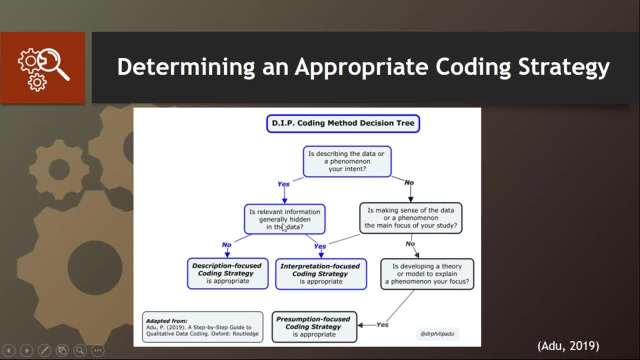 If yes, is relevant information generally hidden in the data? So this means that you have to go and review the data and see the kind of data that you have in terms of if you are looking for significant information to address your research question. do you have to make sense? 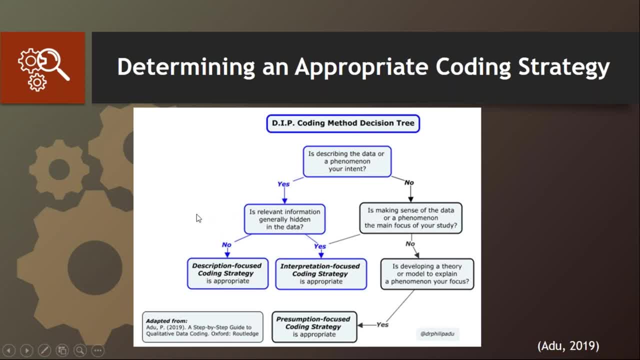 of the data threat. Do you have to ask yourself: what does this participant saying? What does it mean, Right Before you could make sense and address your research question? If that's the case, then, in terms of your research question, you have to make sense of the data threat. 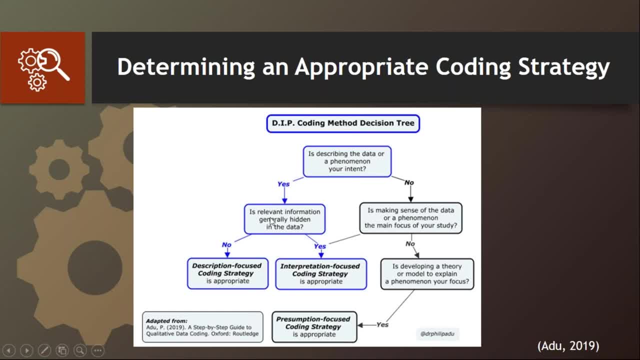 interpretation focus coding will be the best right. But if the information is not hidden, like the data that I showed to you, then description focus coding will be appropriate. The presumption focus coding normally is used when you want to explain a phenomenon or develop a theory. 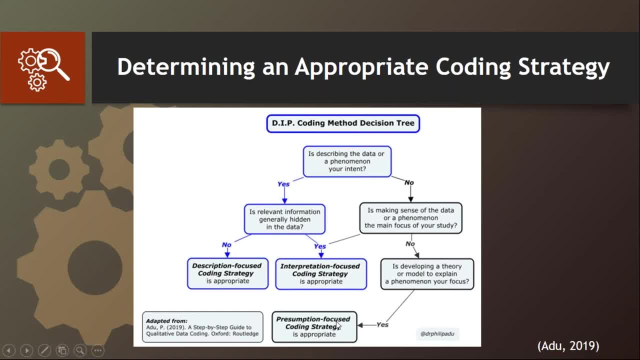 right, and that will be good for you, right. And besides these strategies, there are many, many others, right, so you don't have to use what I have here. They have thematic analysis, we have content analysis, right, so we have many types, you know. 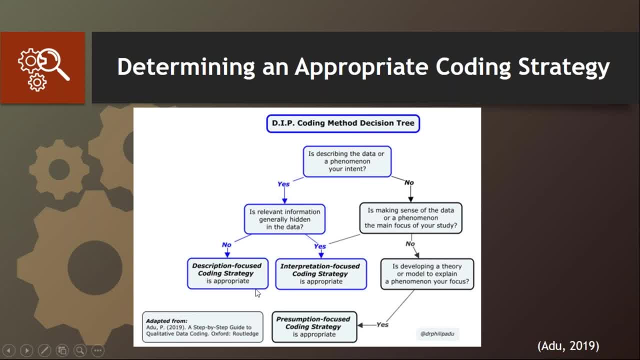 so if you think that maybe these are not really, it doesn't really fit, you know steady, you don't have to use it, But I think I tried as much as possible. you know, after reviewing a lot of approaches, I tried to come up with a simple way. 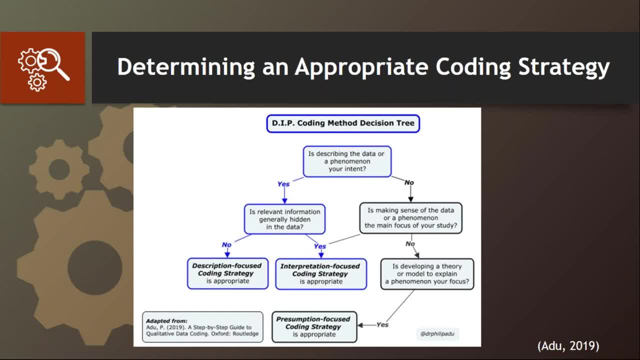 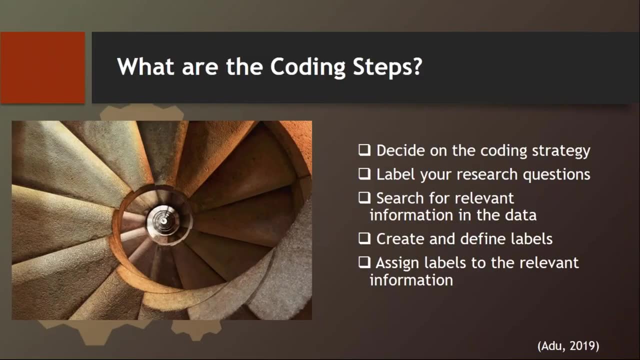 that will help you to address your research question that you have right. We have another question, Dr Du, from Danielle. She says: are the steps the same for the other two coding strategies? Oh, The other, oh, coding strategy. 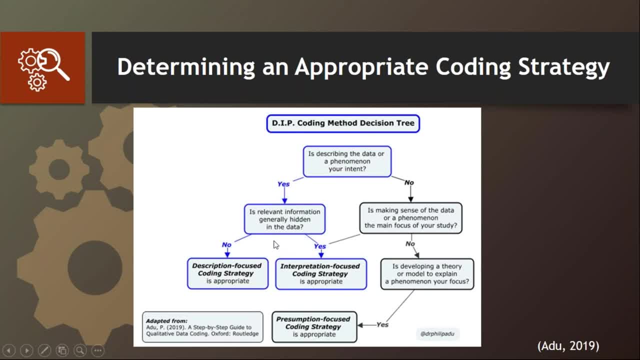 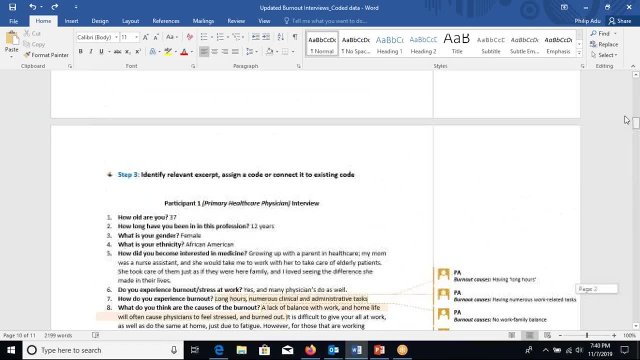 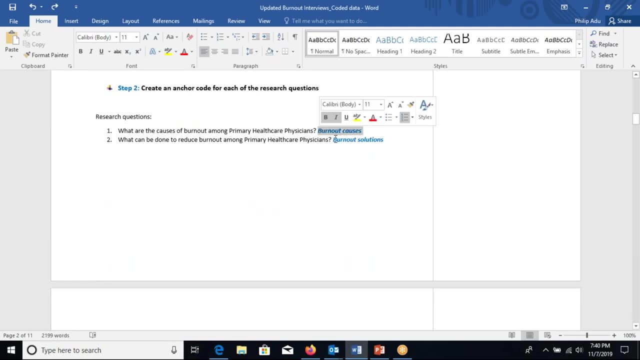 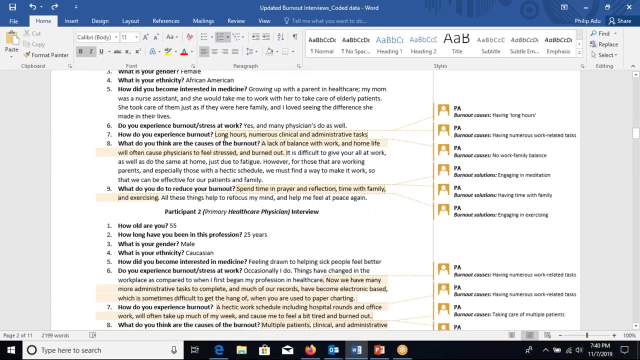 Yeah, they are similar because the same process of let me show you. So let's say, we chose interpretation-focused coding, right? So you're still gonna label your research question, right? And then when you are coding, when you identify the significant information. 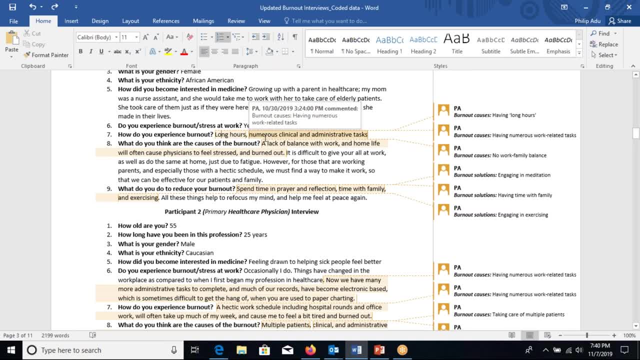 you have to do a couple of steps right. One step is ask yourself: what does this information mean? consider it okay, mean right. What does it mean If a person says that, say, make a comment about something. 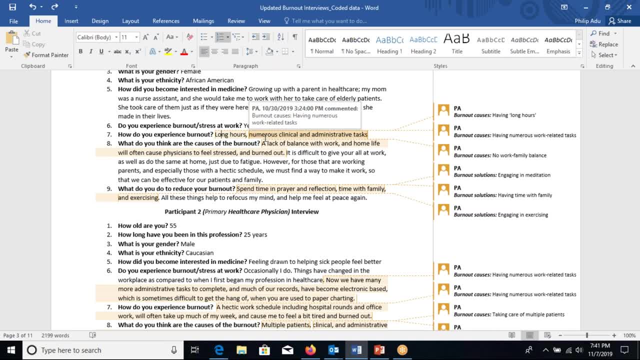 in order for you to understand a person, you also have to look at a person's background Right And a situation that a person finds himself. right If somebody says that today is my last meal. right If a person said today is my last meal. 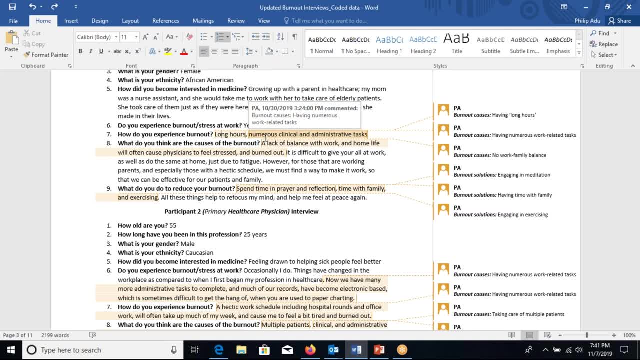 and you don't know the background of the person, the situation the person finds himself or herself, you might not really understand what the person is saying. He's saying Maybe this is the last meal for the day for the person right? Or maybe this is the last meal. 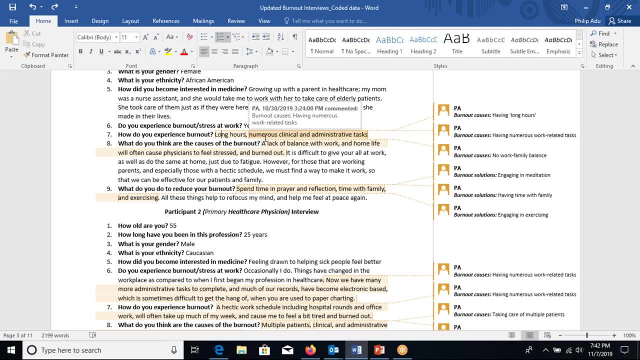 because the person doesn't have any money to buy any food at all. Maybe the person is homeless, right? So you see how one statement can mean different things when you take into consideration who was telling you that in the background of the person, Right? 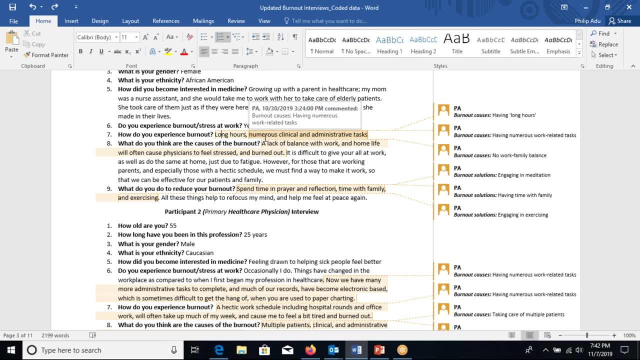 So, when it comes to this one, you have to first make sense of that, what the significant information, and then, after making sense, then you develop a code, a phrase to represent your understanding or your meaning of that information that you have identified. 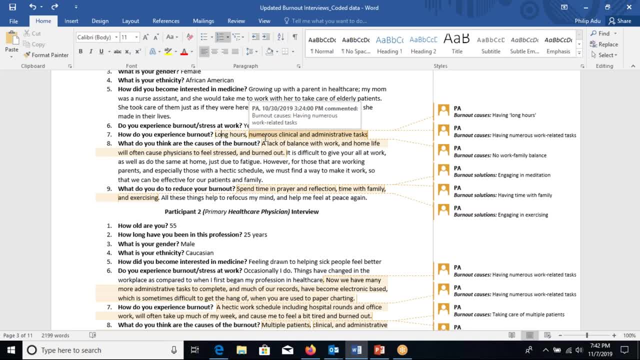 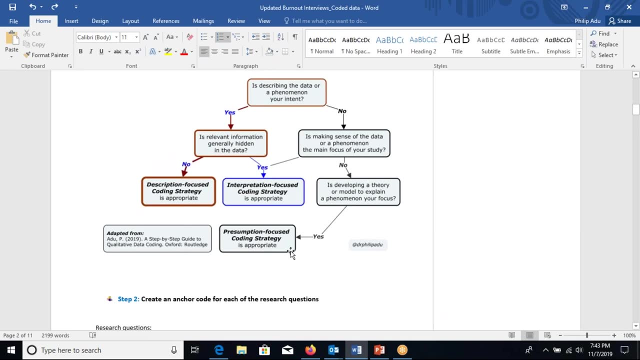 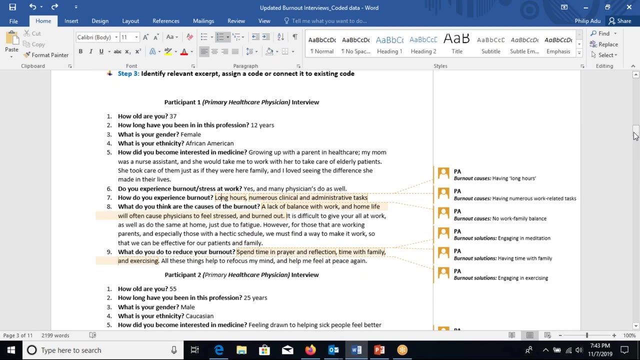 And so that code will be representing the significant information that you have identified. And for the presumption-focused coding you identify, first go through your data. look at the data as evidence. right, It's just the same thing as a lawyer. A lawyer makes claims about something. 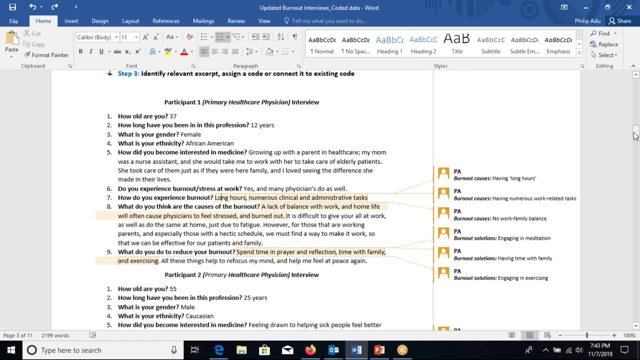 but before people, the claim can be convincing- convincing only if the lawyer shows evidence to support a claim. So you're going through the data, The data is. they are all evidence here, right. So you identify significant information as evidence and then, based on that, you make a conclusion. 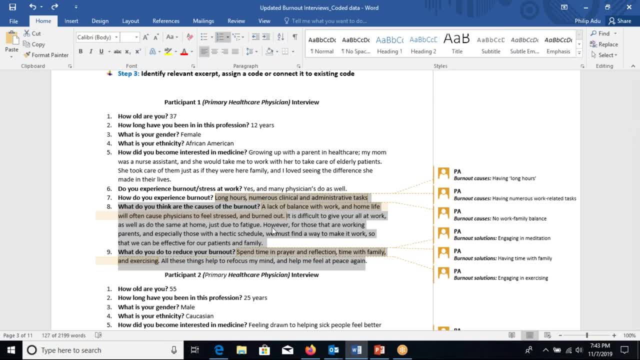 or because of this, maybe participant is hungry, or because of this information, maybe the participant needs help. right, You have make a conclusion based on what participant told you, so the conclusion will be a claim. that will be a code and the participant statement will be evidence that are that's connected to the claim. 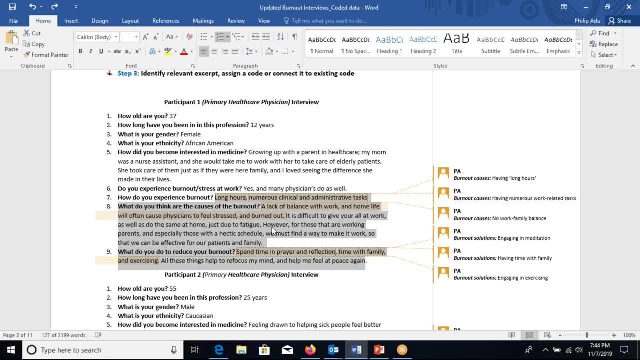 right and, and you know, in my book i explain, you know step by step how to do it. sometimes you have to use um, some labels that um there's. i don't have time to explain um in details. it's it's a little bit complex, but i think when you, you, you have time and go through uh, what i describe in. 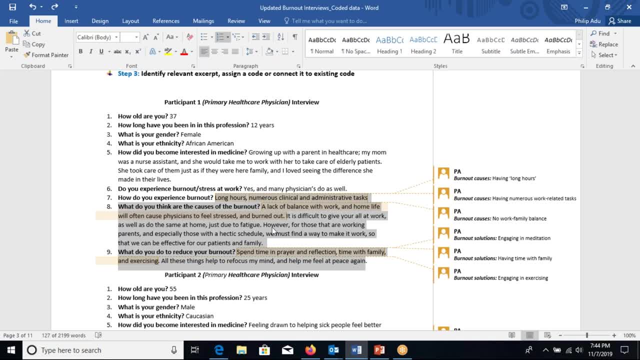 a book, you'll be able to understand the process. this, um the 10 level of coding, which is a little bit complex compared to the simple, uh, the simplest one, which is the descriptive description, focus coding. can i add something? dot, yes, yes, and this, and thank you so much for bringing this out. i know for 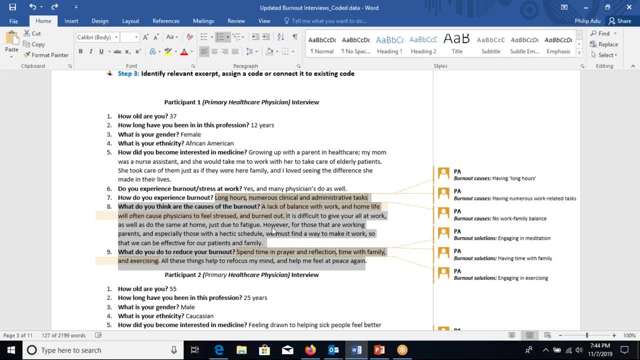 for some of, for some of them, they this may be deer in the headlights moment because of where they are with understanding this and even executing it, but i think this is a really important point to to hone in on because, in reviewing chapter four with students and working, 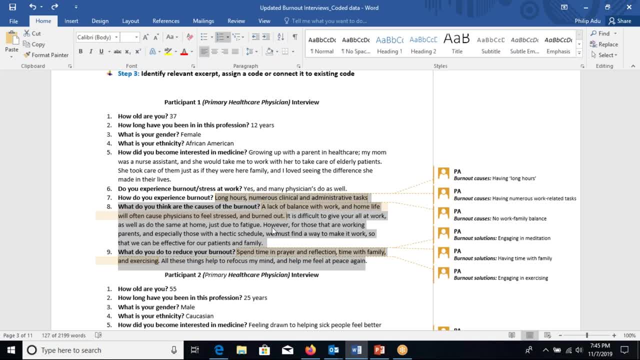 through the book process of coding and analysis and interpreting and then reporting, that there are often times- or not- when I say I can't follow the logic and what you're writing right, so there's a science behind this and the layers that, doctor, I do is talking about, from coding to categorizing and developing themes. 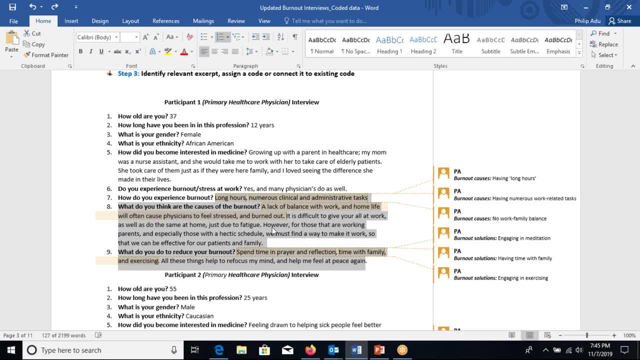 around that and providing evidence. sometimes, if you skip those steps in effort to get done quickly, or if you don't spend enough time doing one of those, it gets choppy, and so there's a disconnect between what you may have, as here's what you articulated as a theme, but I can't see how those layers cascade. 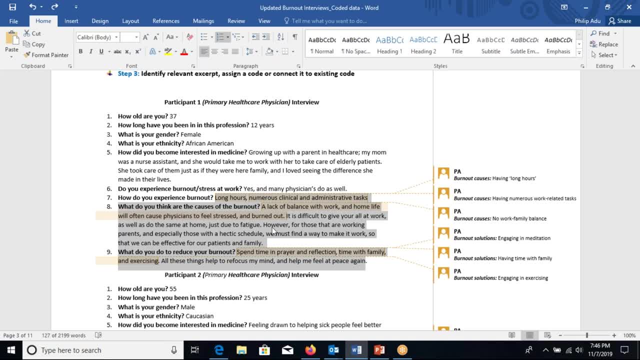 down into the codes, and so it it seems, I know, when we're looking at this for the first time, sometimes it seems sort of high level and you might even interpret as: oh, that seems pretty easy. now, no doubt it, there's. there are some points in the code that are very, you know, very simple and very easy to take. 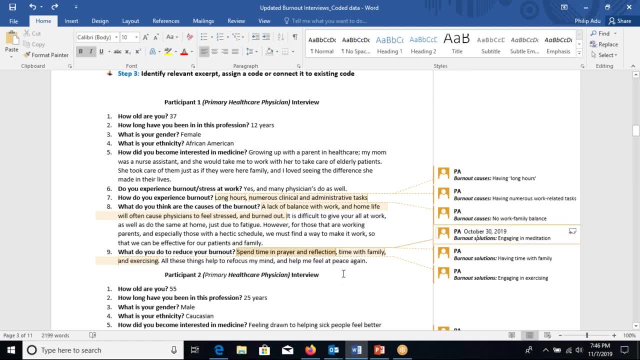 parts of this that are relatively simple to execute and understand, but the level of interpretation and analysis that he's speaking of really takes some time, and that's where your scholarship comes in, That's when your work in becoming a PhD and developing all this stuff and these competencies- 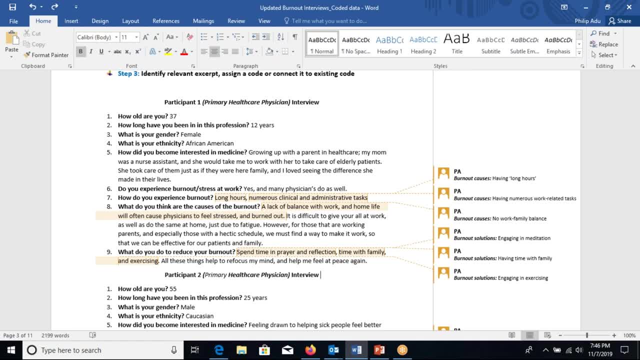 over your time in this program. this is where it comes to bear, And I always say that qualitative analysis is a skill that you have to develop right And upon me writing a book on this. I'm not perfect in developing goals and coming up. 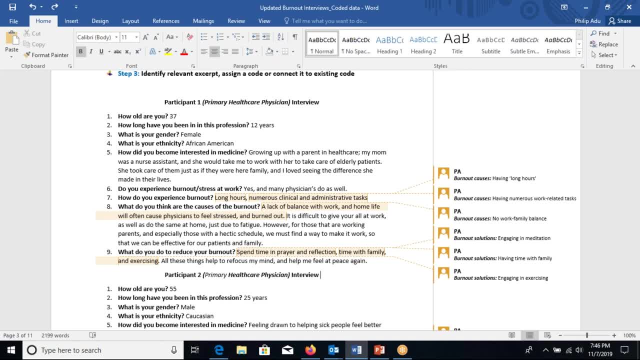 with themes, right, But the most important is the more you do, the more you become better and the more you become confident about what you do. right. So it's a process. you just there's nothing like a perfect code. 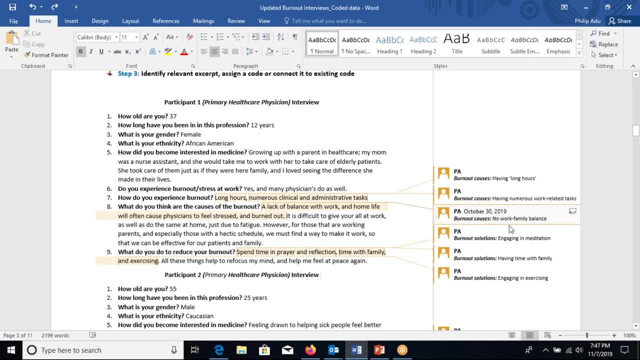 The reason why there's nothing like a perfect code is that that's why you have to define the code, right? So if you say having time with family, somebody might interpret it in a different way, right? Or it doesn't really perfectly represent the significant information. 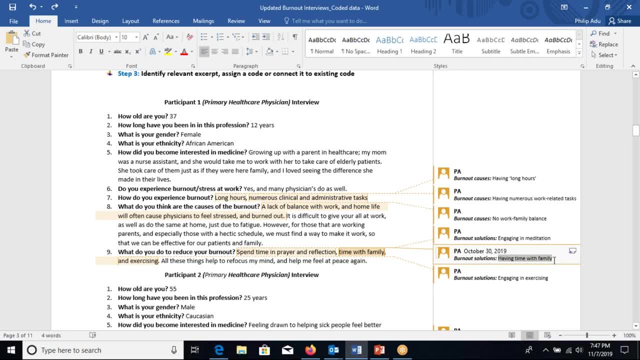 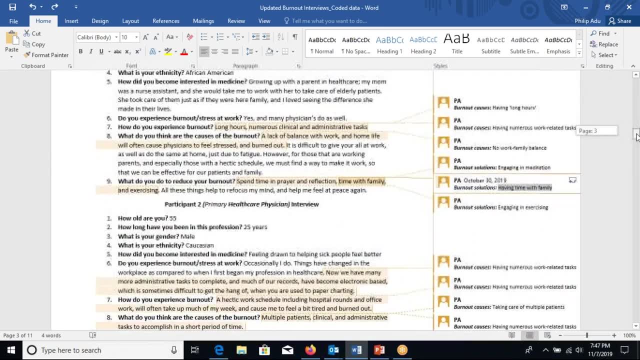 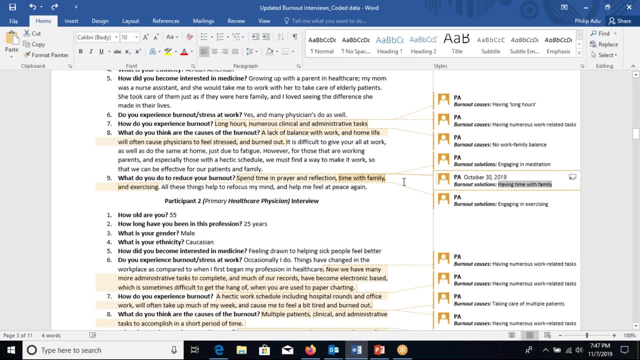 That's why it's always important to define your code And also you have to be able to define your code, So be flexible. Sometimes what happens is that as you are coding, you realize that, oh, I think engaging and having time with family doesn't really best represent this information. 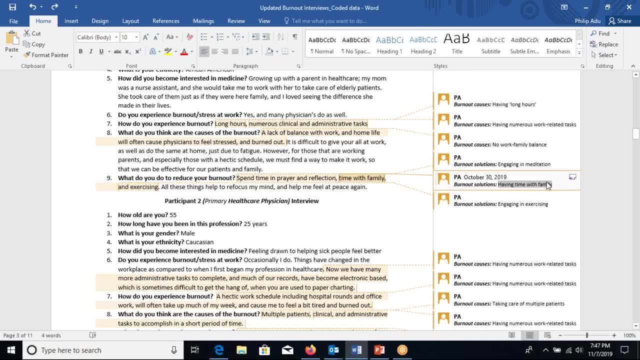 So let me change it. Yes, you can change it. right, You should be flexible, can go back and change the code if you think that you have a better one. to represent, As you are going through the data, you understand it more. 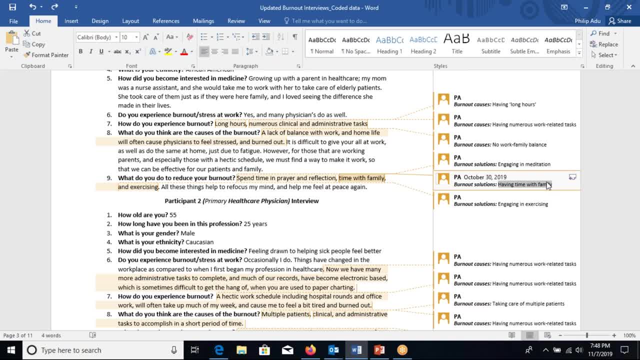 So, when you understand it, you can go back and make changes. So that's why it's important to be flexible. Okay, So there's always going to be flexibility, but, as Dr Morris said, you always have to make sure that you are following a systematic process, because that's the only way people 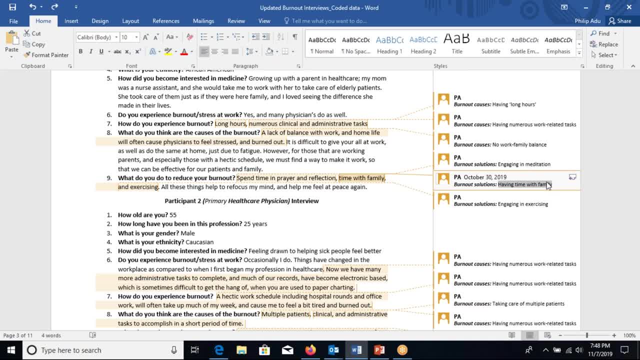 will trust what you found. Coding is a subjective experience. You are, you and your data right participate when readers were not there or your audience were not there when you are doing the coding, So you have to be able to document the process so that you can explain to them how you move. 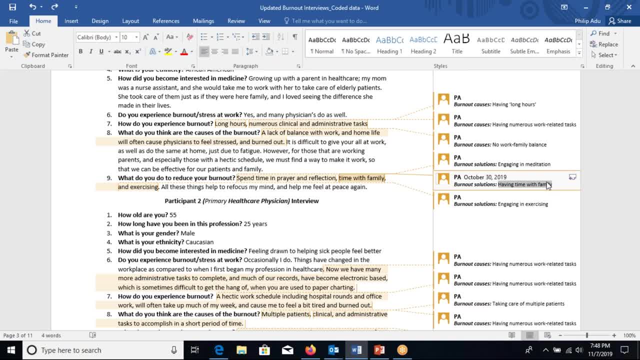 from identifying significant information into developing codes. how you move from developing codes into developing themes so that they will believe what you found right. So it's all about documenting. it's all about being systematic and you'll be. it's all about perfecting the process. 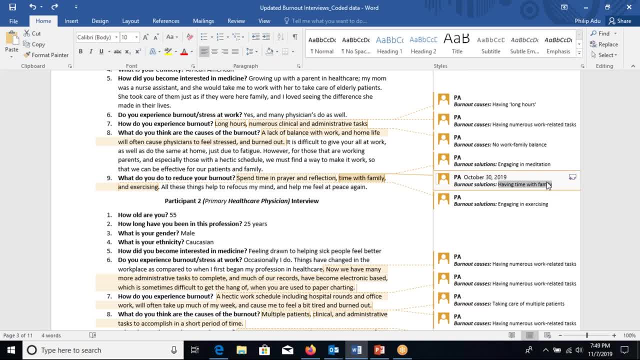 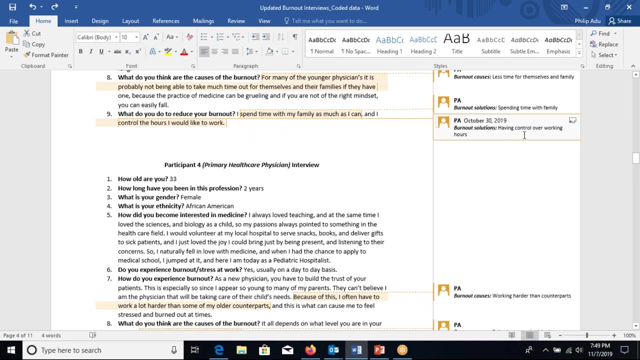 It's a skill that you know needs to be developed, and you, you are not going to be perfect the first time, And I'm me personally- I'm always learning, learning how to code better, right. So what you have here, I have here, may not be perfect, right, but the flexibility for 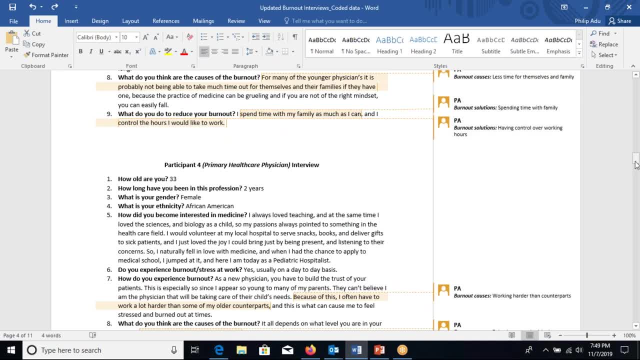 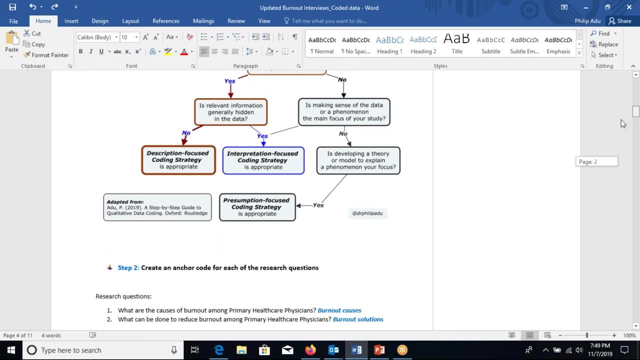 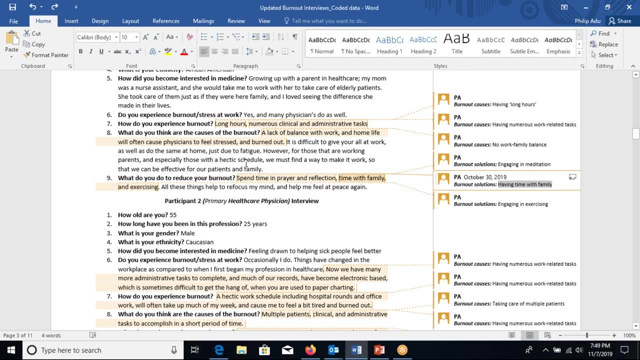 me to go back and reflect- Okay, I can even change my mind- that oh, I think descriptive coding description coding wasn't. I wasn't able to get a lot of information using description description focused coding, because I was just describing. 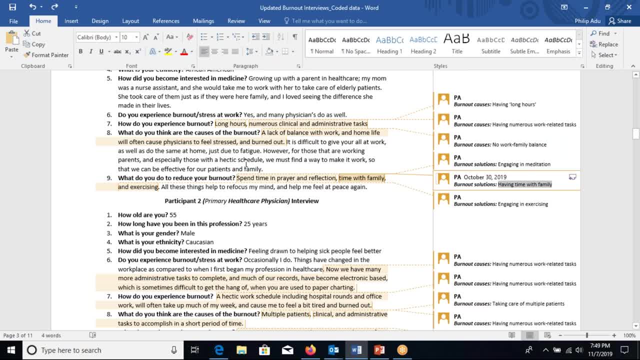 What about moving into interpretation, Making sense? Will I, will I get something from it? if the person say that a lack of balance with work and home No Life would, will often costs physicians to feel stress, Master the game? who we? who is talking here? 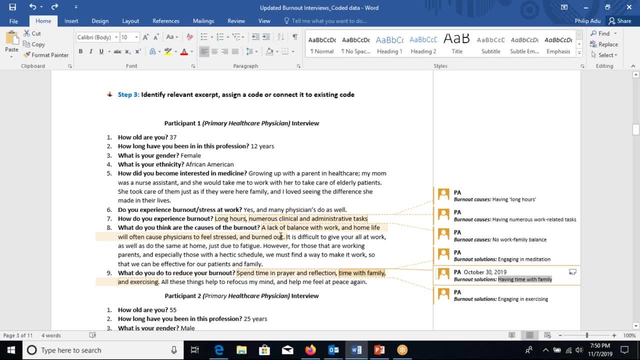 Let me look at a person's background, right, Can I? can I get additional information from what the person is saying? the person is 27,. the person has 12 years experience. Maybe the person's a female. my person is African-American. 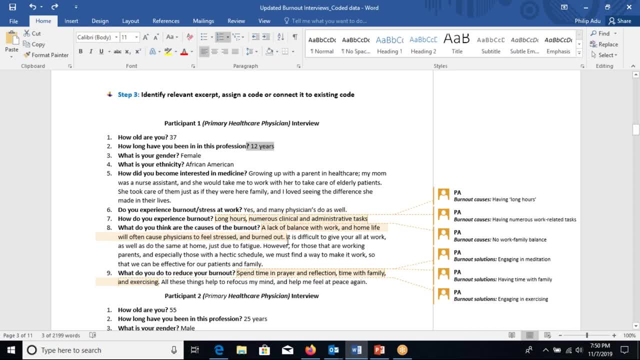 Can I? can this background information help me to understand what a person is saying? Oh, let's cycle it. Well, the question is from Another Care Dominant. Okay, right, so sometimes maybe you will start with description focused coding, but you can change. 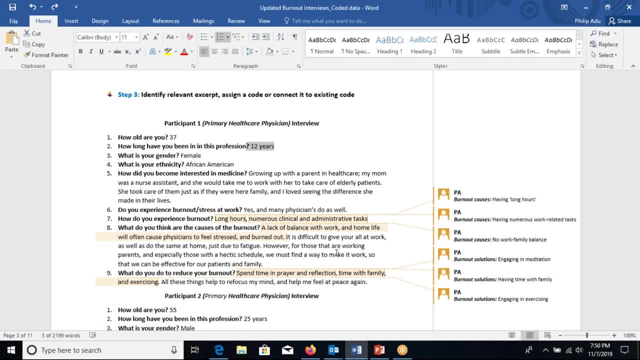 to interpretation focused code and most important thing is to have rationale behind. why have you changed? is you know you have to be flexible. at the beginning you realize that maybe this descriptive was the best, but you realize that you are not getting enough information to address a research question. so let me. there's some hidden information there that descriptive will not help. 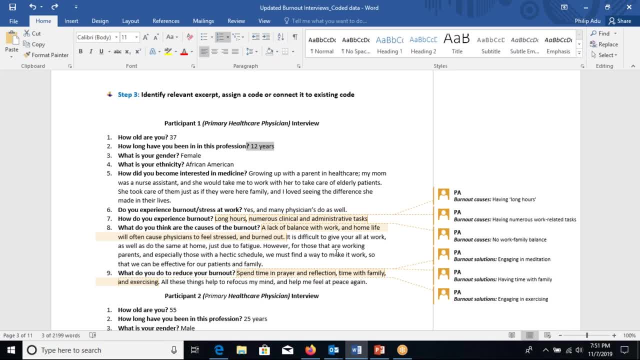 me to get them to my destination. so I go to interpretation, focus coding, and you can even use both. some I've seen some studies where they start with descriptive and then they go into interpretation right, so it's all about being systematic and they're also having rationale when people ask you. 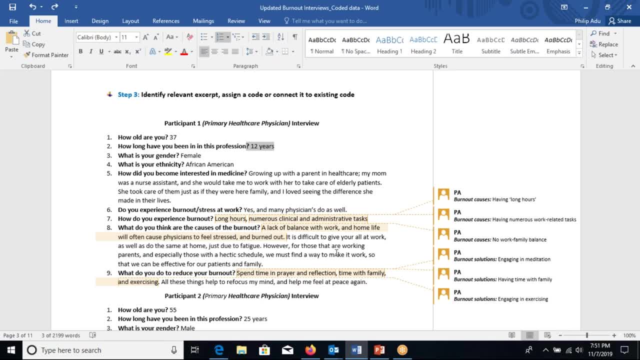 why are you not using presumption focus coding? what would be your answer? it's all about justifying your actions. right, I'm gonna. can I add something to that, doctor? obvious, particularly about the systematic about it which is really important. and so there are multiple times and I serve. 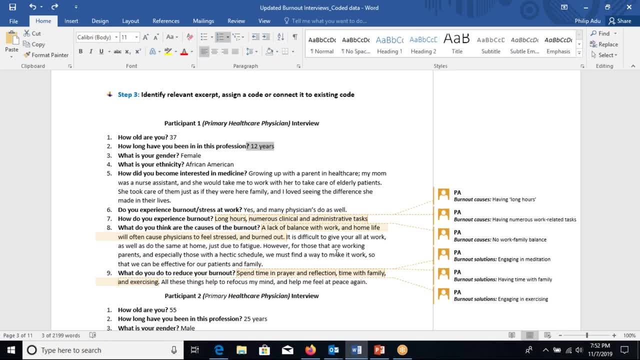 on-campus committees for students for whom I don't chair, and so I don't necessarily work with them closely on the analysis. but when I read the document- and this is, this is not just for me, but this is for everyone- even in just publishing your, your work, with your dissertation, we people should be able. 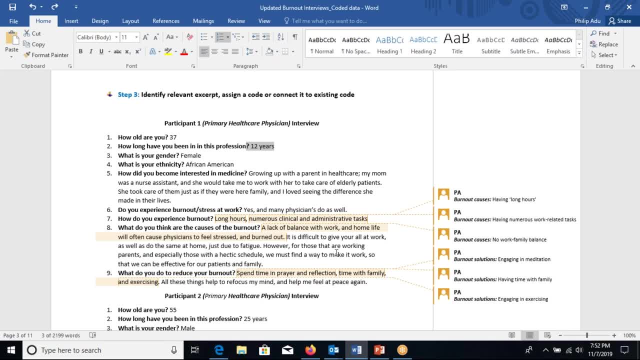 to ask you, show me the documentation, so show me the system that you created. and so I've asked students in the past: export your code system to me so I can see it. send me your, your, your code system to me so I can see it. send me your, your code system to me so I can see it. send me your, your. 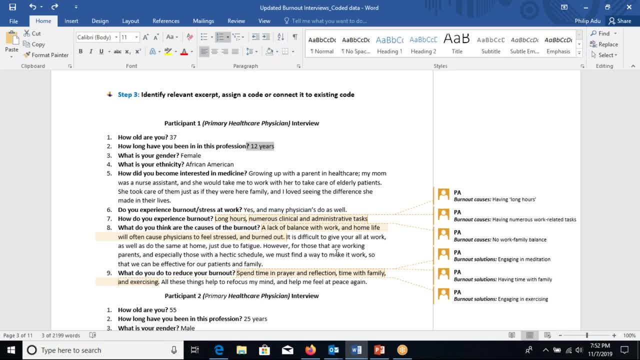 your summary tables so I can see what you wrote to help me understand how you got to this. and- and part of what doctor I do is describing this- is sometimes it takes a while to sort of massage it and having conversations with others and even continue to look at the data and I can. 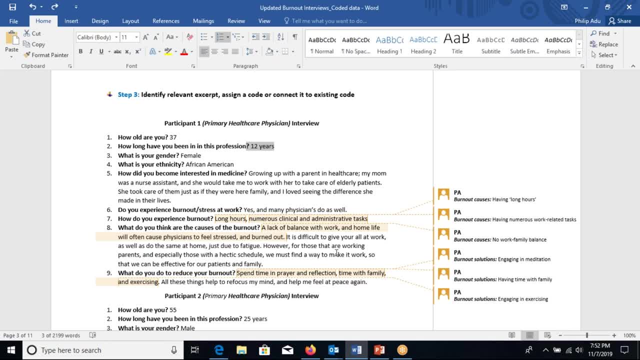 tell you, just today, with a student with whom I'm working, I I gave feedback. today I'm looking at on my screen that says I'm not yet convinced that the ideas articulated are fully aligned with the data you collected. Yes, the things you're describing so far were experience, but I'm not. 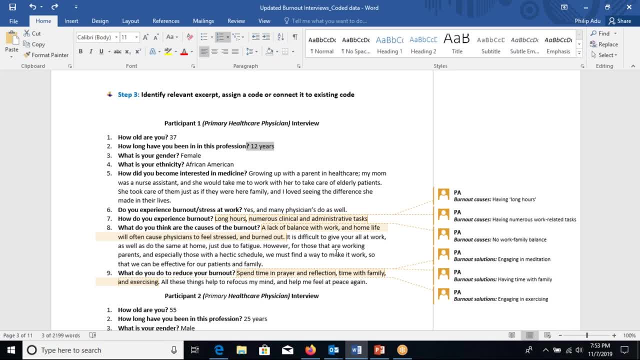 sure they're at the theme level. My concern is that, after reading earlier drafts of this, it seems there were many more positive experiences expressed by participants than you currently have in the theme presentation. right, So it's? show me the system, show me the evidence that he mentioned. 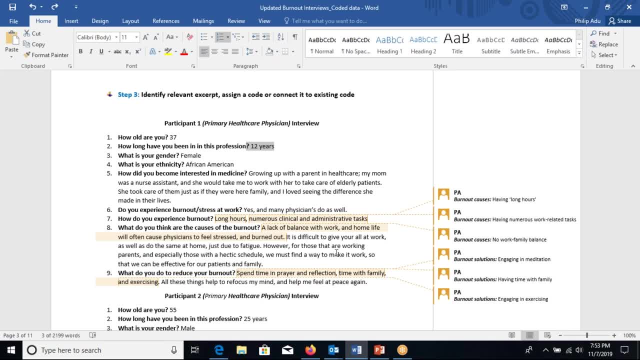 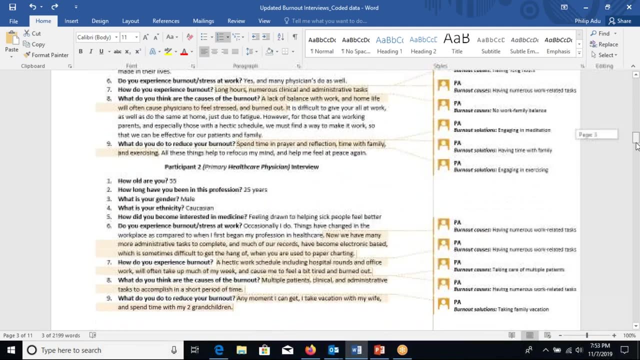 and now let me follow the science of how you put that together. So it's complex, it's layered, it is a skill that you develop, learning to be a qualitative researcher. It's so true, so true. That's the only way people believe what you found being able to demonstrate. 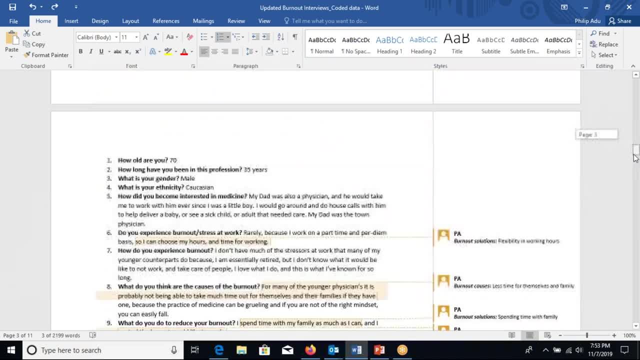 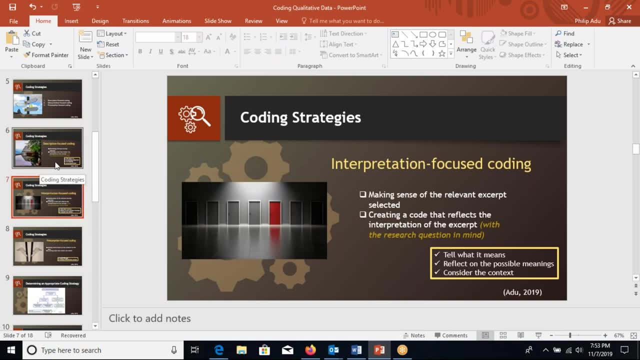 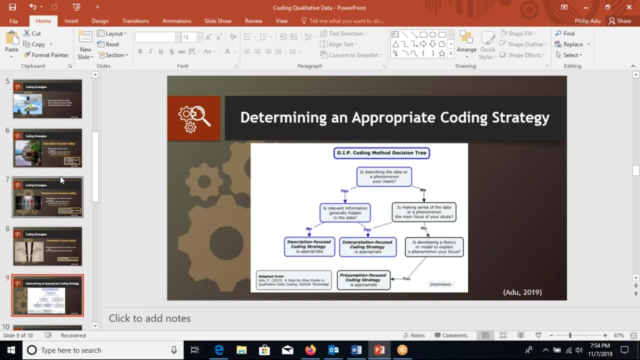 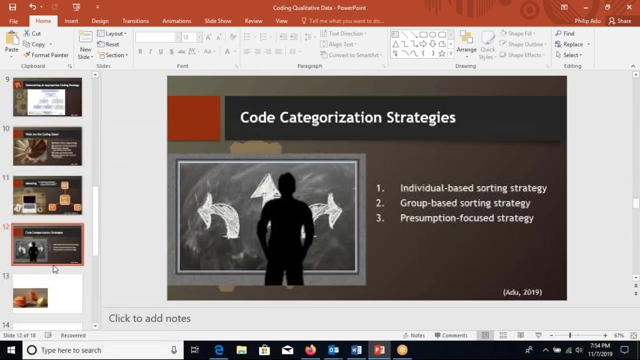 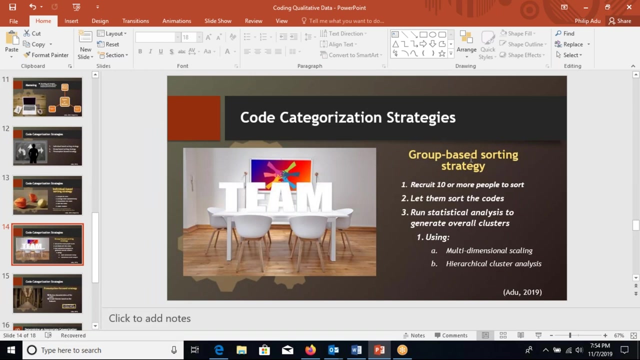 how you arrive at the themes That you have. So let me briefly touch on the second and the third categorization strategies, and then we can end this presentation. Let me see here: So group-based sorting strategy is more about. you know, this is where you're going to be able to. 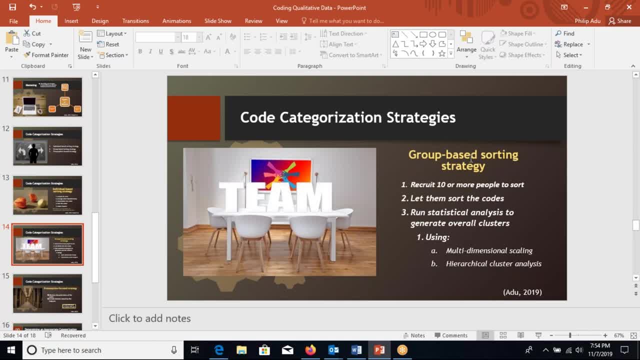 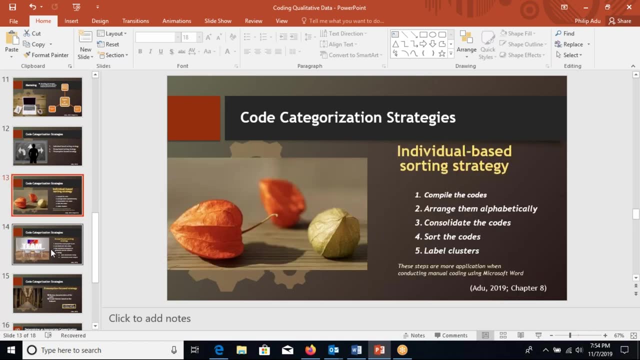 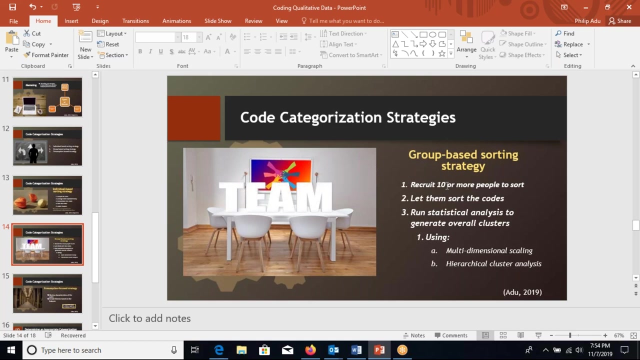 where you may have to use a quantitative approach to come up with the themes or the clusters, right. So you see how you did it. I demonstrated you doing it as individual. This one- you are involving people. So if let's say you have, you can involve participants to do the sorting, especially if you 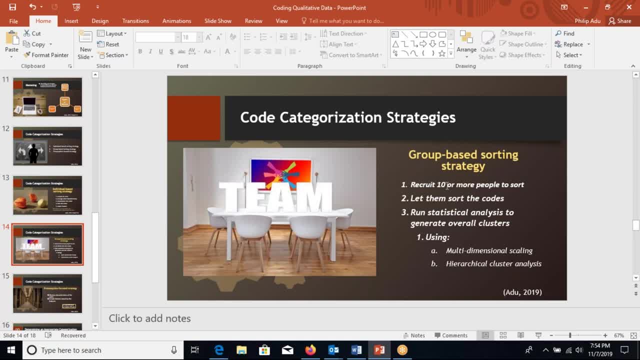 are doing a descriptive, Description-focused coding where you have summarized, technically, you have summarized participant responses. You can give it the summary to them in terms of the course and let them sort it, group them for you, right, So you can. if you have a group of 10 or more, you can let them do it. Another one is: let's say you want: 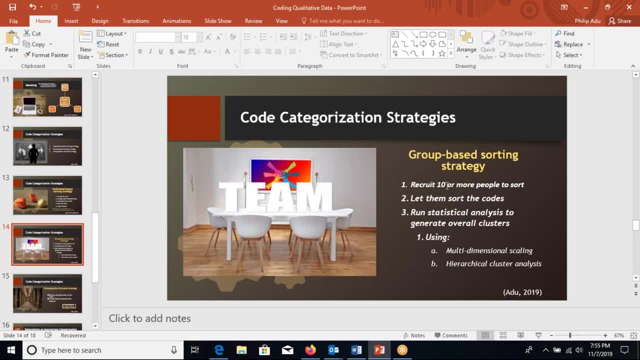 to involve professionals, right, Maybe mental health workers or mental health clinicians- to review the codes that are related to maybe their work, right? And then you tell them just to categorize the code for you and then they bring it back to you. 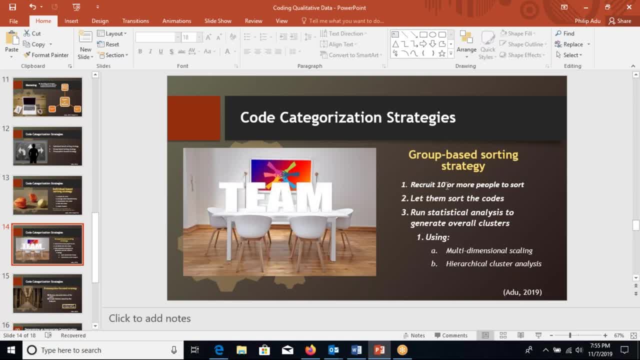 And so when you give it to them and they bring it back to you, right, You put it in an SVSS and run an analysis, And then you'll be able to categorize my request right, And if they cans, the most accomplices. so do you want me to take an individual größer question? 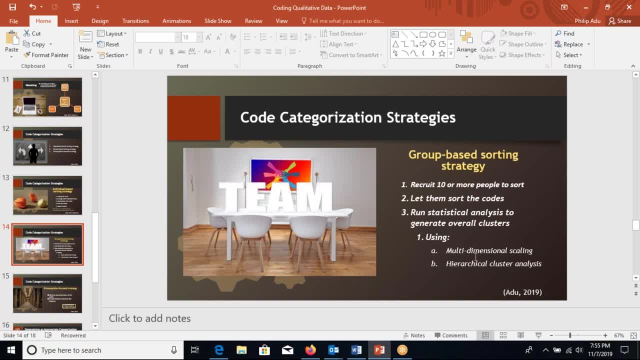 about that question Because I have that key question. Yeah, So first of all, if you think like a social improvements, incentive, development, how well can I do this? You can. you only need the subsequent questions. come up with clusters And in my book I talk about how to do it. You're going to do two main 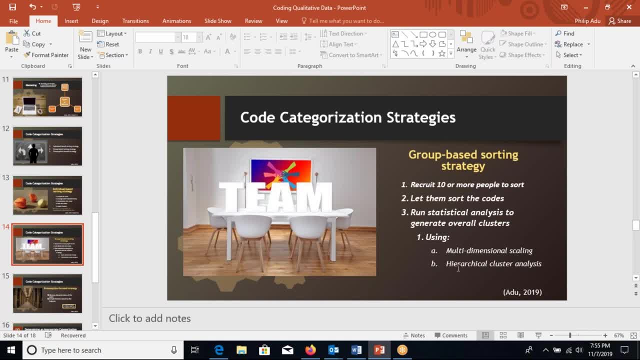 analysis, multidimensional scaling and also hierarchical cluster analysis, And at the end of the day, you come up with clusters similar to what you have. I did it manually here, but the system will help you to come up with clusters And those clusters will be the teams right. 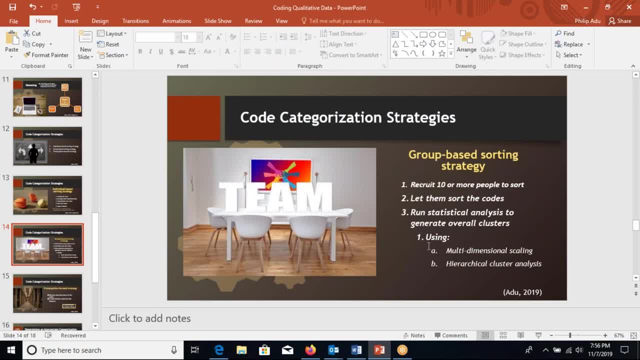 And that will help you to address your research question And, as I said, I provide detailed information in my book if you're interested. Normally you do this when maybe you are doing a participatory action research and you want to involve participant or you involve stakeholders. 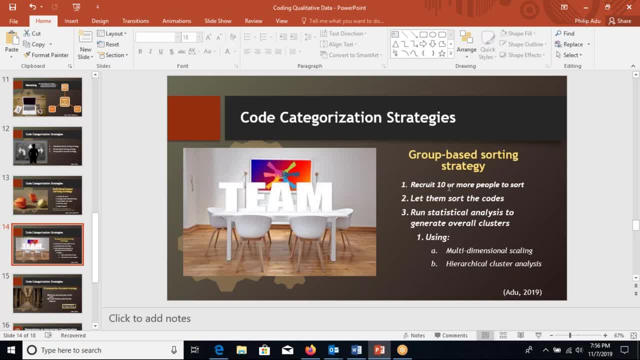 in maybe solving a problem or implementing something. you can involve them and use this kind of method, That's the group-based sorting. This means that you allow them to sort it right Instead of you doing it yourself. you allow them to sort it, They bring that information to you and you use SPSS. 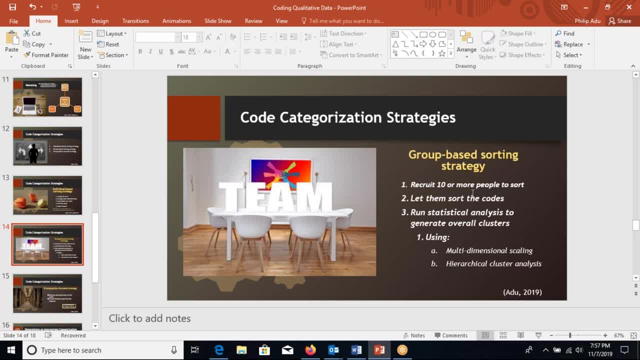 or any statistical analysis software to come up with clusters that represent individual categorization, All the clusters that individual participants have done right. So that's all about the group base. If you are doing it individually, you don't have to use this one, but if you want to involve, 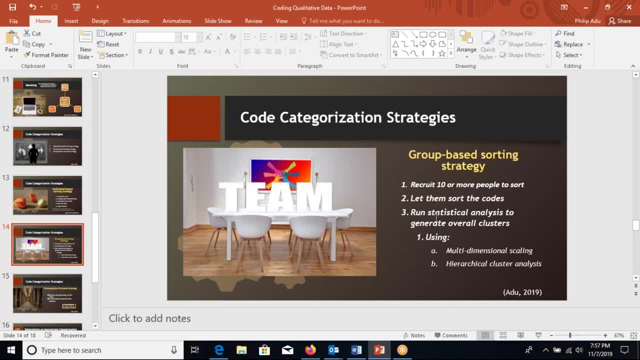 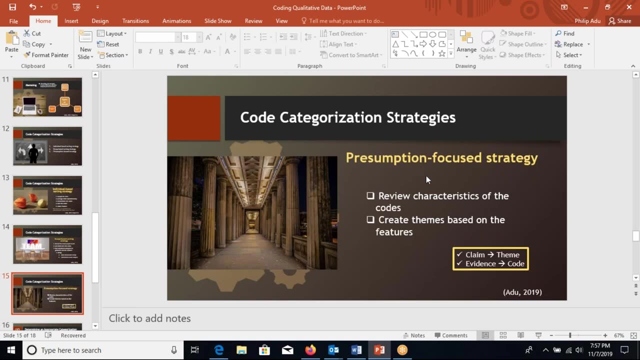 stakeholders, participants, professionals and maybe colleagues in coming up with themes, then you can use this kind of approach. And the last one is the presumption-focused strategy. It's quite similar to the one that I talk about in the coding level. So this one, what you are doing is that now the codes that you 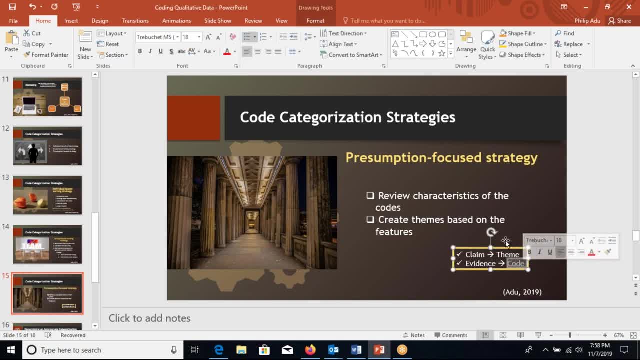 have come up with will be the evidence right. So you look at the codes, you review the codes and then you come up with claims or fees And then you connect the code to the claim that you have come up with. So, as I said, the codes that you have come, 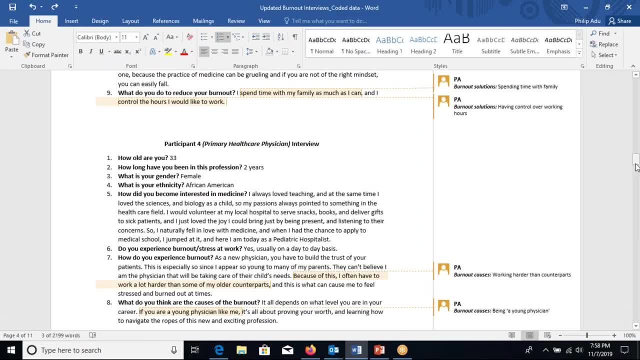 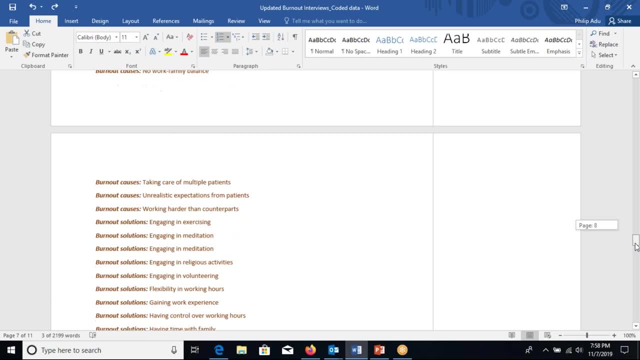 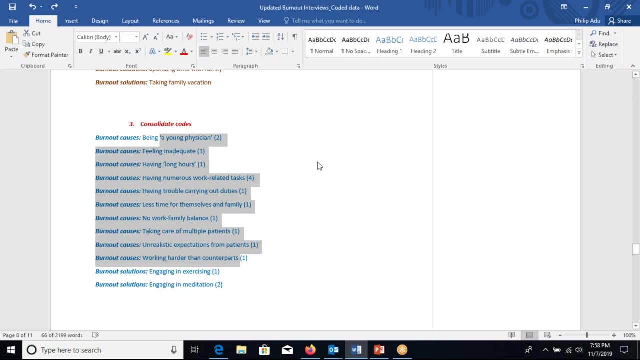 up with. So let's assume that you are using presumption strategy for categorization here. So these will be evidence, right? So you go through the evidence and then you come up with themes, And then you connect the themes to these evidence. right At the end of the day, you have 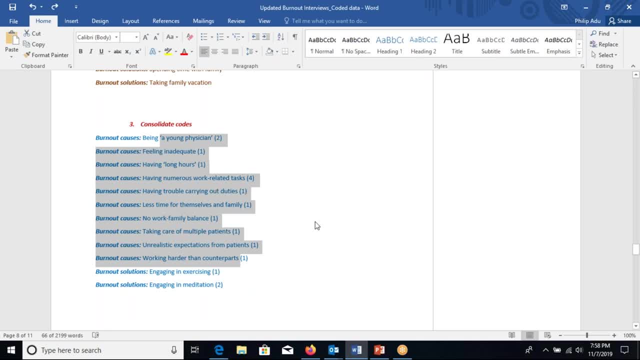 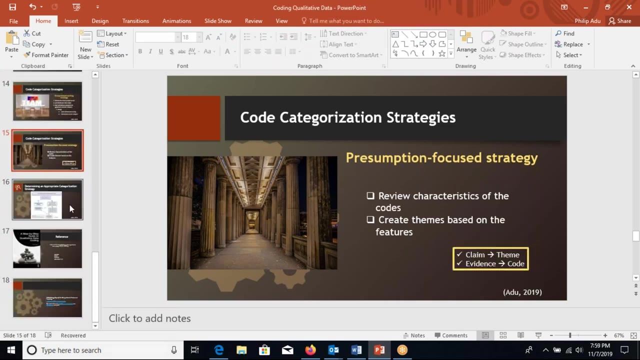 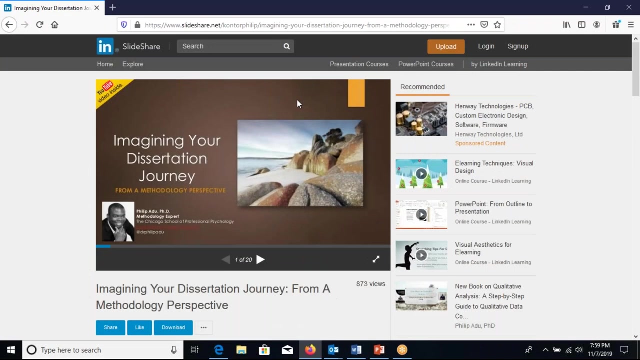 you know a few themes and then a couple of evidence connected to the themes, right? So for this strategy, these are evidence and the themes are claims. okay, So that's all that I have for you. If you want to get access to my book, you can go to Amazon and 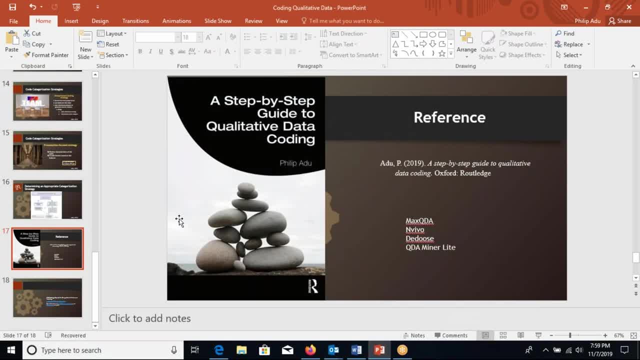 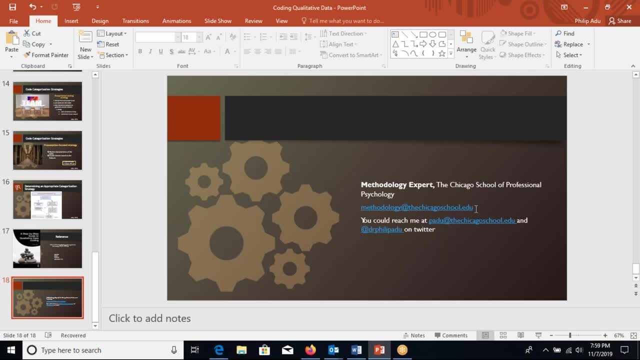 then search my name and you'll be in front of the page and you'll be able to to it. If you want to ask to meet and have a discussion about your methodology, especially when you are doing your dissertation, you can email methodology at thechicagoschooledu. 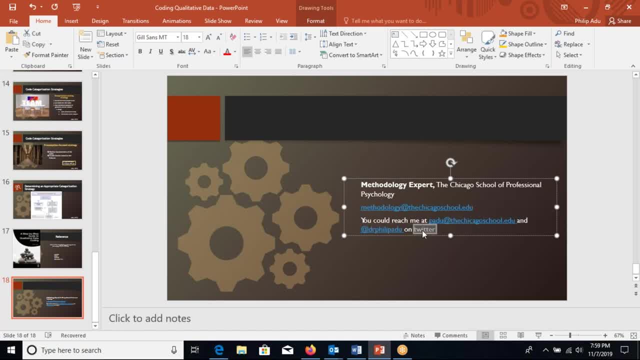 or you can email me personally or you can follow me on Twitter or you can add me as your LinkedIn connection colleague, And what I do in LinkedIn is I provide a lot of information about methodology- articles that I see I found interesting and informative, and I share information. 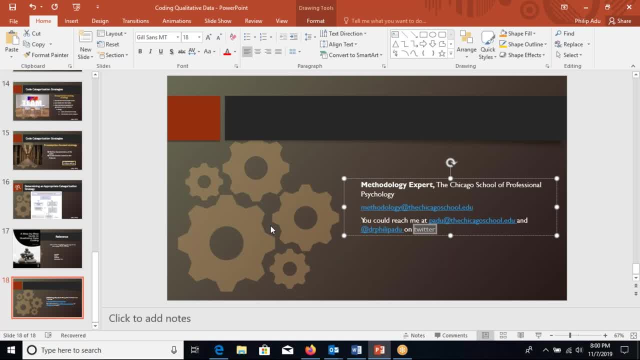 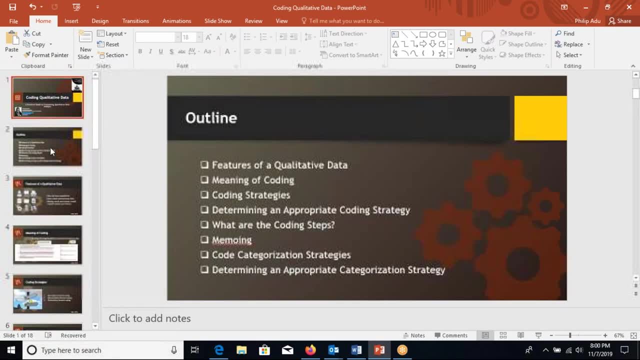 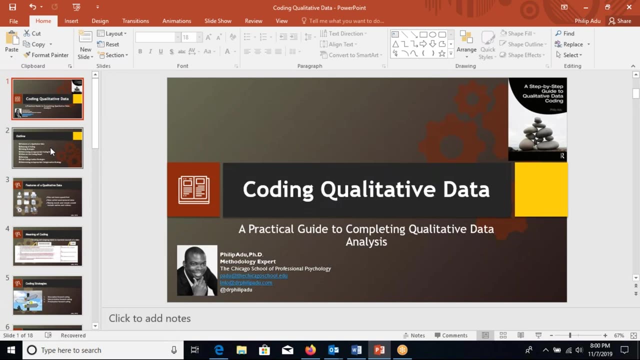 to my followers, So you can also follow me on LinkedIn. So this is what I have for you. I don't know whether you have questions for me, I'll be happy to address them for you, Or if you want to ask me about what we do as. 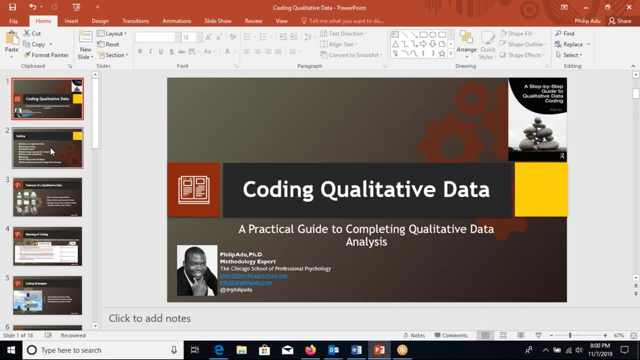 methodology experts and what kind of support we provide to students. you can ask and I'll be happy to address Any questions. Okay, Okay, I don't have any. That was pretty straightforward. Thank you, Sarah, Appreciate it. And you told I think I might have missed something. You told us where we 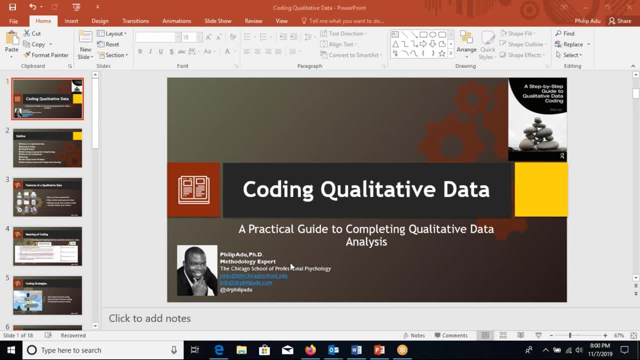 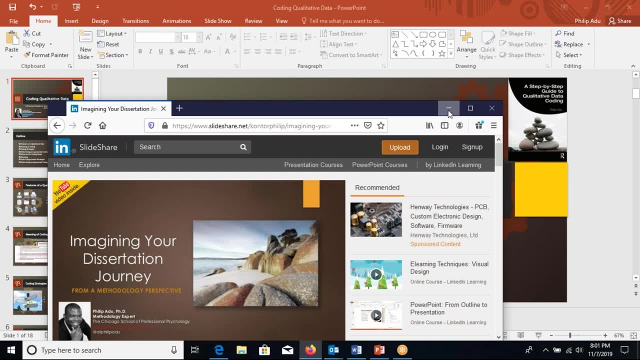 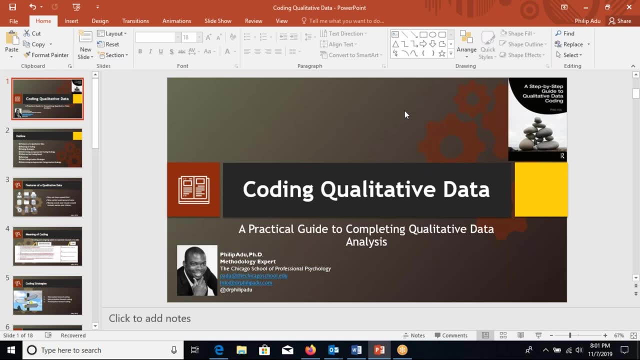 can get your book. Yes, I want to go to Amazon, Okay, And you type my name, Philip Edu, and the book will pull up. All right, Okay, Thank you, Thank you. Thank you, Hi. I have a question, But before, thank you so much for taking this opportunity to come. 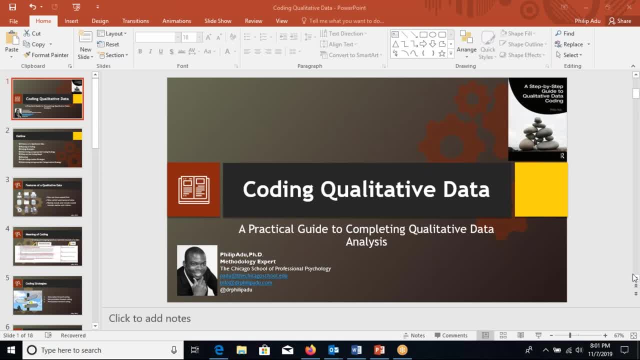 on and show us about cutting. You're welcome. I personally need very much help in cutting. This is all new for me And I appreciate it. yes, my question is: well, I was a little bit late. maybe you talk about that, but when will I know, or how will I know, the best coding software to use, or? yes, okay, 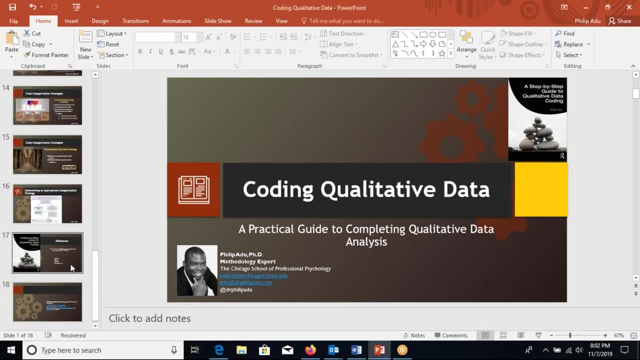 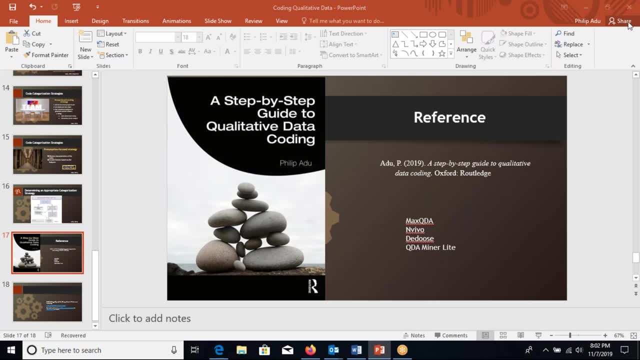 so in terms of the best it is, it depends on the student. I can tell you what a lot of student use a lot of feeling. you use mass QDA and in vivo deduce and QDA minor light. most of my presentations I use in vivo. I have a lot of presentation. even my book I use in vivo and also max QDA is very good I have. 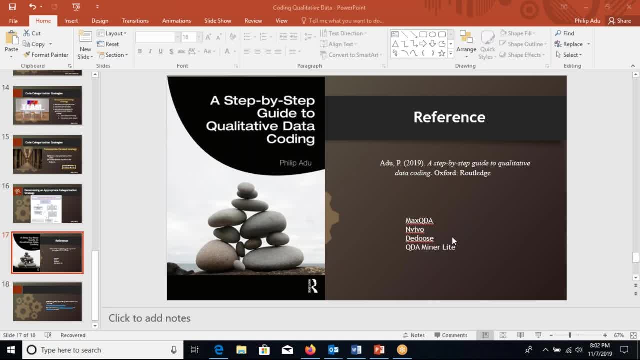 a presentation also on QDA minor light. so what I always tell students is that first of all go to YouTube and type the software that you are interested in and see whether you can get videos when you review some other videos and you are clear about a process and it's user-friendly. 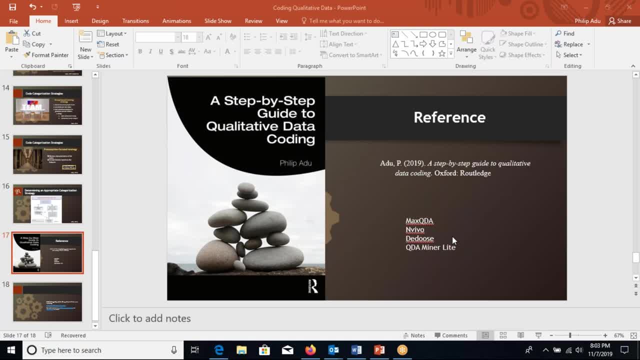 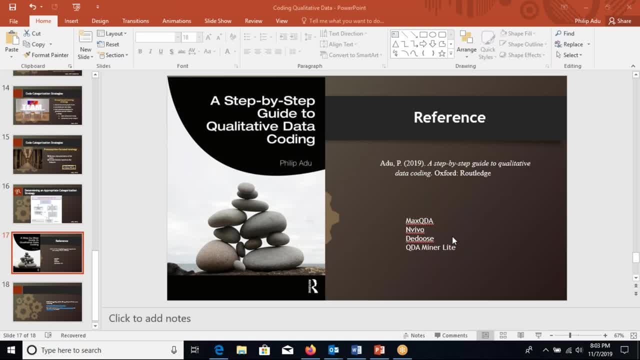 but me personally. the one that I use is in vivo but, as I said, mass QDA is also very good for the But the D seminar, but it was a lot better than I was used to. three you can download what I like about did uses that you don't have to download anything into your onto your 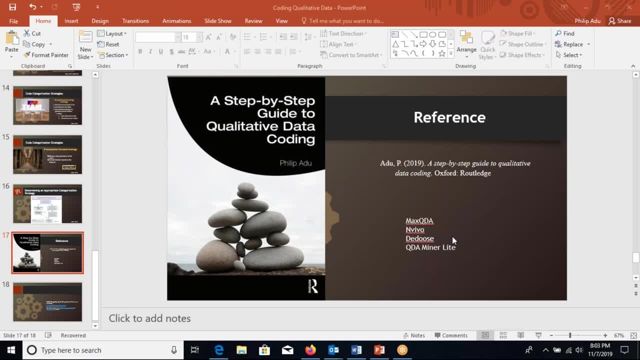 computer and you can do everything online, right, so you can upload your information online, your date online online and analyze it. You just have to log on. Then, when you finish, you can support and information. four, deduce and qda minor. in my book i wanted to cover a lot of um, all kind of students. there are people. 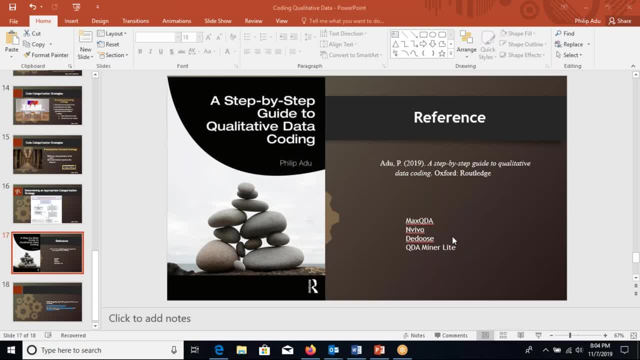 who cannot afford to buy a software. so i use qda, minor light- and i have a presentation on that- for people who don't um don't have um money to buy. and there are some people who don't want to download anything on their computer. they want to do it online. right, i demonstrate how to use deduce. 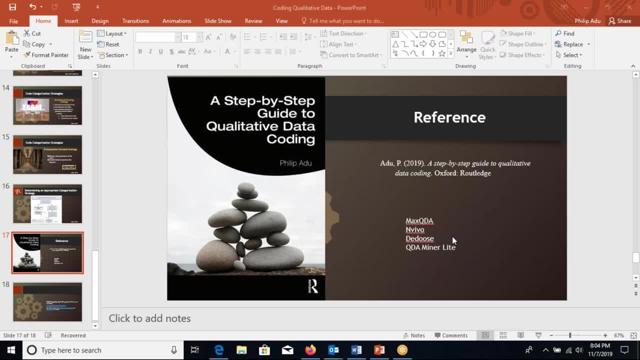 and most of the students i work with use in vivo and that's why i i also use in vivo in my book. um, and i didn't use qda minor i i masked qda because it's quite similar to in vivo and so um. so that's why i didn't use, but it's also a very good. 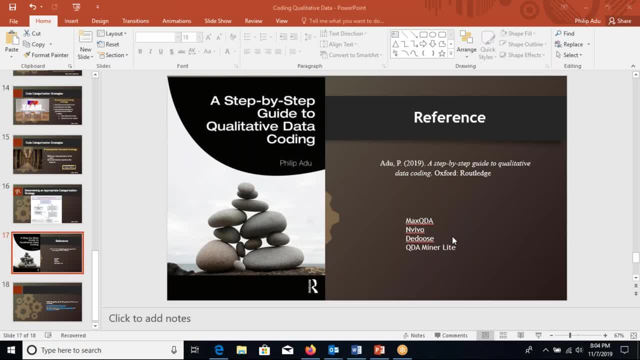 software. yeah, and let me. and let me add something i think is important in considering which software to use. uh, i always encourage students to use something that someone on your committee knows, so that that helps reduce the learning curve for you, and so i use max most of the time i have used. 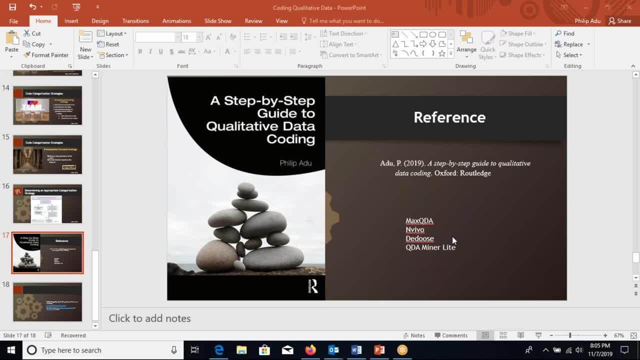 deduced, and so when i'm working with students, i always encourage: say, pick one of those, because i can help you, because i know that i i understand in vivo, because most of it, as you can tell from what you showed us, we know what the output should be, and so the nomenclature within the system might. 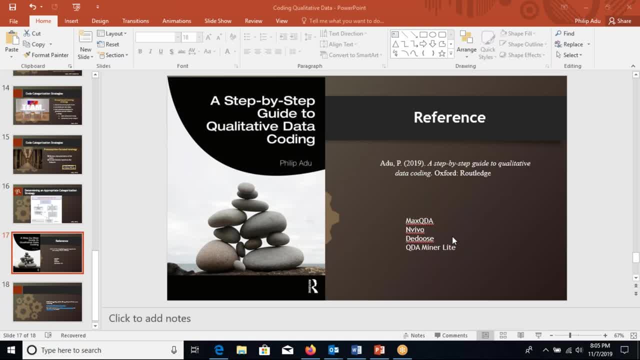 be different. the, the direct function might be slightly different, but we know how to navigate to what you, what we need to see there. so i would say: trust the people that are closest to you and supporting you in the process, and so if you've got someone who says, hey, i know in vivo, i use 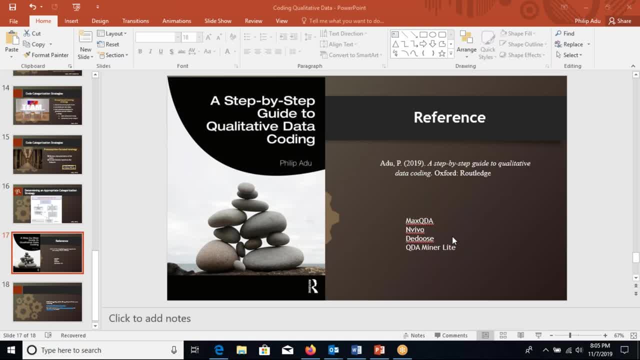 that all the time. you're probably best served with that because they can help you through the hurdles you might have in trying to understand it on your own. i completely agree. yes, i, i appreciate that, but my question uh goes more intense because there are some softwares that they are friendlier than. 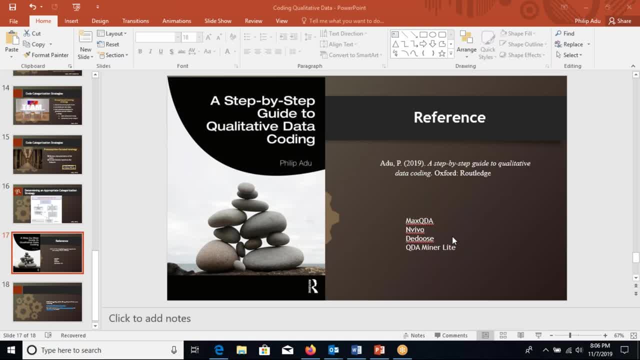 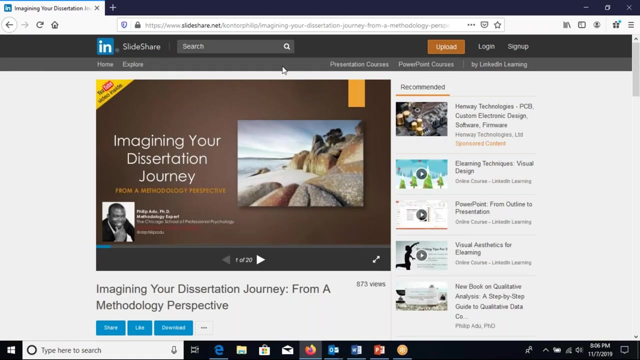 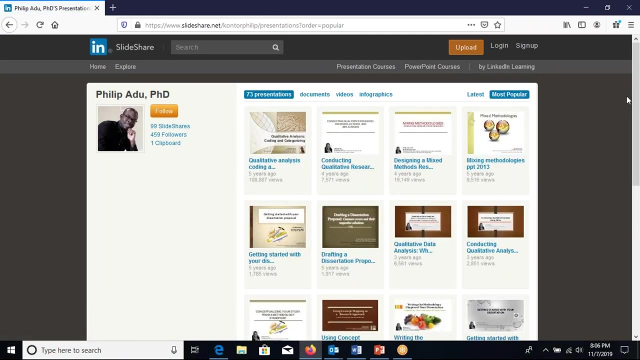 the other one, especially for those ones that does nothing. that is just about it and that was my question even. it's just like uh, first level, um just how to learn the basic foundations, like because, um, some softwares they are so pretty, pretty complex. so my my question basically: uh was in in that scenario, okay, so for me, 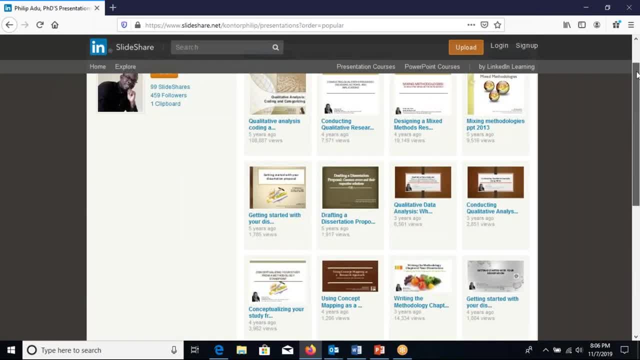 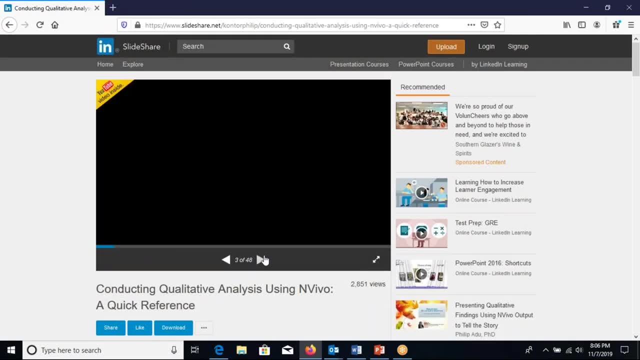 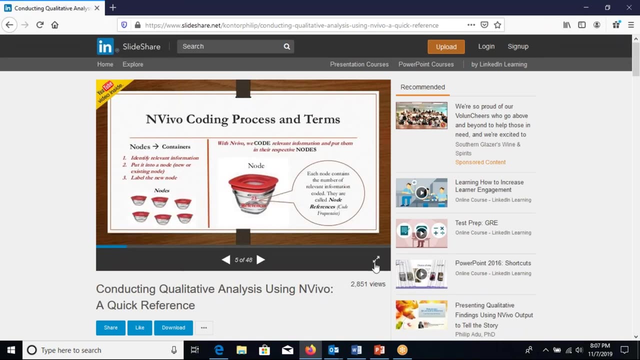 personally, i recommend in vivo uh to you and i also have a presentation that you know i try to keep up as much as i can on how to traduce and our experience itself from the traditional standpoint. so if you have any questions in vivo or, um, any other questions if you want to. 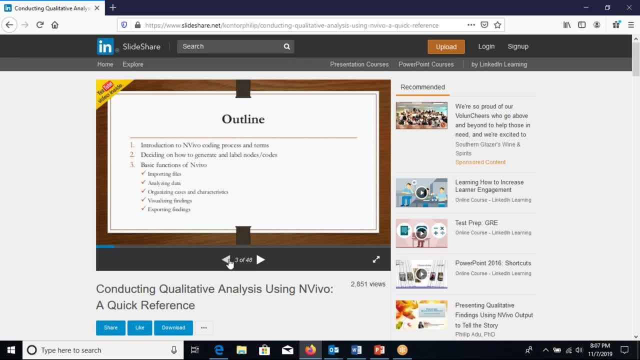 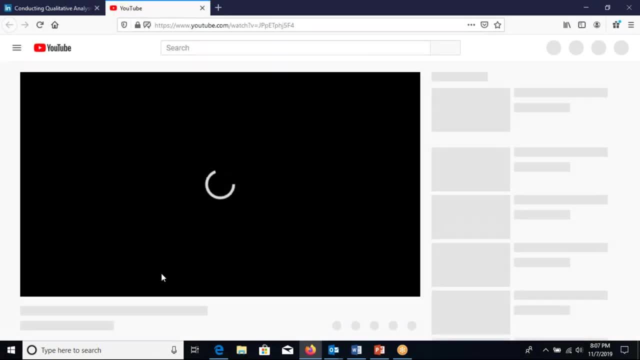 like to comment or like to share? um, feel free. um, i can't tell you know, it's, it's, uh, it's, it's still a. it's a little bit confusing, but that's okay. if you have questions and i will give you a time to answer them and we can, i can answer them at the end of the session as well, in the. 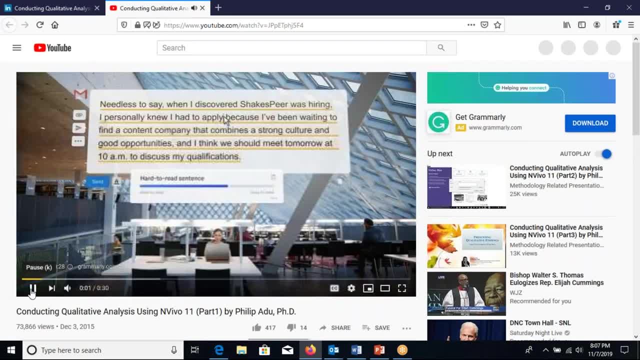 next couple of days. but you know, i um, i got a couple questions from uh from the audience, so, um, uh, yes, we got a few uh questions from the audience, so please, um, uh, if you have any questions, please feel free to leave them in the comments section, and i would like to read them out at the end of the session. 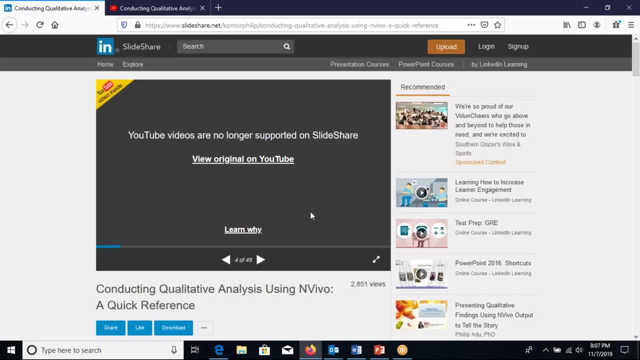 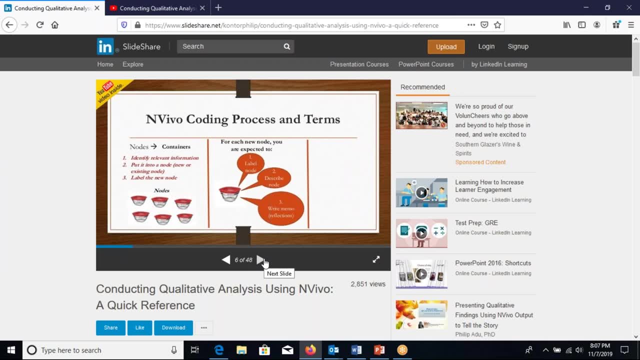 23,000. so I try to break things down for students and if you are beginner, I recommend in vivo for you, and especially if you have PC- not because most of that my presentation, I use PC, Windows- so if you have PC then I recommend in vivo for 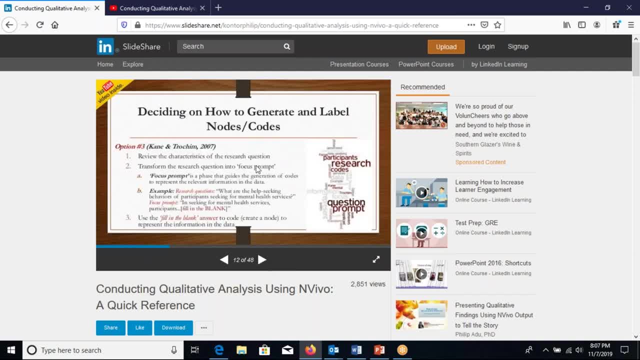 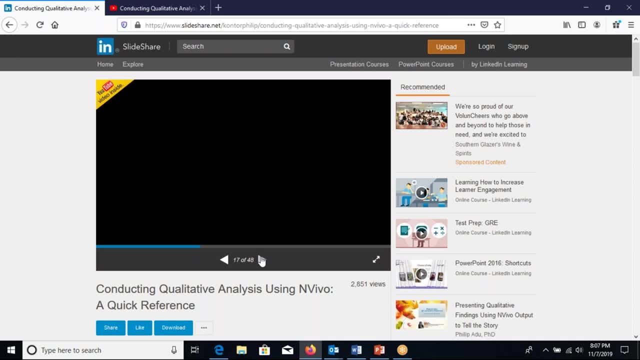 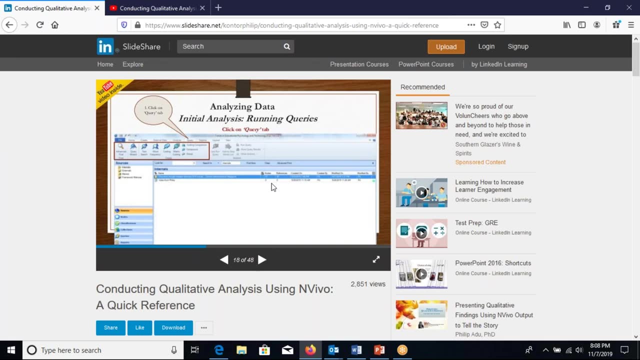 you. thank you so much, but that will be. I don't have a PC, I have a Mac, but anyway, I just, I guess is foundations, I I need to interpret that foundation of coding. you know that I can then put it to work in any software. okay, thank you, doctor. 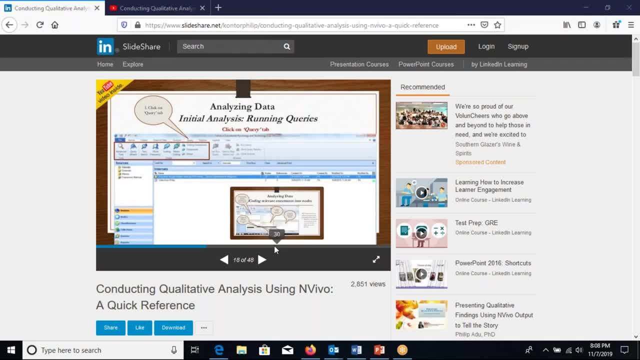 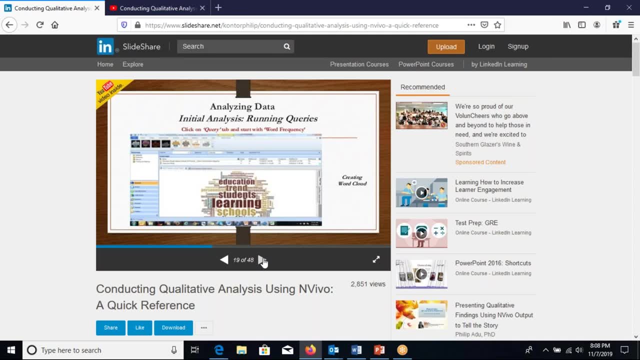 one other thing about choosing the software. that's part of reason why we have max QDA in this course, so you can get some opportunity to test it out and see how it feels, and that that might be your choice. you might say, hey, I learned to use this in class, this feels good, and this feels good and this feels good, and 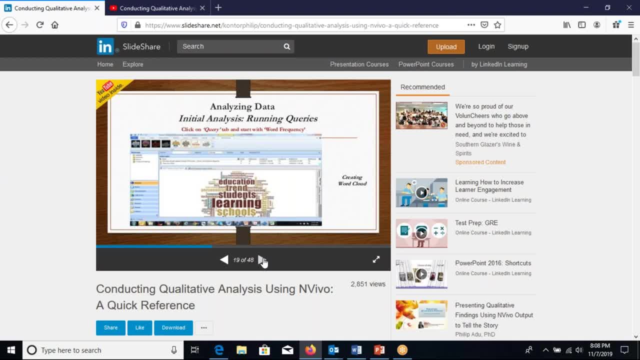 find something I can apply this to a course I've just always always done. if they do that, have some skills that maybe I need to teach some themselves, both different devenir kind of changecs and things. but really find something that you're most comfortable for me, let me move forward if need not require you. 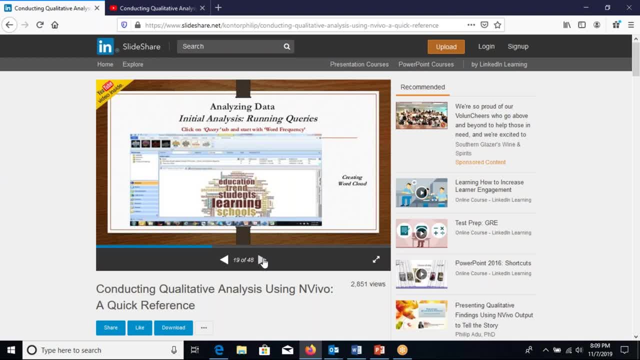 might decide- and I've done that before- say this didn't work out for me and we even have- I think John can speak to that in our class. he says: hey, I've been using one, but it's not as intuitive for me, so I'm looking for another option. is it the? 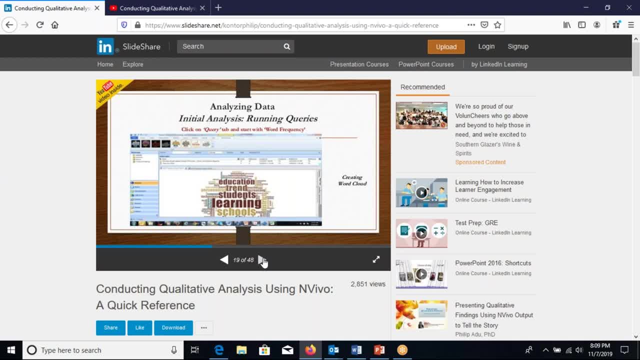 a license for the duration of the course and then, if they decide to purchase it after the course, they get- I think it's a 20% discount on the student license. if it's free, then use it, because you know for this one you have to buy it, so it's free. 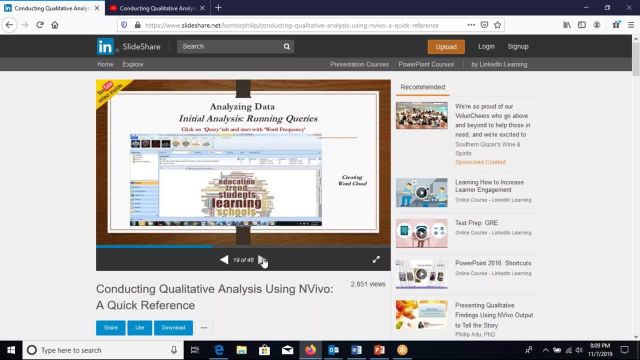 okay question: all right, going once, going twice. I know we are you minutes over our scheduled time, but i did not want to stop you to know this was going really well. so thank you again, dr adu, for all of your expertise and your wisdom, and appreciate your.